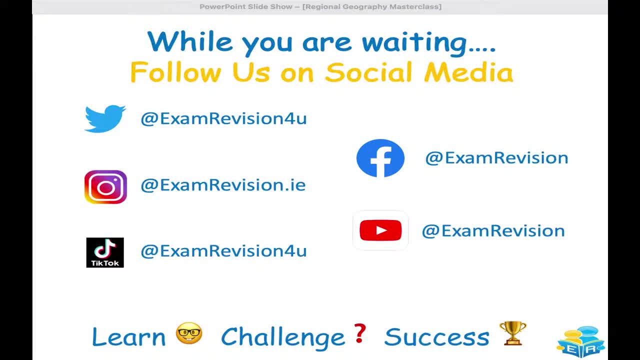 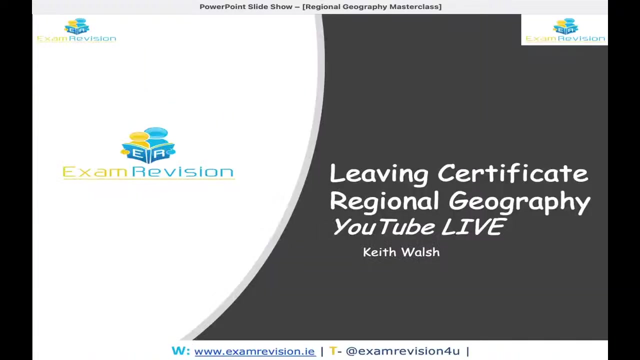 Thank you, Hi everyone, and welcome to today's Masterclass for Geography with examrevisionie. So today's session is going to be based on regional geography And Keith Walsh is my name and I'll be taking you through the next 45 minutes or so. 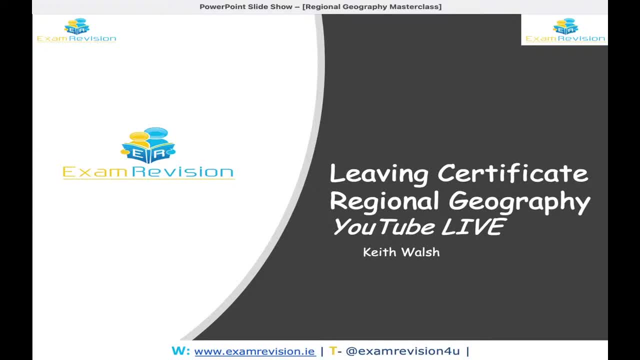 45 minutes to one hour. It's going to be like a whiz tour through regional geography, Looking at the key things that I think are going to be important for you guys that are taking the 2021 geography higher level paper, like this year. 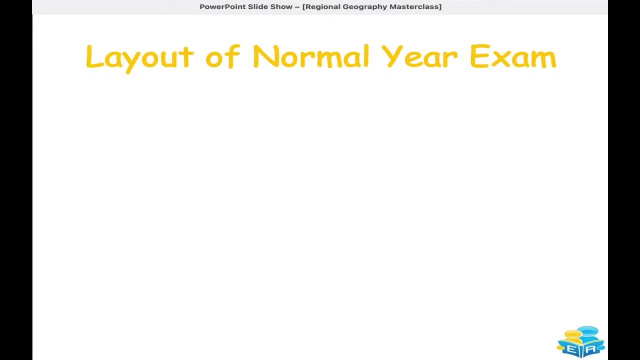 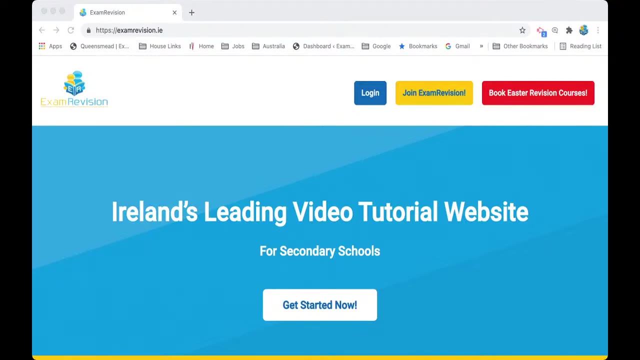 Okay so, just Before I go on to that, if I just bring you on to our website. Okay so, on our website, what we do have. we do have some Easter revision courses that are taking place And our Easter revision courses they're online. 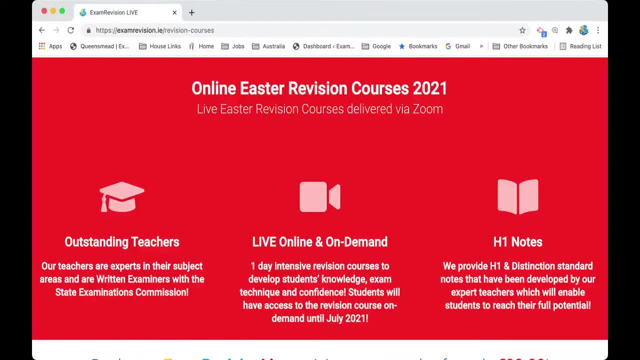 They're all being delivered by outstanding teachers. All our teachers are written examiners highly experienced And they all will be able to give key insights into how to maximise your marks for each of your subjects. All of our subjects are live and will be online. 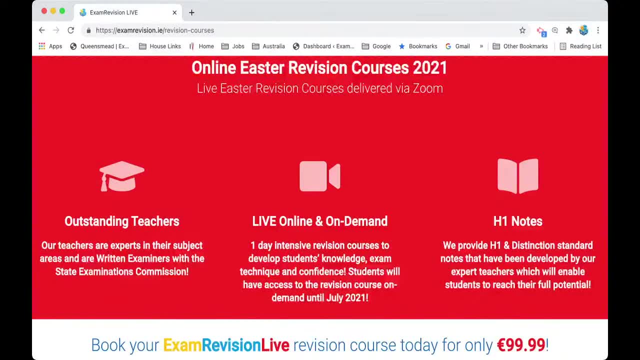 And you'll be able to watch back on demand at like 24-7, all the way up until July 2021.. And all of our notes have been produced Our H1 standard And have been produced by All our expert teachers. 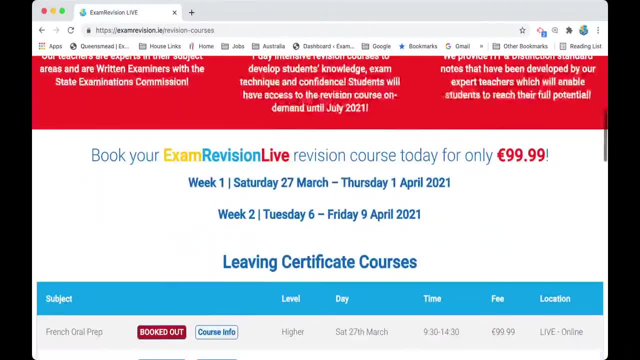 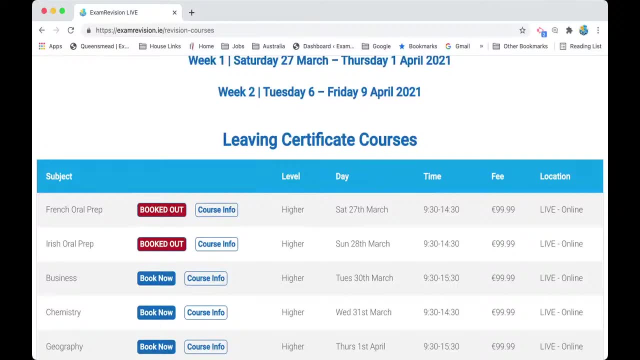 There's still time, So we just started today with the French oral. That course is booked out. Tomorrow's Irish- That course is also booked out. There are a couple of places left on the courses here that you can see. So business, chemistry, geography, maths, economics. 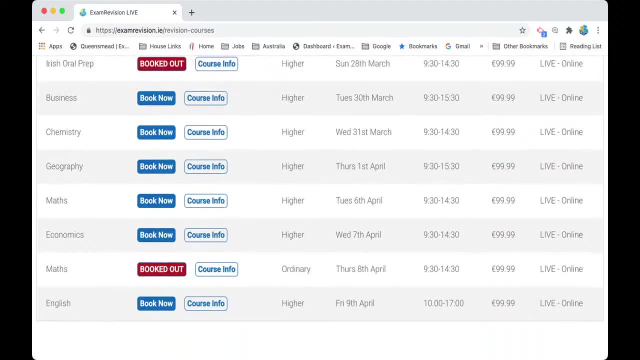 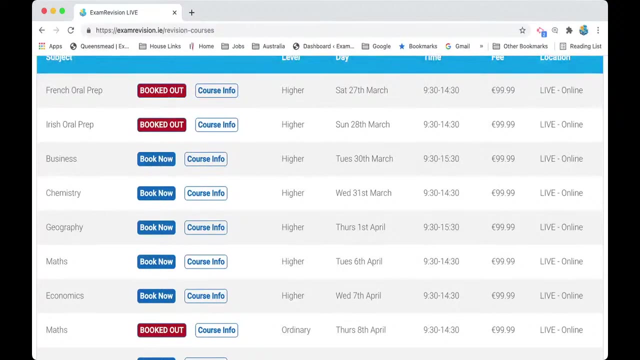 Maths ordinary level is booked out. There are some places on the higher level course And the English higher level course is also Has some places available. Okay, We are capping the classes Because we want to To make it really personalised and to allow students to get the most out of our Easter revision courses. 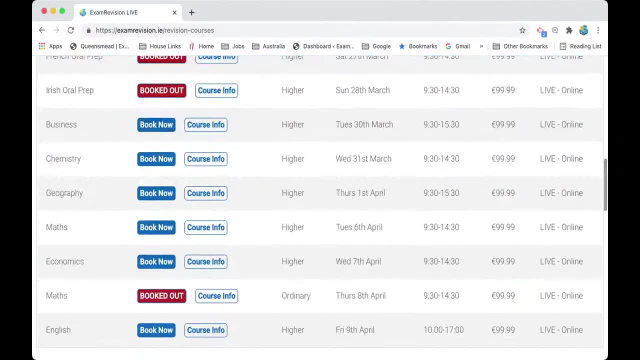 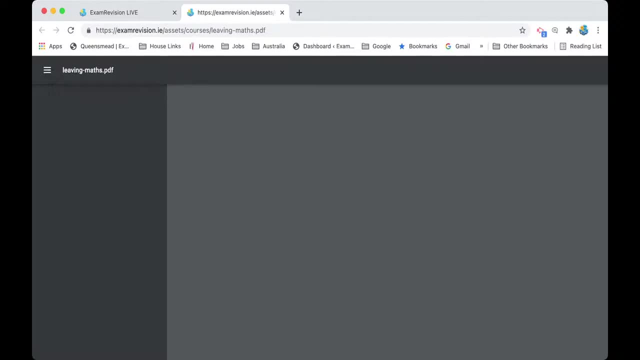 If you want to know what's going to be on the Easter revision courses, you can click on course info And when you click on course info it'll open up and you'll be able to see exactly how the revision course is going to run. 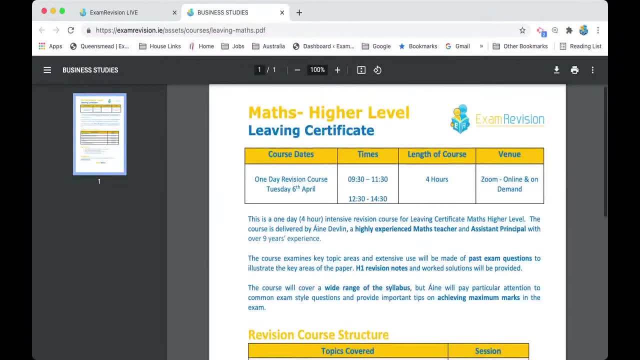 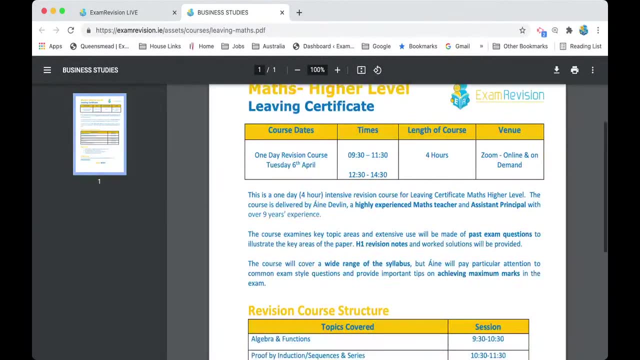 So, for example, the higher level maths course. it's a one day intensive revision course, Starts at 9.30.. Finishes at 2.30 and it's four hours long, And Áine is our maths teacher. She's a highly experienced maths teacher. 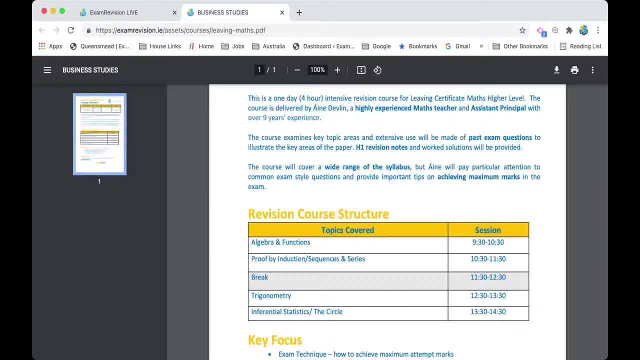 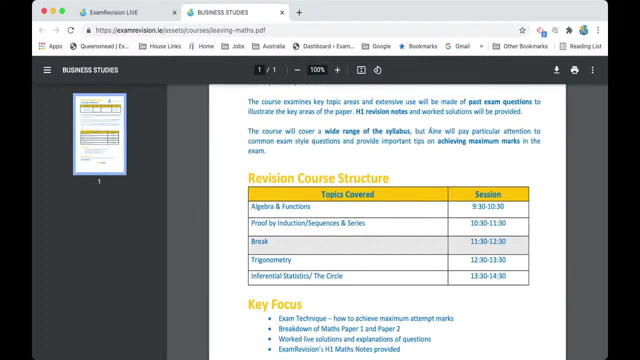 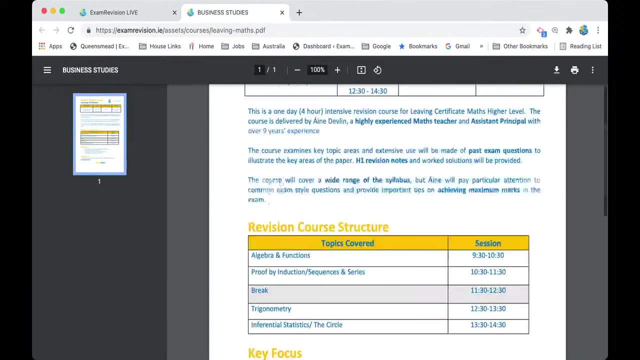 Assistant Principal. She's won awards with the Maths Association, She's a fantastic maths teacher And she'll be going through algebra functions from 9.30 to half ten and so on, So you can see exactly what is going to be covered in each of the courses. 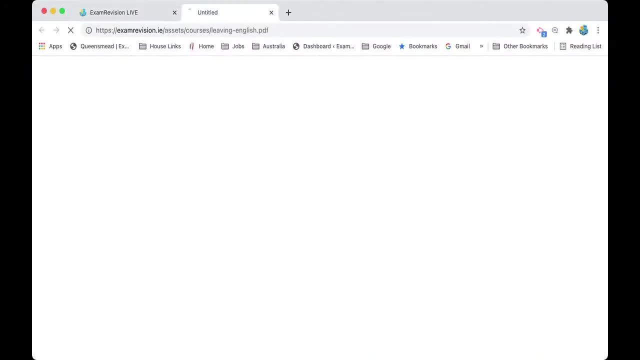 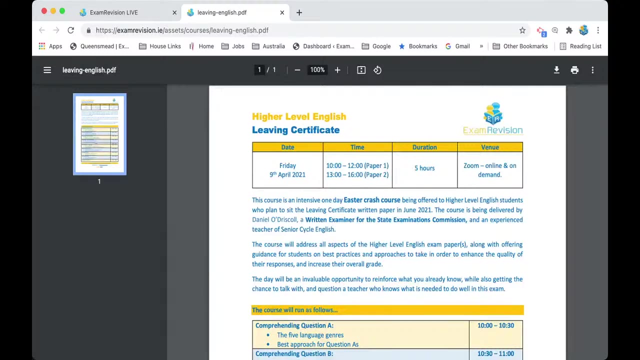 Likewise, if you click on, say, higher level English, You will get the breakdown of the day. Okay, so this one is going to be five hours. It's run from 10 to 12.. Paper one: There's a break for lunch from 12 to one. 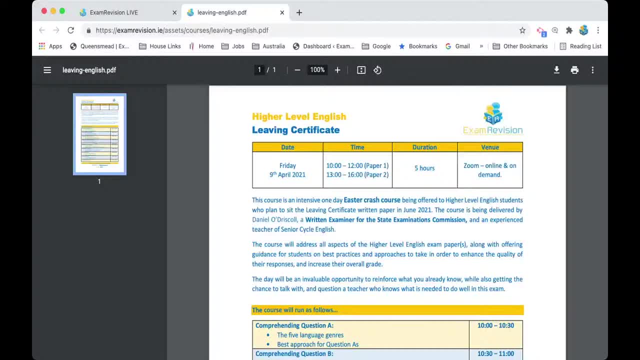 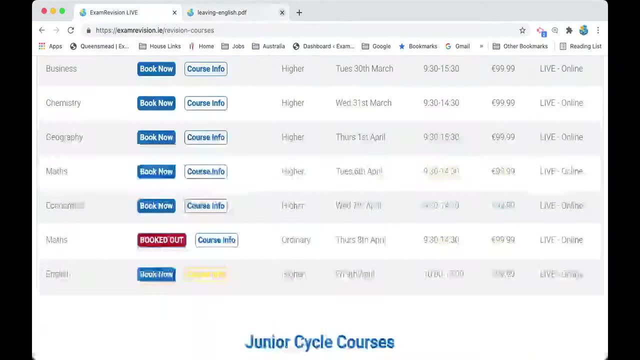 And then, from one o'clock to four o'clock, Daniel is going to be looking at paper two And you can see in detail how the course is going to be broken down. So that's there just for you guys, And the geography course is going to be delivered by myself. 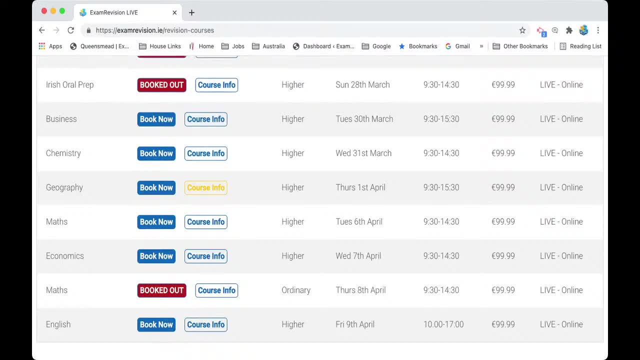 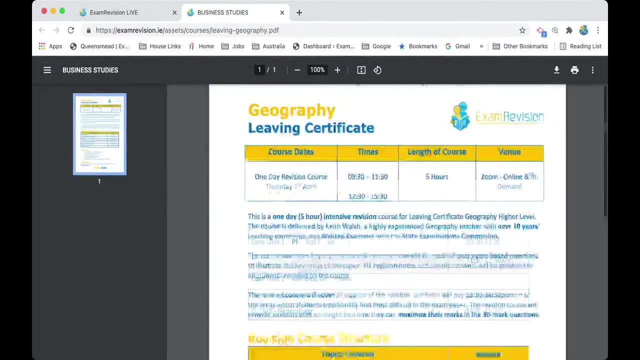 And it's going to be five hours long, And you can see the breakdown, The breakdown of the course, here. So it'll start at half nine and it'll finish at half three. So if you would like some, if you enjoy today's class, 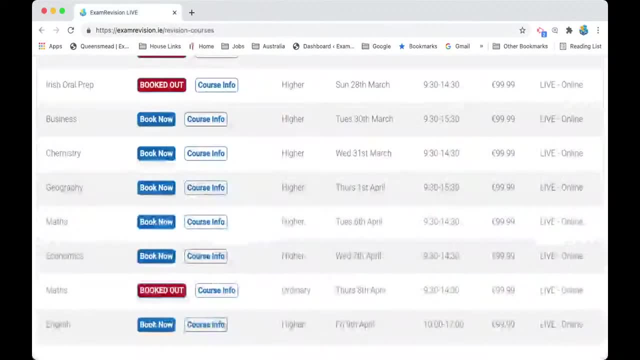 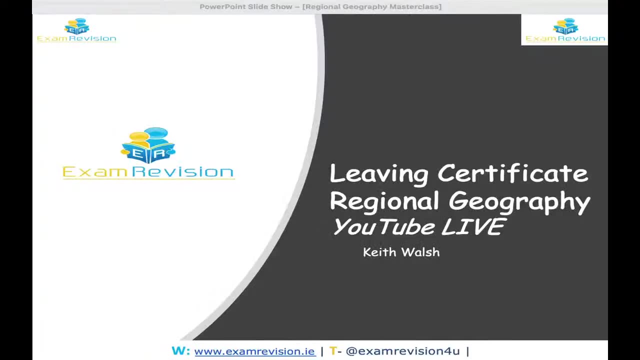 And you'd like some more. you'd like to like some more information And to look at it in a bit more detail. You can, of course, book on to our courses to get that information. Okay, so normally the normal layout of the exam. 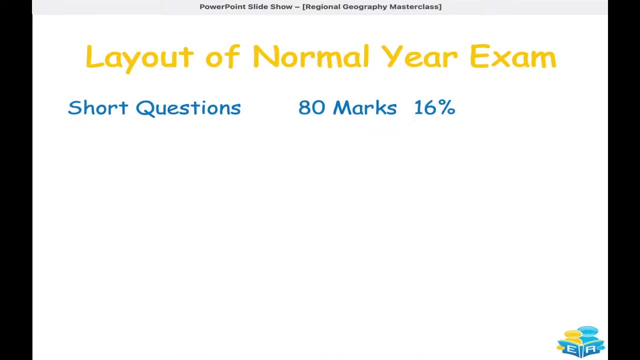 Okay, so normally it would be, the short questions would be 80 marks And it's worth 16%. physical geography will be 80 marks and it's worth 16%. regional geography We're going to look at today is 80 marks and it's worth 16%. your elective. 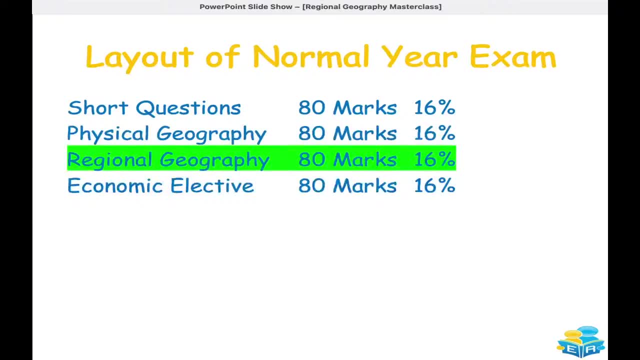 So it's whether you do your human or your economic elective. I tend to choose the economic elective, and would be 80 marks or at 16%, and your option, And again I tend to do the geoecology option, as 80 marks is worth 16%. plus you got your field study, which is 100 marks, and it's 20% overall. 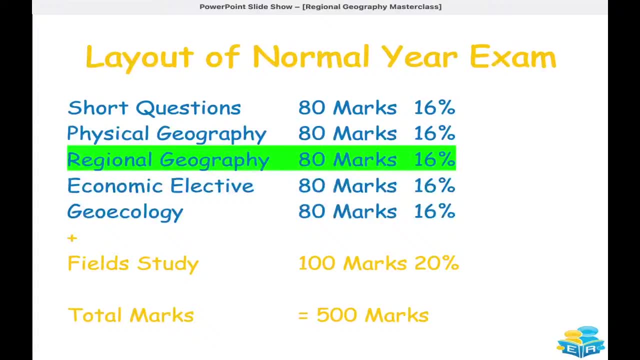 The paper is worth 80% and it feels like it's worth 20%, and this is how you would, this is how I suggest, like breaking down, like the timing. So half an hour for all the sections apart from the geoecology the option. I'll give that 40 minutes. 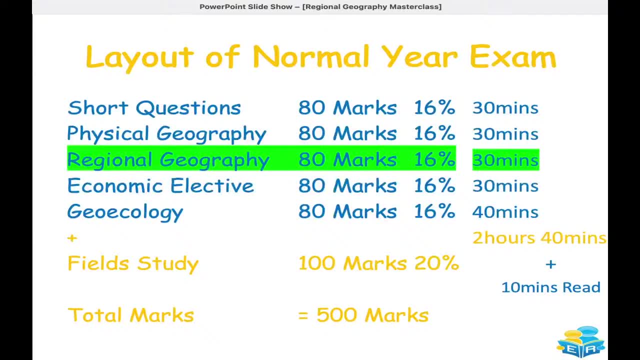 And what timings is. timing is definitely up to the, to each individual and you. you'd have to understand and learn what timings you're going to produce, Cause some students might do the short questions in 25 minutes and they'd have five minutes to put into into maybe. 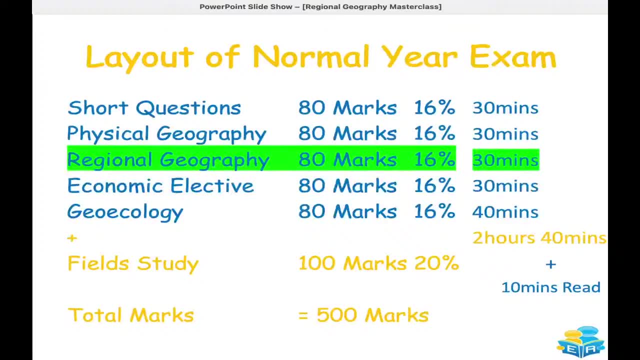 Two and a half minutes into physical geography and two and a half minutes into regional geography. So you have to. it's timing is something that you need to understand and work out, And you do that by practicing past paper exam questions and working on your exam technique. 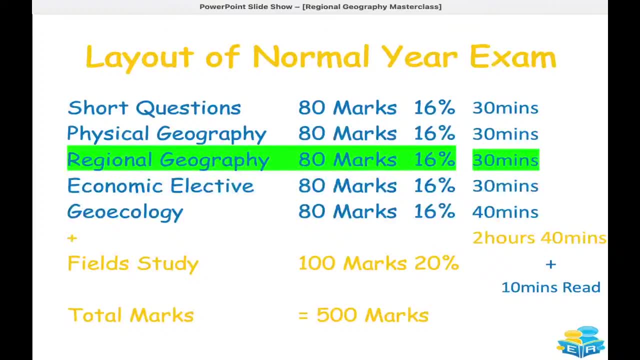 And then that would leave you 10 minutes to read the exam. However, like this year, 2021 is different. Okay, There has been adjustments, which I'm sure you've all been aware of, that just come out like this week: 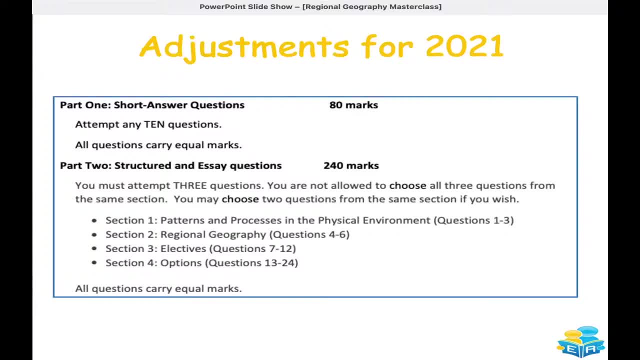 Um, and what's going to happen is there's going to be, um, a few, a few changes that you need to be aware of. Okay, Okay, Short questions. It's going to be worth 80 marks, just like normal, but it's, and you have to attempt any 10.. 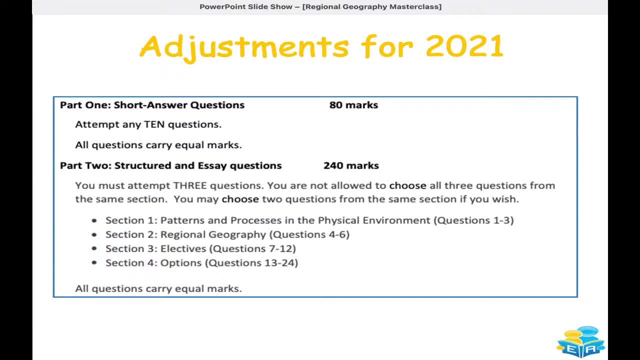 Okay, And they're all going to carry equal marks, And then we have part two. So this is like your physical, your regional, your electives and then your options. Okay, And what? like this year, what you guys have to do is, if you're sitting the paper in June 2021, you have to attempt three questions. 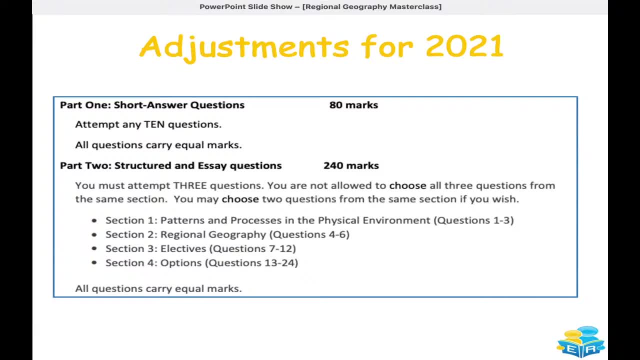 Okay, Usually you would do four and you do one from each section. So you do one physical, One regional one, uh, one elective question and one option question. this year It's very, very nice, Okay. Uh, for students sitting the paper, you have to attempt three questions and you're allowed to choose two questions from the same section. 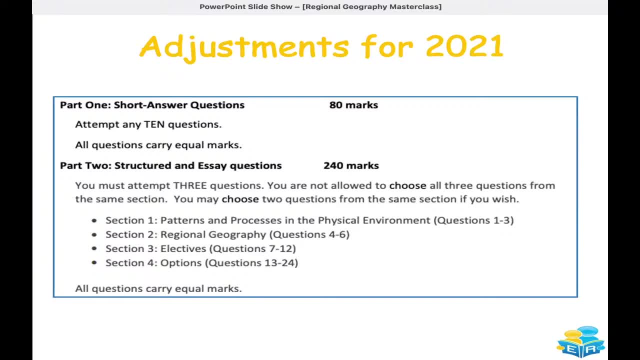 Okay, So you're actually allowed to pick two questions from the re, from regional, or two questions from physical um, or your elective or your options. So it's very, very nice, Um, that you have so much Um, that you've got so much options, uh to do. 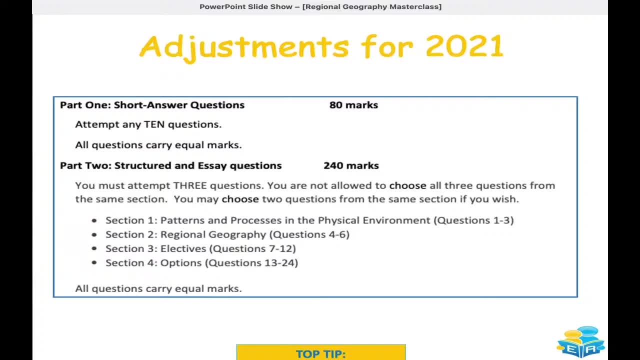 Okay, So what would be my tip? Okay, I think students should uh answer four questions, like this year, because the timing should stay the same, So you're still going to have two and a half- oh sorry, two hours, 50 minutes to to answer the higher level paper for leading search geography. 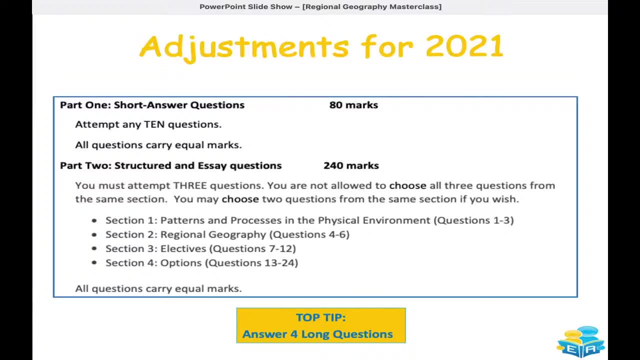 So my tip would be to to try to get to do four, because you're not going to be doing four in in any less time than usual. It's going to be the same time as always before, Um, and what will happen is the examiner will have to mark all four questions and then pick your best three. 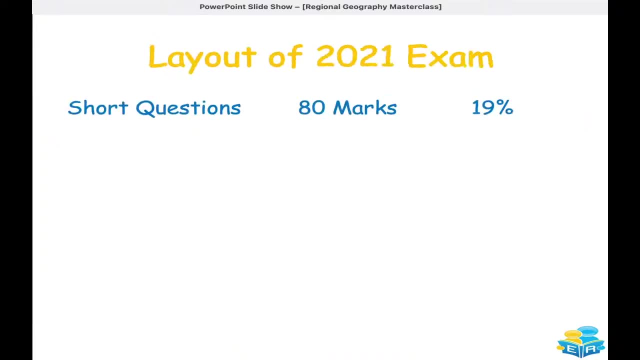 So this year, this is how the, this is how the, the, the waiting is going to go for the 2021 exam papers. So the short questions is worth 80 marks and it's going to be worth 19%. So it's going to be up from 16% to 19% this year. 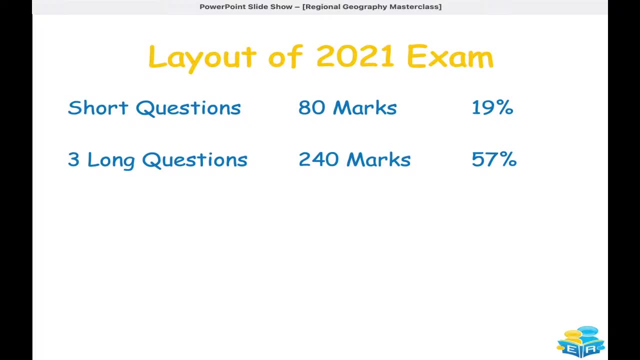 Then you've got your three long questions, which is 240 marks, 80 marks each. So 80, 80 by three, it's 240 and that's going to be 57%. Okay, Okay, Okay, Okay Okay. 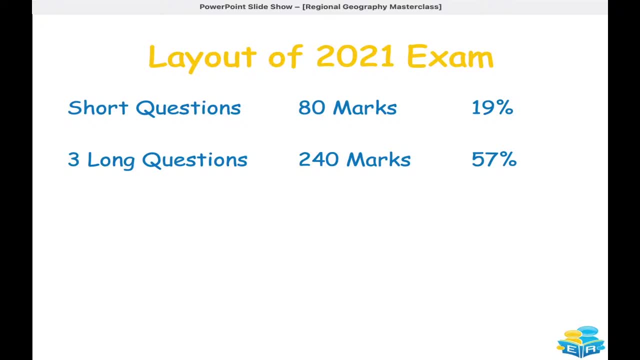 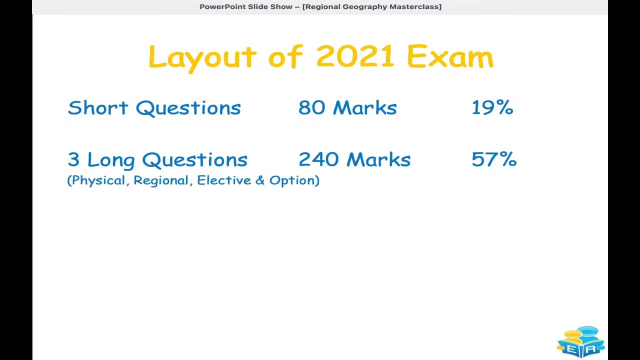 Um, and that's going to be made up. So your three long questions come from your physical, your regional, your elective or your option, And two of those are allowed to come from one of those sections. Okay, Now you can't answer three questions from, say, physical, or you can't answer three questions. 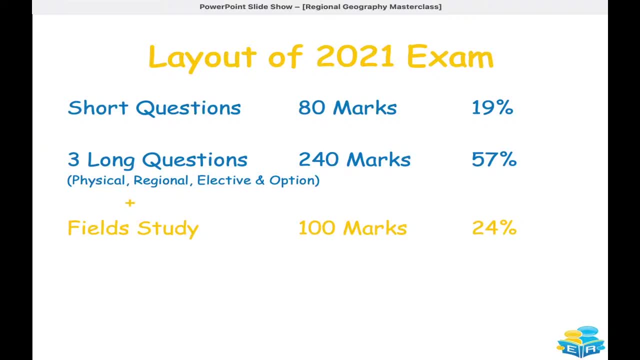 from regional, but you can answer two from physical. You can ignore regional, You can ignore You're elective and do one question from your option. Okay, So it's very, very open. It's very, very nice for students sitting the paper, uh, and then your field study. it's. 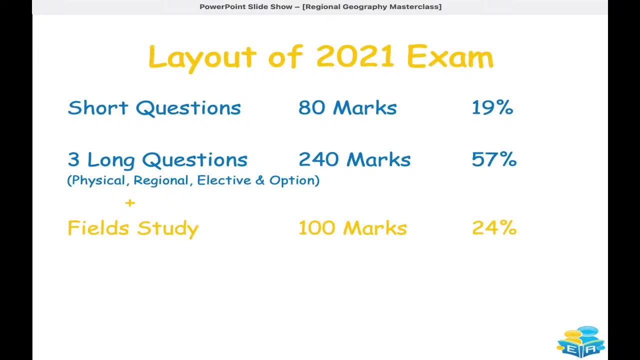 a hundred marks. Okay, So it's worth 24%. So it's up from 20% to 24%, like this year. So total paper it's usually at 500, but this year it's 420 marks. You're allowed to pick two long questions from one section. 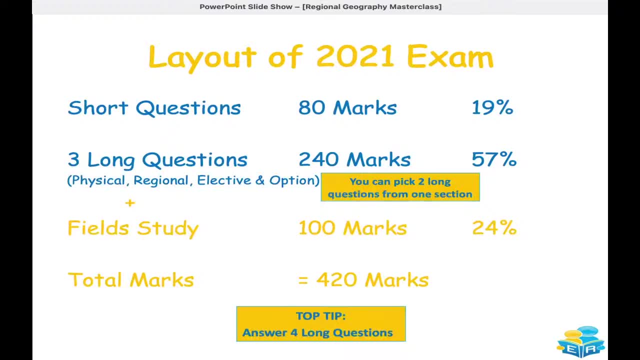 Like I've said, and top tip, I would be trying to answer four long questions. Okay, Because the timing is the same as all as before, As previous papers. So for regional geography, this is the timing that I would suggest in previous years. 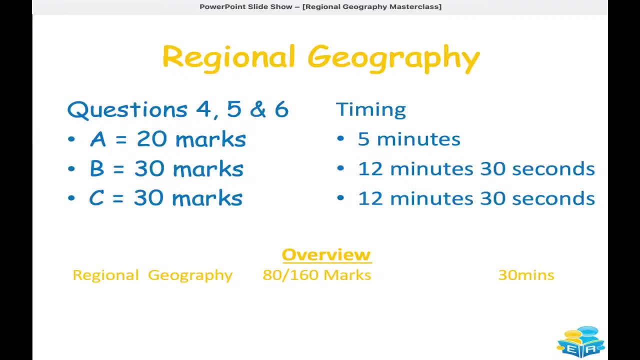 And again, even if you're setting the paper in 2021, I would suggest the same thing: 30 minutes for your for one question. So now this year, you could do two. So you could do say question four and question five from regional. 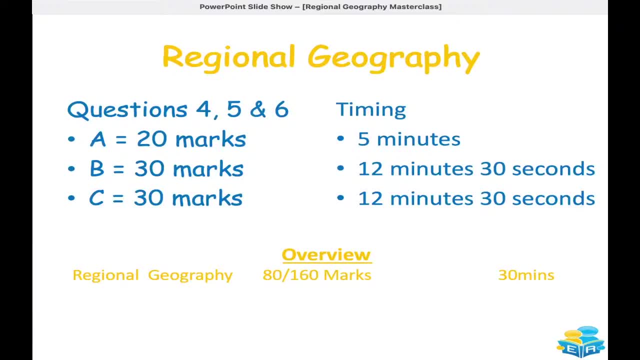 Um, and these will be the timings that I would suggest that you go with. Okay, So a: 20 marks five minutes. uh, your B and C: 30 marks each. You have 12 and a half minutes, Okay, Okay. 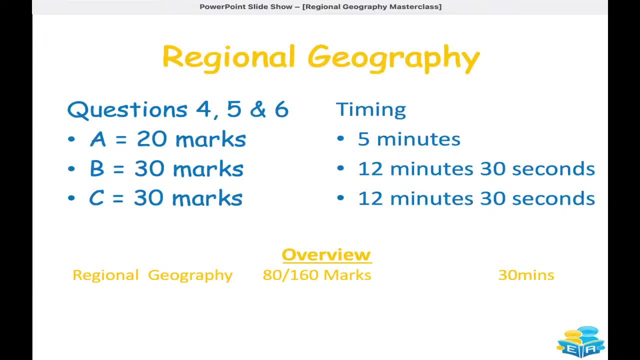 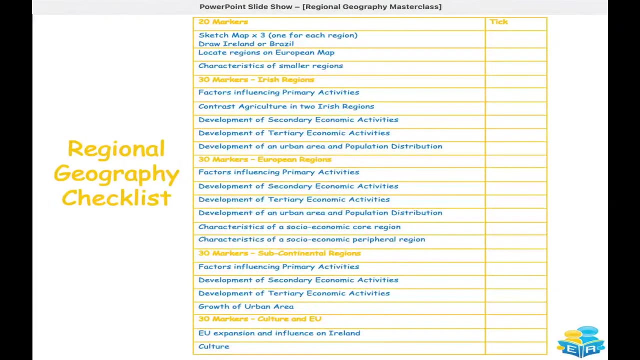 Um, to answer those questions, Okay, And I'm going to go through some long questions. some part A's the sketch maps on some long questions in today's- uh, in today's lesson, Okay. So the first thing is: this is like a regional geography checklist that I've put together. 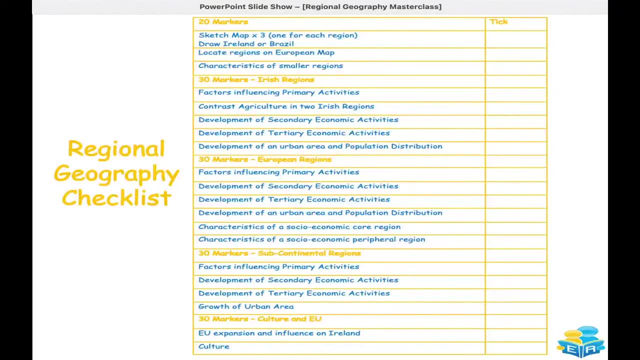 Um, and it has everything that you need to know, um, for the 20 markers, the 30 markers, for the Irish region, the European regions, subcontinental regions, and then some questions that appear, uh, frequently. Um, the paper is like culture and EU, that, um, you need to be, you need to, you need. 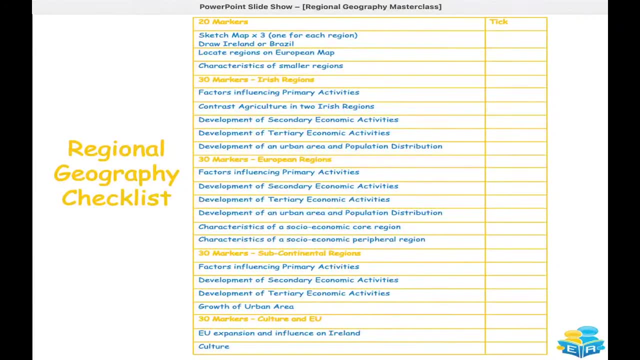 to be aware of Um, and so here's like a nice uh checklist just to break everything down, because regional geography it's very uh, it's a very big part of the of the course Um and it's one that sometimes students can feel is a challenge and it's, but it's, it's. 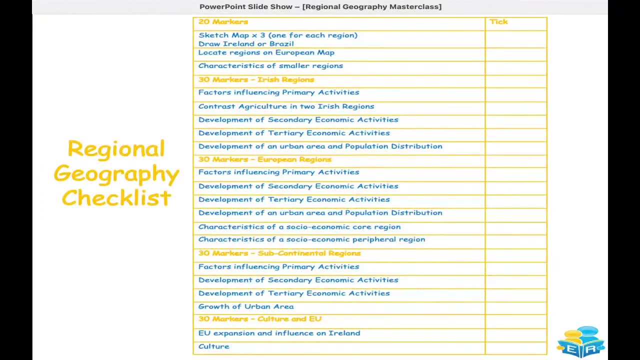 it's a very, very enjoyable part of the course because, um, a lot of this is like, particularly with Irish regions- It's where we live, Like. so it's, it's, it's a lot of the information is quite, we know quite a lot of the information. 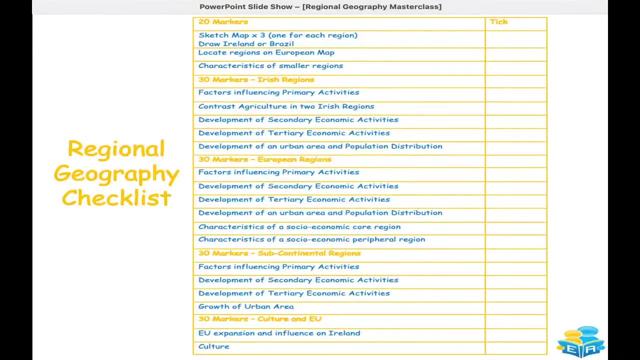 already, And then, obviously, with the, with some of the European regions and your subcontinental, you have to really like do your research and and and delve into, into those regions. Okay, So here's like our exam revisions, like essay structure sheets that we, um, I think are: 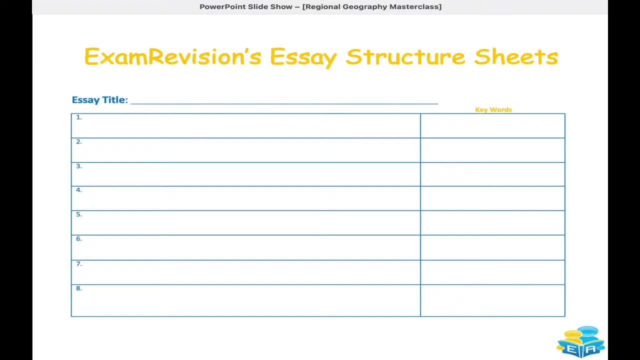 very useful, Um, and students can get these. So if you want the notes- um, I haven't mentioned this, sorry- if you want the notes, just fill out the the Google Uh form. Um, so the Google form is in it's in the description. 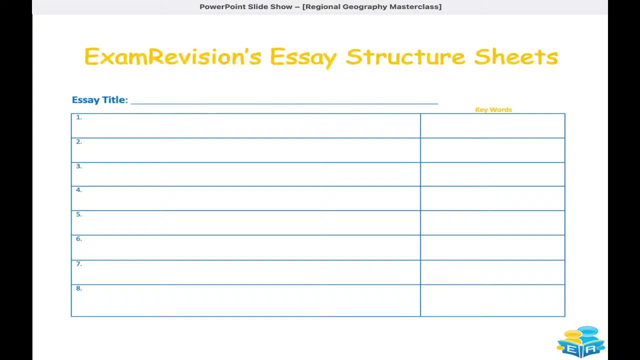 And so if you want any, if you want these notes, I can send them out. I will send them out, like we always do. Um just be aware sometimes that goes into the junk or your spam, your emails, And so if you save um exam uh office at examrevisionie as a contact, it will go straight. 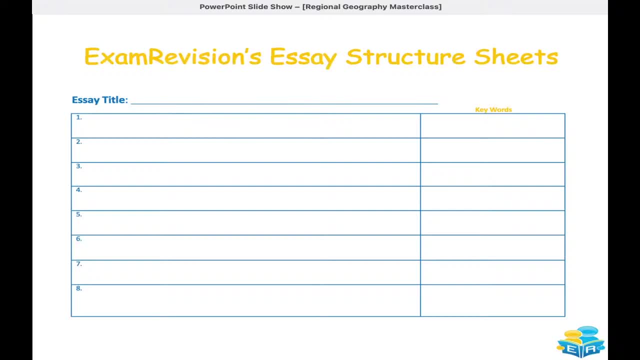 into your inbox, Um, but when we send them out, we usually send them out within a day or two. please do just check your spam, Your junk And, if you have Gmail, just check your promotions, because sometimes it goes in there. 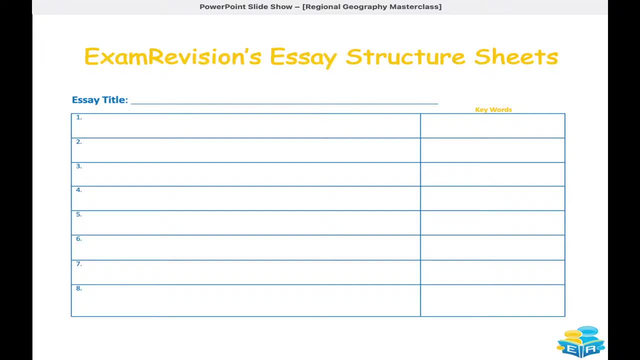 Um. so this is like the, the essay structure that we use um for, about for all our different sections, So for the long questions, so for physical or regional, your elective and then your, and then the options is different, but we still have. we have a different uh essay. 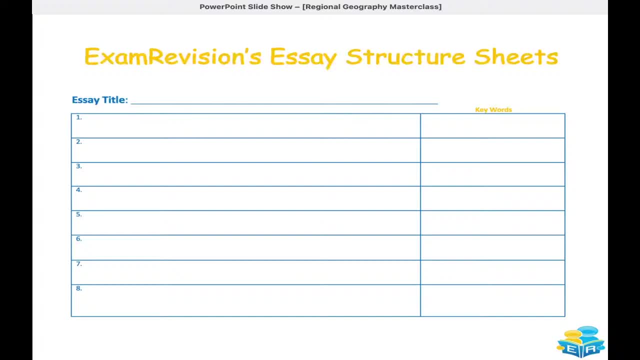 like structure sheet, which is similar but it's just a little bit different. Um, and I will go through that. if you're on the Easter revision course or under a Saturday session, that we'll be putting on. Okay, We'll be putting that on for um, for the option in the next coming weeks. 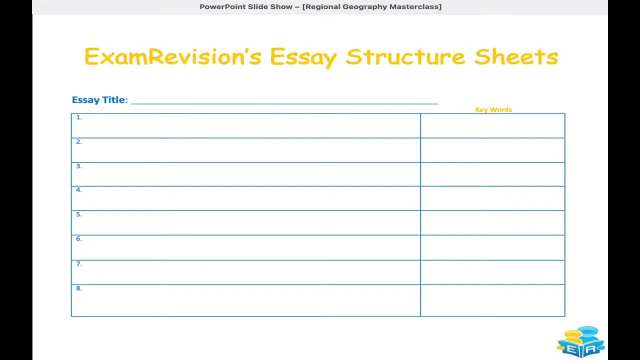 Okay, So your title is your title, obviously, and whatever the question is asking, and then you're going to have, um, your eight SRPs here, Um, what I like to do here is put your keyword Okay, And what the keywords do here is it's just, it summarizes, like, your SRP. 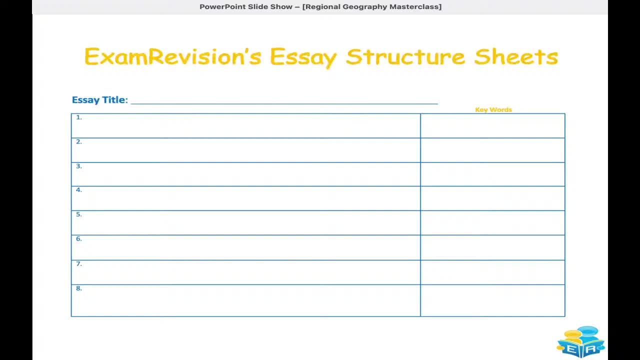 So your entire SRP just in kind of one or two words, and it can just make it make it much easier for you to be able to learn um, to be able to learn Um like like what's um, like like like what, like what you need, because when you 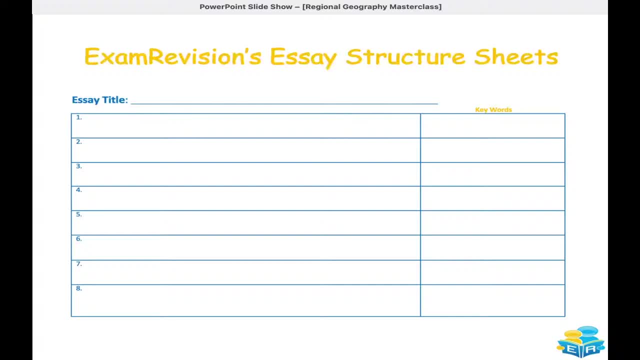 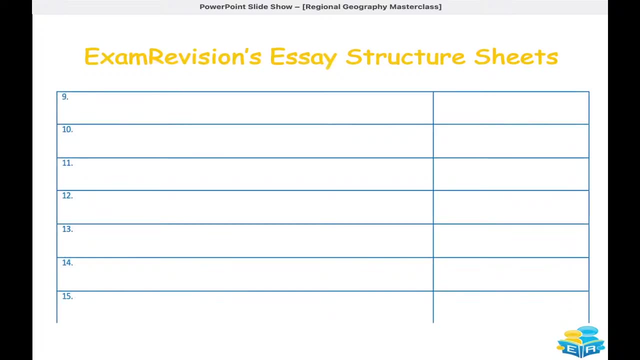 have got the whole, um, you've got the whole, like uh, SRP, it can be a lot of information, So it just summarizes everything, uh, really nicely Okay. So here's the, and then here's like from nine to 15, that's your, your, so that'd be your. 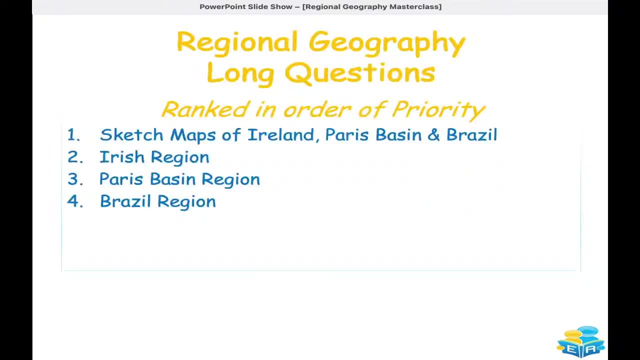 15 SRPs for your 30 marks. So ranked in order of priority. Okay, This is a priority that I've put together. This is not the knowledge. I'm not like the if anything of all knowledge for, and like no, exactly this, but I'm putting 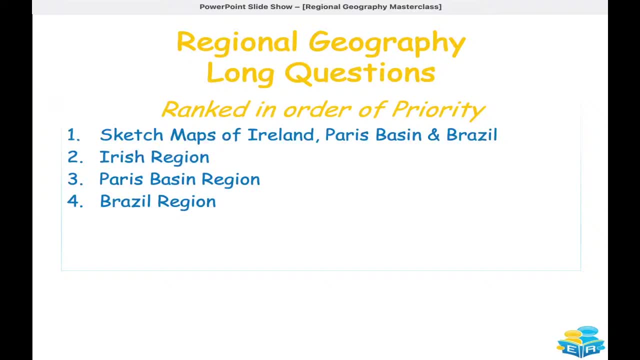 I'm trying to make it. I'm thinking, if I was a student, I'm sitting in your, in your shoes. what do I need to know? um to help me, um to help me like, maximize, um like my marks. 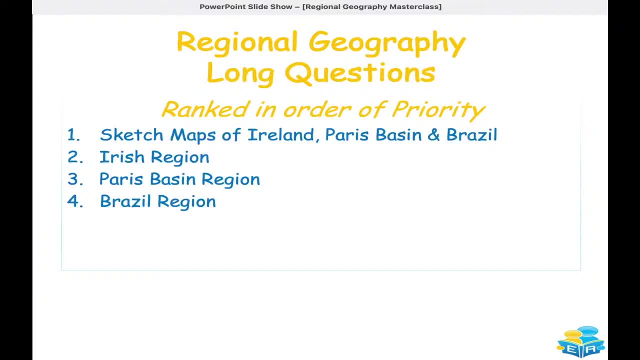 I've got a limited time. now. we're coming into- it's- the end of March, coming into April, we've got May, and then I'm going to be sitting in the exam in June. How can I Um, How can I um, like, maximize my marks? how can I focus my study? 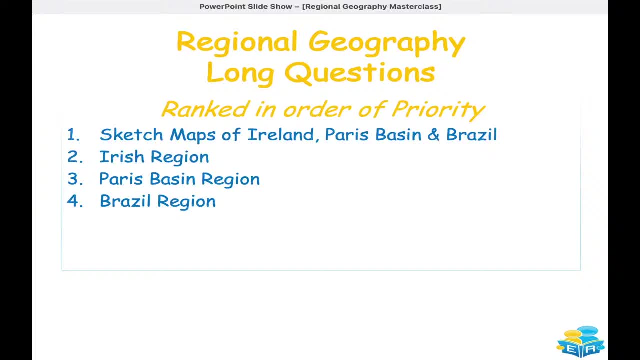 And this is what we're going to be looking at. Okay, So sketch maps of Ireland, Paris and Brazil. we're going to be looking at the Irish regions and we're going to be looking at Paris basin region and we're going to be looking at subcontinent. 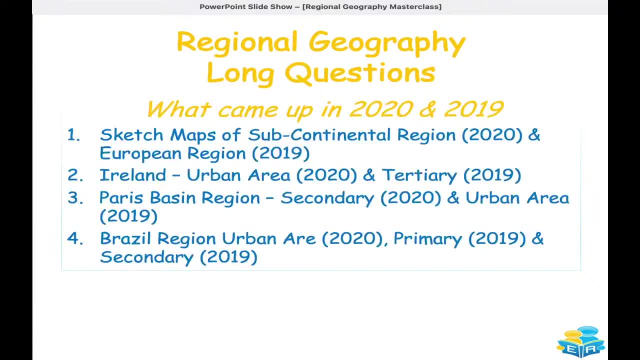 region of Brazil. Okay, So what come up in 2020 and 2019, it's always important to look at like trends to see what has come up in previous years. So the sketch map that you're asked to: you'll always be asked to draw one sketch map. 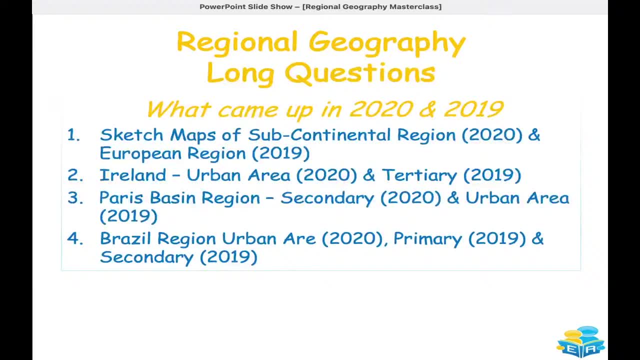 Um for a part day. for the regional geography and what came up in 2020, 2019 was you're asked to draw the subcontinental region for 2020 and the European region for 2019.. Chances are 2021, you'll be asked to draw Ireland. 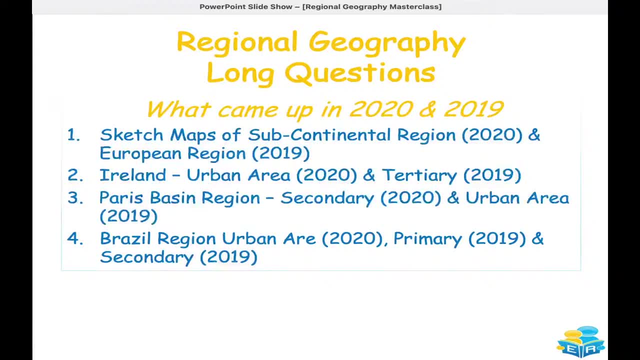 Okay, Um, but you still need to be able to practice drawing all your regions because you can use that as your diagram for the long questions. Um, in our for Ireland, uh, for the Irish for Ireland, the regions of Ireland, uh, what? 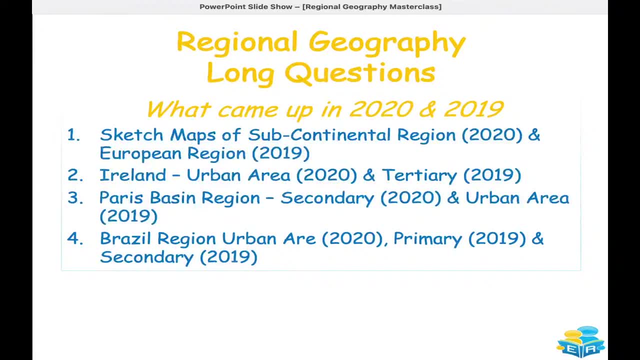 came up was the urban area 2020 and tertiary economic activities. Okay, And 2019. Paris basin, secondary economic activities in 2020 and the uh, an urban area, in 2019.. And then for the Brazil region, it was an urban area. 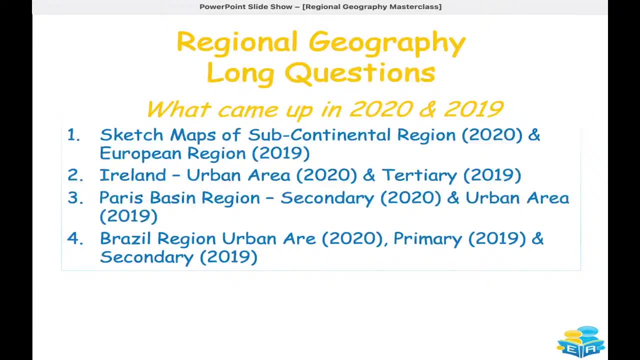 So it's typo there: It should be an A for 2020 and then primary and secondary come up in 2019 for the subcontinental region. Okay, Some people might do India, some continent regions, Some people might do America. Uh, it depends on on on the region that that you've, you've decided the reason, the 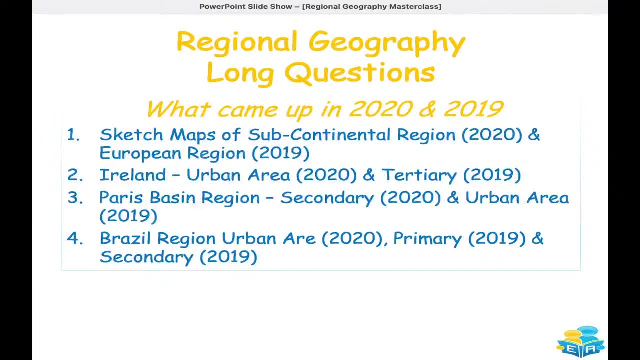 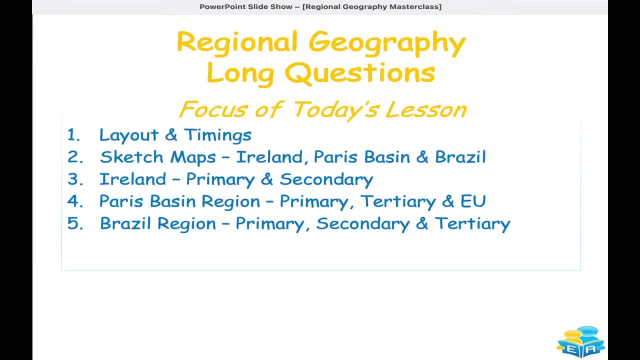 region that I like to do is, uh, Brazil, So focus of today's lesson. So we've already looked at, like, the layout and timings, and we've had a look at the adjustments for 2021.. Um, and I've also showed you then how the paper is normally as well. 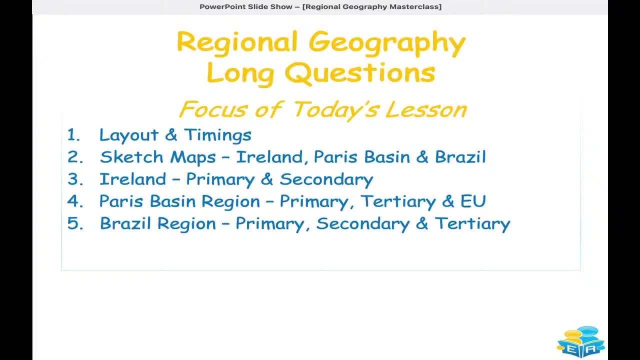 So if you're a student that's sitting in the paper in 2022, where you sit in the paper in 2023, that's more than likely how it's going to be. Um, it's gonna. it would be, uh, like the normal layout and the there there probably. 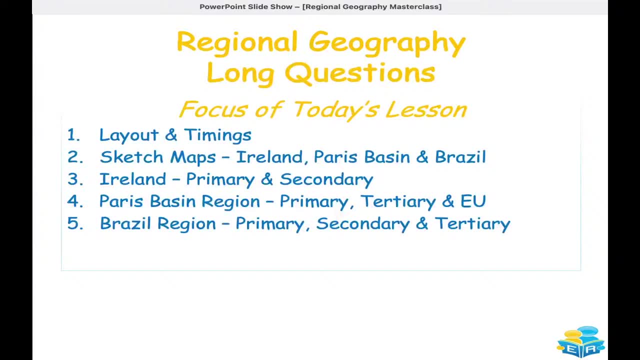 might be some adjustments for some students sitting who's in 50 and I was sitting the paper in 2022, but we learn more about that at a later date And then we'll Focus on that. Like then we're going to look at like sketch maps. 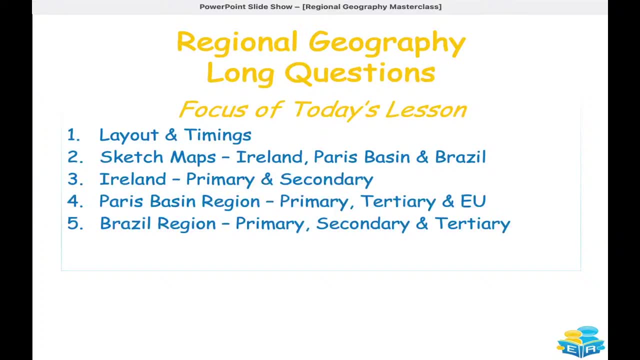 So we're gonna look at Ireland, Paris basin in Brazil, We're going to look for Ireland, Um, we're going to look at primary activities and secondary economic activities and for Paris basin, we're going to look at primary tertiary in the EU and for Brazil region. 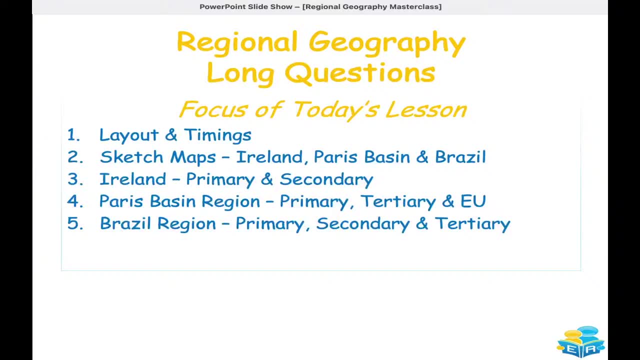 we're going to focus on primary, secondary and tertiary. So these regions are, these are the. these are the areas that I think are the- uh like the big priority for students If you're sitting sitting the paper for 2021. 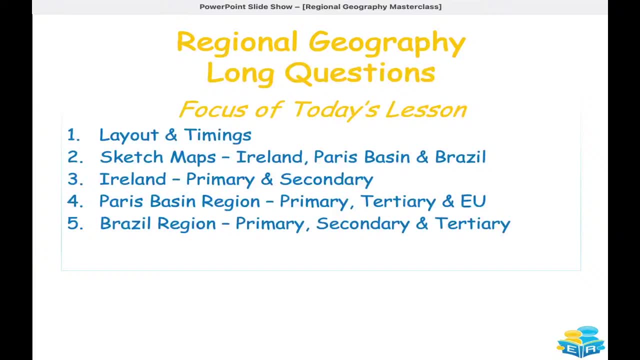 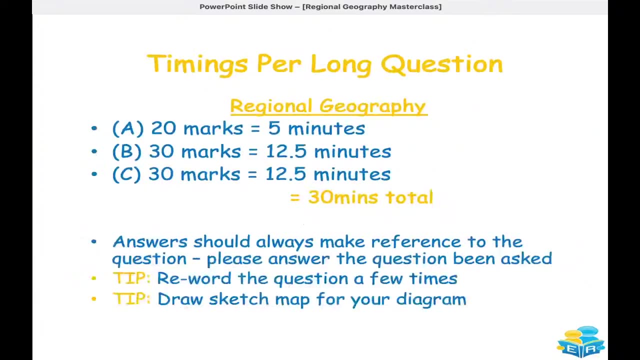 So I'm I'm trying to break it down for you, to give you, like a real focus on what you need, what you should and what maybe is more likely to appear on the paper. and for you guys, Okay, The regional, um, the timing. 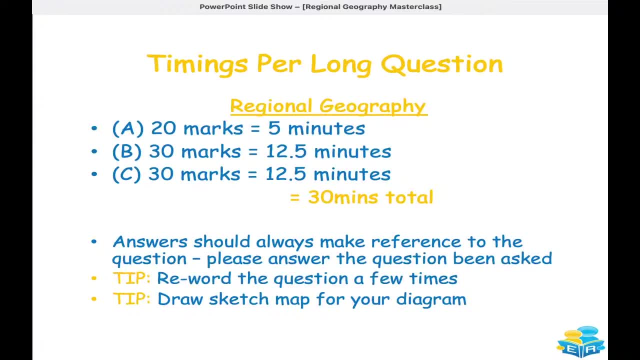 Okay So, if I've touched on this already, but 20 per day, 20 marks, I would suggest five minutes. Your B and C, it's 30 marks, 12 and a half minutes. Okay So, um, with the, with, with the, with the timing. 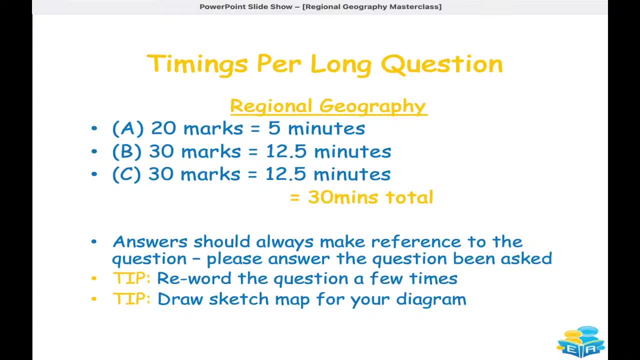 Okay, It's going to be. um, it's going to be something that you have to learn. You'll have to to adjust and to understand, like the like, your own timing, because everyone is a little bit different. So it it, it is going to be something that you have to, and the only way you learn is 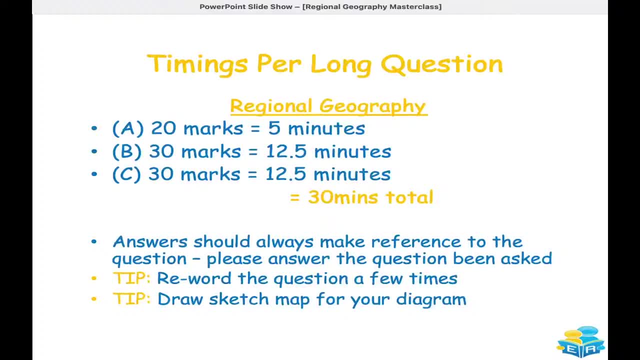 by practicing short questions, Um so, um. a little tip for you, um, with the long questions, though, is to reword the questions like the question a number of times. Try your answer, because sometimes, um students, they, they can go off on a tangent and don't. 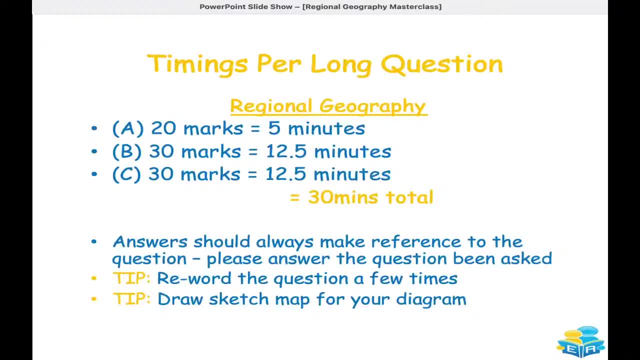 ask the question. That's that that they've been asked, and a way to like kind of keep yourself focused is to reword the question a couple of times. Also, for your diagram, draw the sketch map of the region that you're talking about. 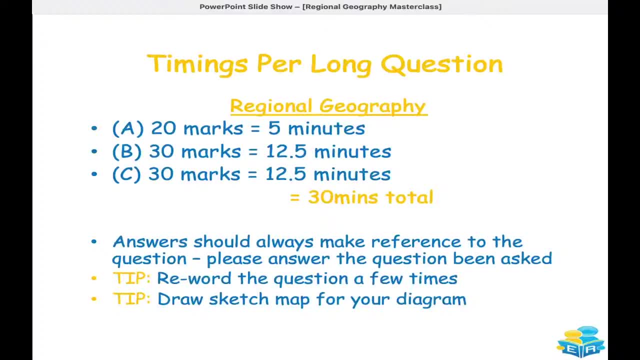 So if you're talking about Ireland and you're looking at the, the GDA, the rest of the Western region, you're looking at the Paris basin, or you're looking at the message, you know, draw you, So you, you will have practice like drawing these regions. 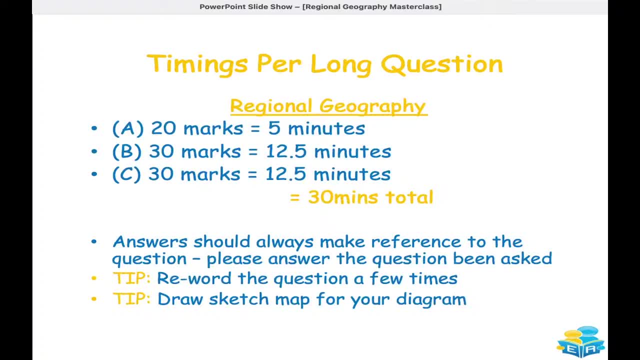 So, whatever region you're talking about, draw that as your sketch map for your diagram. So draw the sketch map for your diagram and it'll get you at least one SRP as long as you annotate it. and you can pick up, uh, more SRPs depending on how well you annotate the. 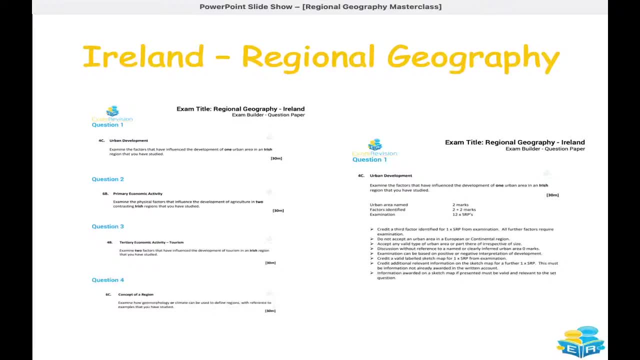 diagram: Okay, So these are just come from um the website. Okay, So from exam vision. um, we've got, like the past papers like all broken broken down. So this is, this is a thing that like. 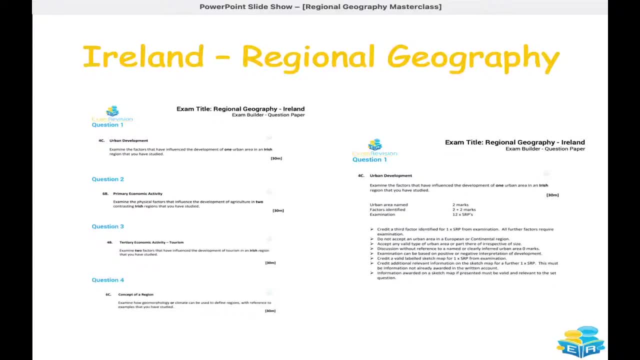 It's important for you to do go on to uh the past papers and break them down to what like, what comes up like like every year, and what comes up. um, you need to understand like what comes up. like what come up last year, what come up the year before, how frequently. 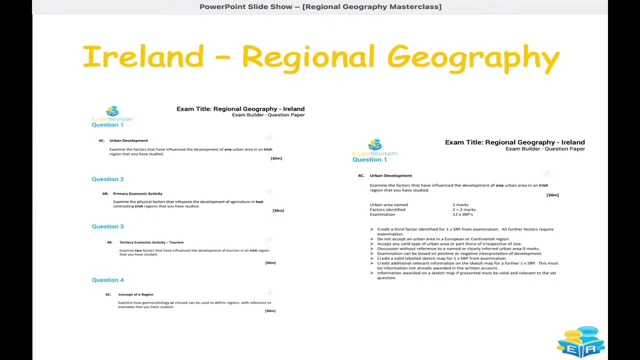 do the questions be asked, and a really good way to do that is just go on to exam revision and you can use the, the exam, uh, the, the past paper, uh, topic, uh. that breaks it down into each, into each specific like topic. 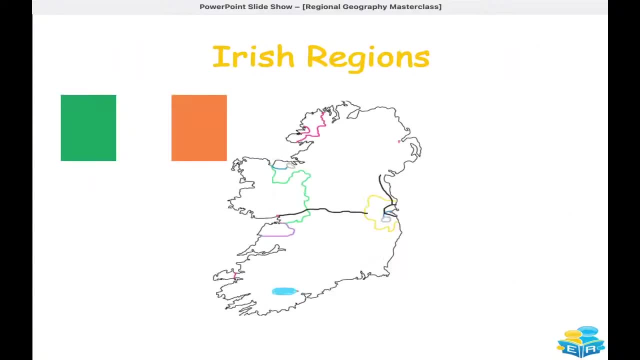 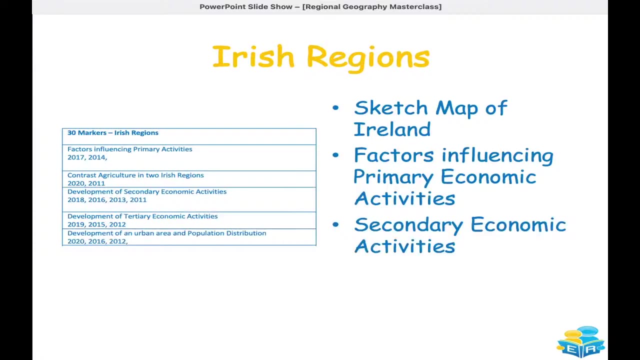 Okay, So Ireland. Okay, So Irish region. This is the first time we're going to look at and the what we're. the focus that we're going to look at for today is um sketch map of Ireland. Okay. 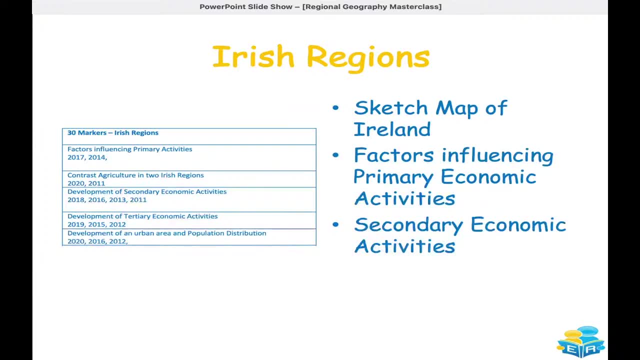 So I'm going to look at draw on Ireland, We're going to look at like factors influencing primary economic activities and we're going to look at secondary economic activities. Okay. So um, with the, with the, with the sketch map, okay. 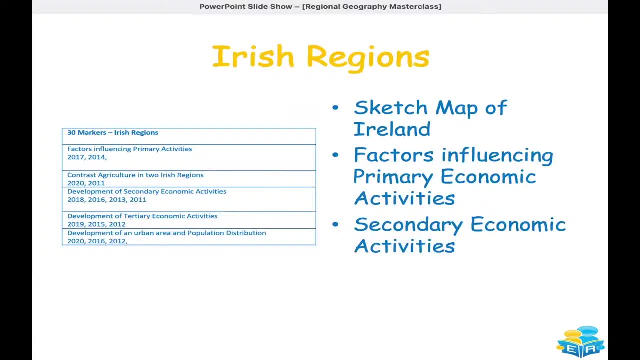 It's just, it's it's practice. Okay, It's um, it's Muslim memory. So you need to practice doing this. You can't just go into on the day and just try draw the Paris basin or try to draw um. 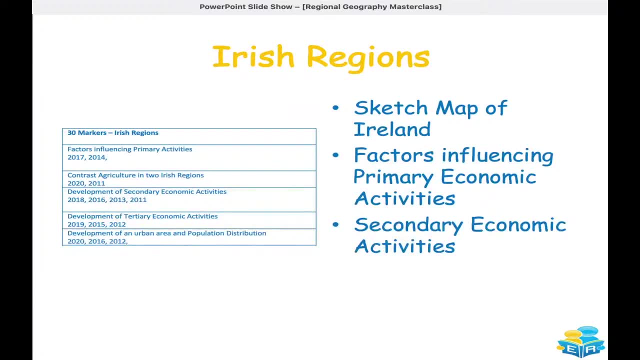 this up: your subcontinent region, if it's Brazil or India, whatever, it might be like what I haven't practiced, You need to practice. Okay, It's really easy. marks for students and factors influencing primary economic activities. Why have I chosen that one? 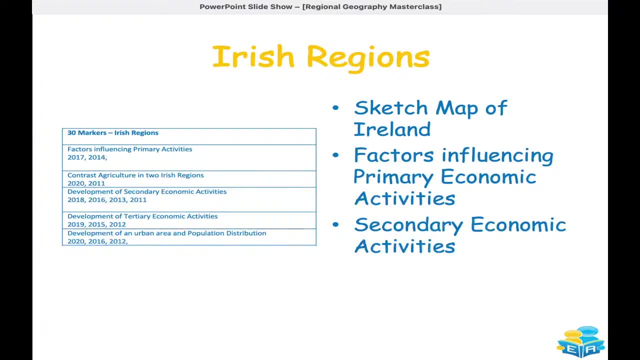 Well, if you look at like this is the breakdown of the of the past um of the questions, using the exam revision like a checklist And then having a look at that like when have these questions like appeared on in the? 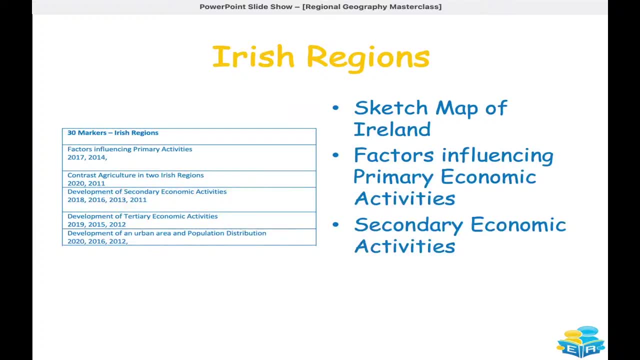 paper. Okay, So you can see primary economic activities. The last time it appeared was 2017.. Okay, So it didn't appear in 2018.. Didn't appear in 2019.. Didn't appear in 2020.. There's a good chance that in 2021, uh factors influencing primary economic activities or 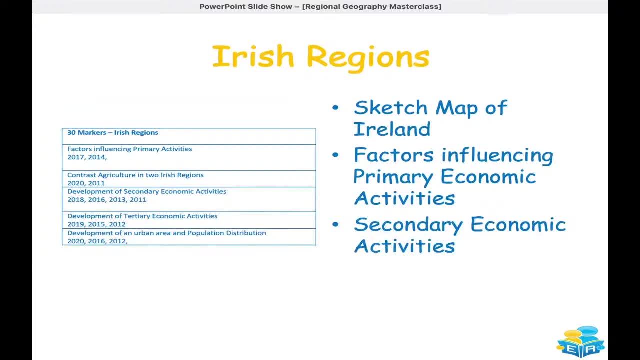 primary economic activities will appear on the paper. be prepared for that one. Um so contrasting our culture into Irish regions that come up in 2020 and 20, uh uh, 2011.. Okay, Secondary economic activities come up in 2018,, 2016,, 2013,, 20, 2011.. 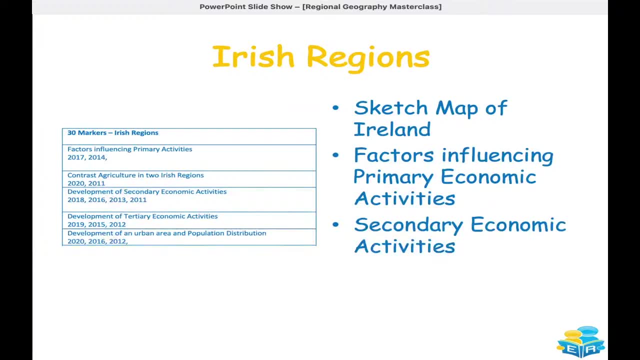 Okay, Good chance that this might appear this year in the 2021 paper. Uh, development of tertiary economic activities: that come up in 2019,, 2015 and 2012.. And then development of the urban area and population distribution was 2020, 2016, 2012.. 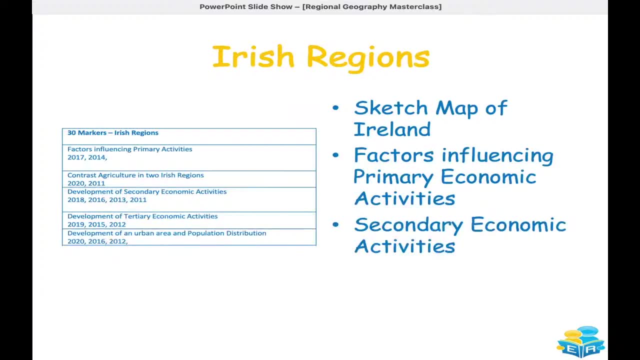 So that's why I've decided that like a focus for you guys sitting the paper in 2021 or sitting in 2022. Depending on how What comes up in 2021 should be um factors influencing primary economic activities and secondary economic activities. 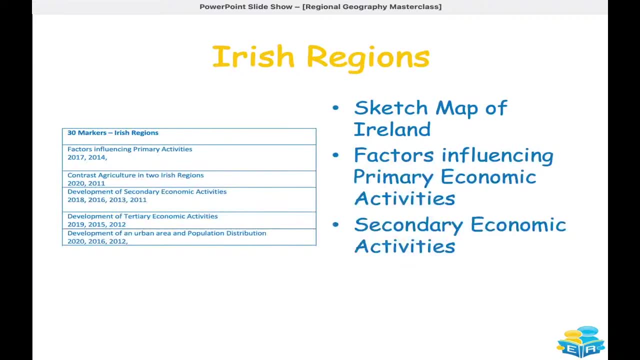 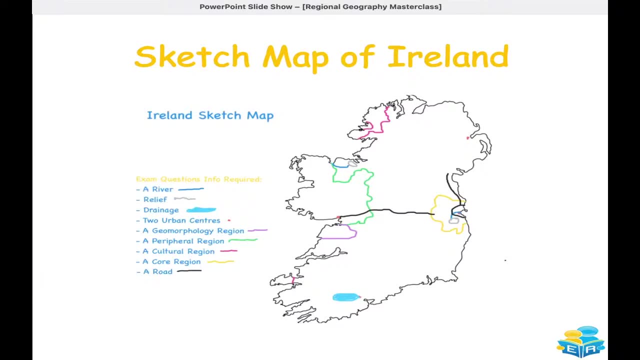 Um, so the very first thing we're gonna look at is sketch map of Ireland. Okay, So I went back and looked at like for the last 15 years, all the different things that you've been asked when you've been asked to draw a sketch map of Ireland. uh, all the. 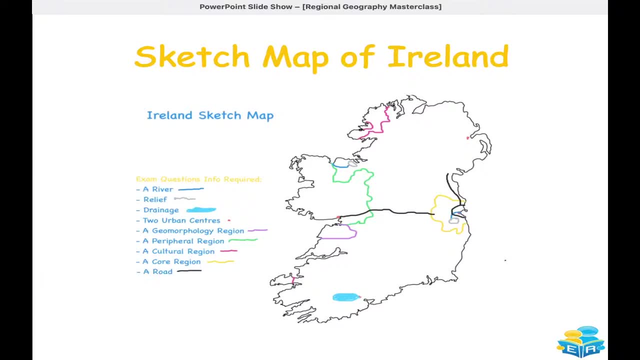 different things that you could potentially be asked. Okay, So an area uh, so a river, an area of relief? it's a drainage uh to our urban centers. a GMR, a geomorphological uh region, the peripheral region, cultural region, core region. 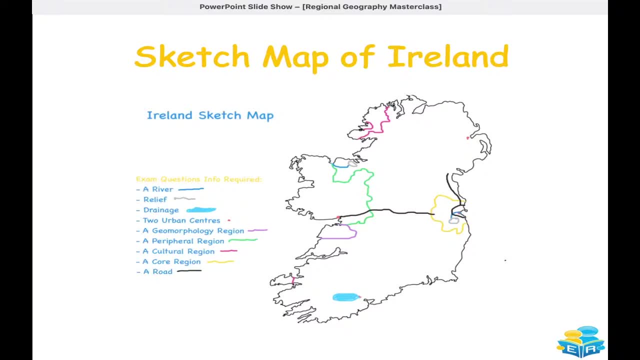 on a road, Okay, And I've put all of these- uh, I've put all these things like these, um into into the map here, Okay. So if it's like the core region of the GDA, if it's the peripheral region of the Western, 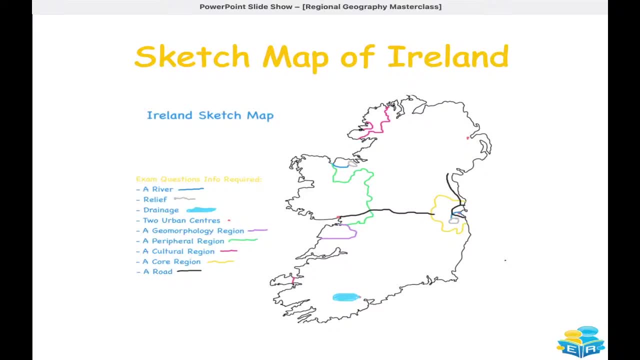 region. um, if it's the, the urban centers, you know I've put in Cork, put in Belfast, then Galway put in Dublin, Okay, So, Um it's. if it's looking at cultural region, like the Gael talk, it's, we've got everything. 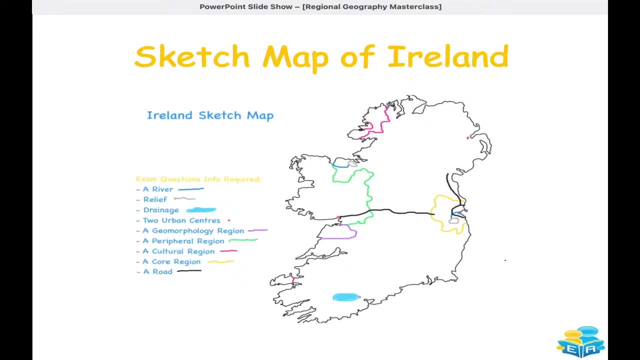 like put in here that you can possibly need. if it's the relief, it's the like low mountains, if it's the roads, you've got the ring road, M50, and then the M1 going up, going up, uh, past the dock there. 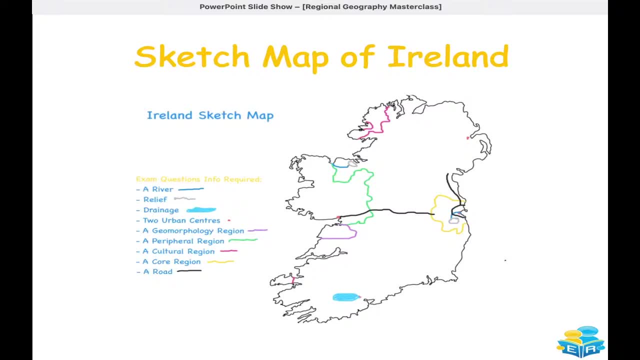 So like it, it, everything is, is put in here for the last um 15 years. So there's nothing that that, that will, that hasn't, that hasn't moved in the last 15 years, that that's not on this map, on this sketch map. 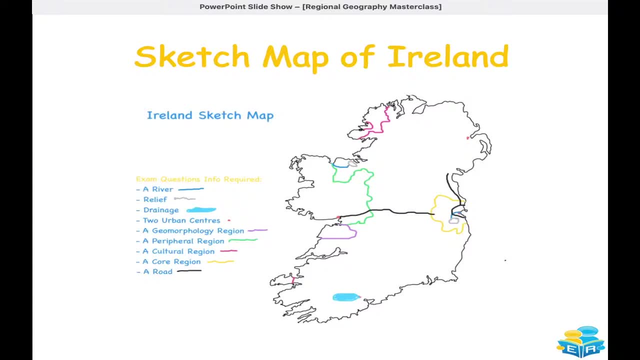 Okay. So, if you can- you're aware of everything on this map- you will be able to score um 20 out of 20 marks. Okay, A little tip for you guys is to use your legend. Okay, So you're given a legend. 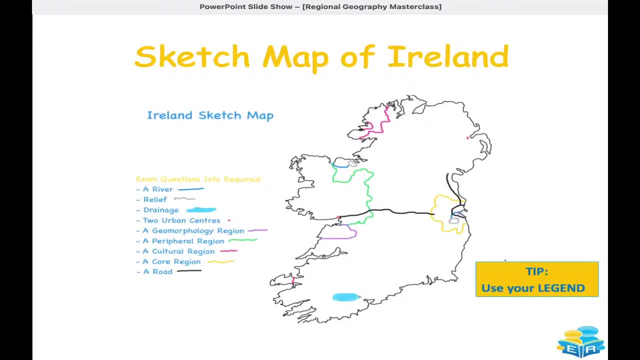 Um, so the legend is what you use with your OS maps And if you look down on the legend, you'll see an outline of Ireland. Okay, So if you don't know what I'm talking about, if you've got exam papers, open up your exam. 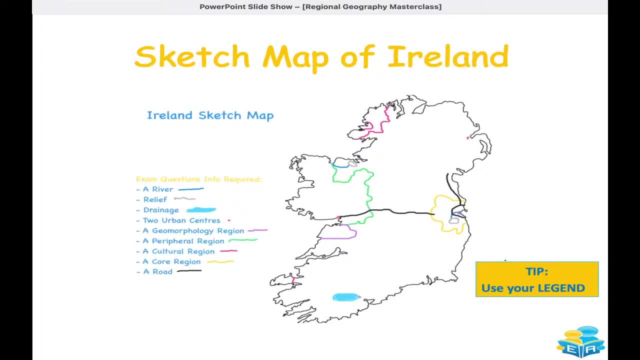 papers and you should see in the legend Um, You should see in the legend uh, the little it'll have, like all the subordinates um for Ireland and we'll have, like Ireland like, drawn out in, in in a small um, like the like. 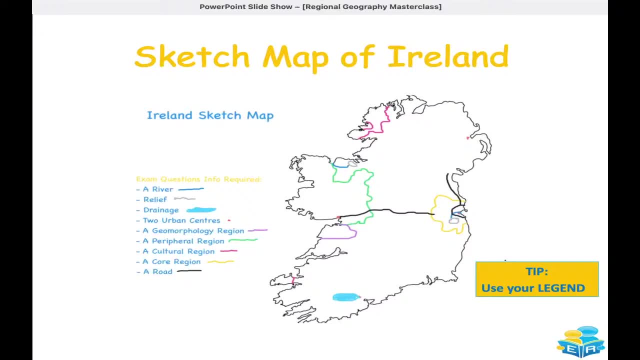 the sketch map of Ireland. So you can just use that on the exam to, to, to, to draw your sketch map of Ireland. So Ireland is a very, very easy one to draw. Also, it's one. it's it's where we live. 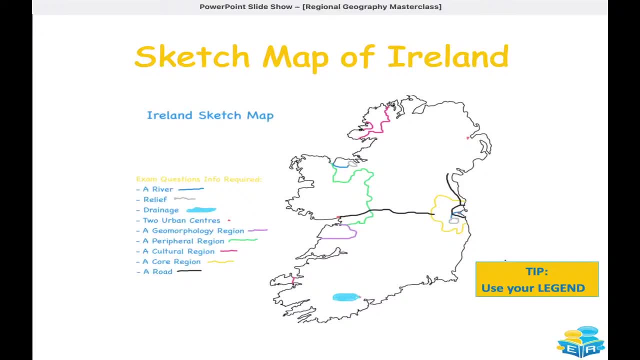 So it's. it's one that we're quite familiar with, but you do need to practice drawing it, because it is most of the memory. Um, if you're not, if you, if you're not practicing it, it can be. it just makes it a bit harder. 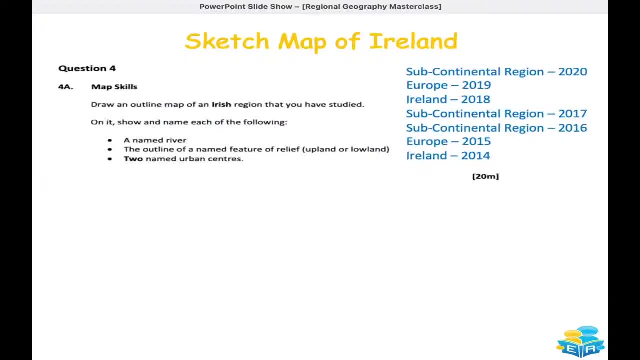 than um to be accurate in the exam. This is a typical question that comes up. Okay, So uh draw an outline map of the Norwich region that you've studied on it. uh show a name each of the following: 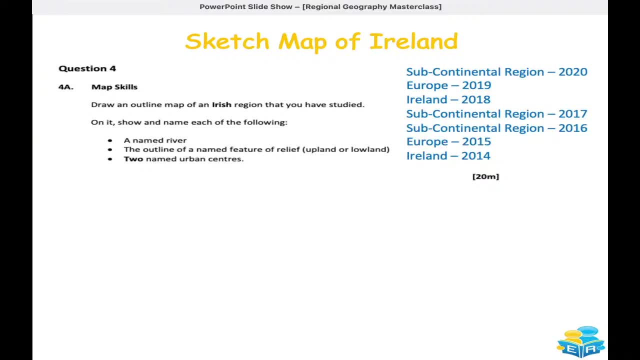 So I named the river, outline of the name, features of relief, so upland or lowland, and two named urban centers. Okay, So this is like the key for what has come up in the previous years. Okay, And my tip would be to make sure you draw, like the, the, the entire outline of the. 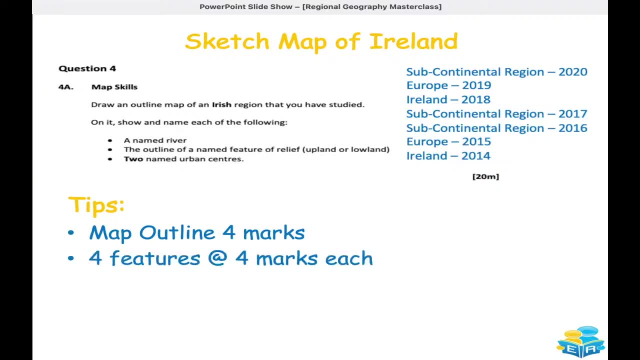 of the map. Okay. So if you're asked to draw like a region, so you're going to draw. maybe the GDA make sure you draw the whole of Ireland, Okay. So sometimes they just draw like the small region, just draw the whole of Ireland and 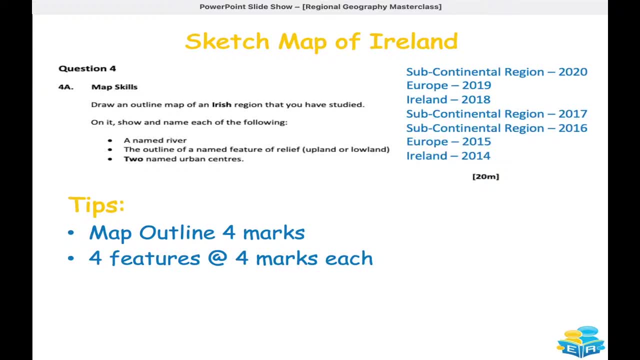 then put the region into, uh, the sketch map. Okay, So if it was like here: draw the whole sketch map of Ireland and then put in the GDA, um, so it's four marks for the for the map outline. 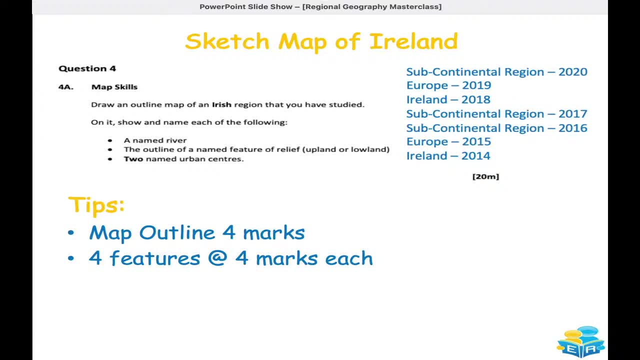 So that's what you want, That's what you will get, And then you each feature. so you're asked to put in four things. So one, two and then two named urban centers. So there's four features there. They're going to be worth four marks each. 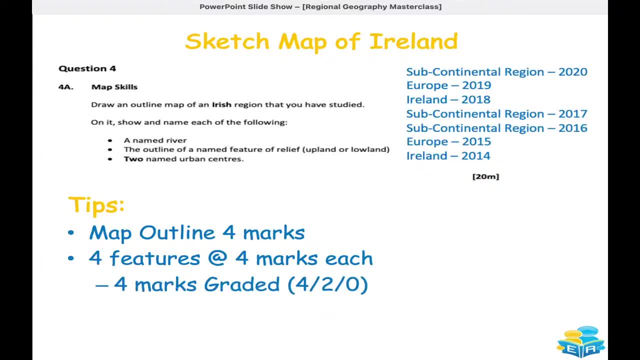 So four marks each. So four by four is 16 plus. you're getting your four marks for your. your map outline How the features are going to be graded, how they're going to be marked by the examiner, is they're going to be going to be going to be given four marks? 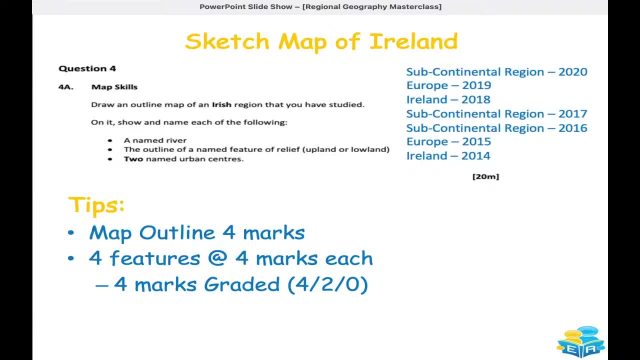 You're going to be given two or going to be given zero. So if you show it, okay, And it's going to be graded to one or zero, Okay. So if it's shown, but- and it's accurate too, if it's shown, but it's not very accurate. 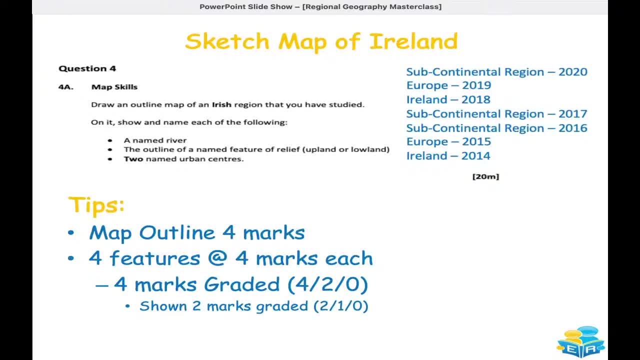 you might get one or zero, depending on what the examiner feels how, how inaccurate is for naming it. You're getting two marks, Okay, So that's how the four marks is broken up for each of the four features. Okay, So it's really important that you're that which you're drawing. you're accurate with. 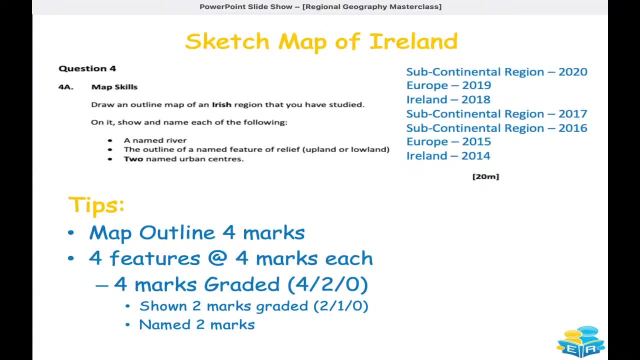 your sketch And it's important that you're also naming Um The feature, Okay. So if you're naming the river, say the river Liffey, Okay, So you put that on the key and then you'd put in where the river Liffey is and it needs. 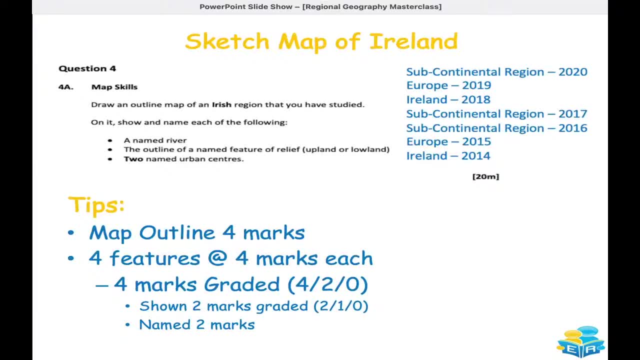 to be accurate. If it's not very accurate, but it's it's, it's it's fairly accurate, You might get one. If it's it's, bang on, It's perfect, You're going to get two. 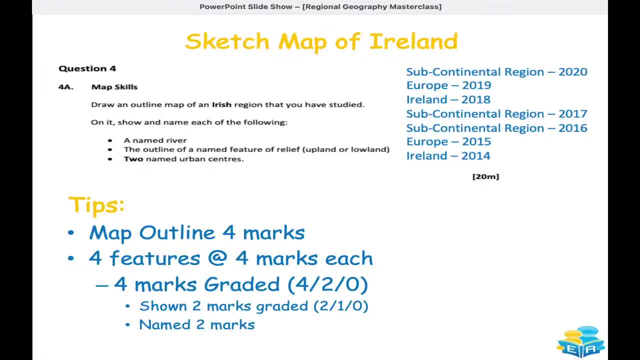 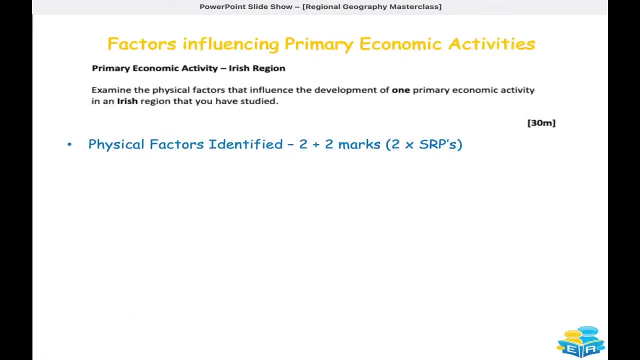 And if it's it's not showing or it's it's, it's it's way off, you'll get zero. Okay, So it's um, it's important that you're aware of how it's graded. So that's how the 20 marks goes, really easy to get those funny marks, and everyone should. 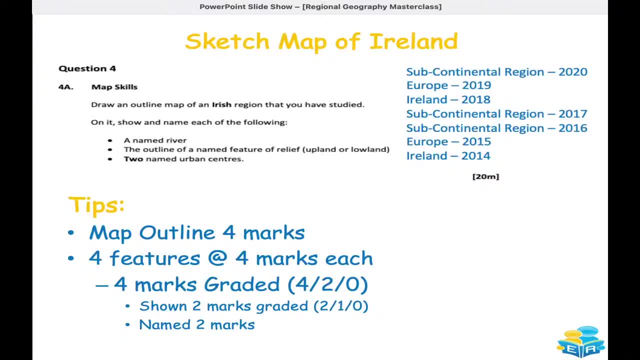 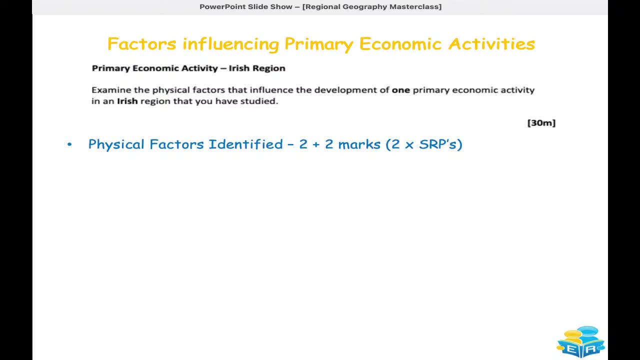 be aiming to To Like, Like to get them Okay. So we're going to look at uh factors, influence and primary non-activities. This is something that I think is important. You need to know. um would be something that, potentially, is going to come up in your 2021. 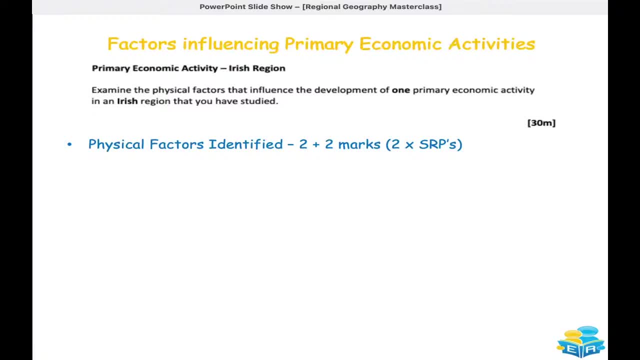 paper And it's it's important. I think sometimes students they're trying to work out, they're trying to write 15 SRPs and they can try to. it can be they can find it like overwhelming and they can't. maybe. 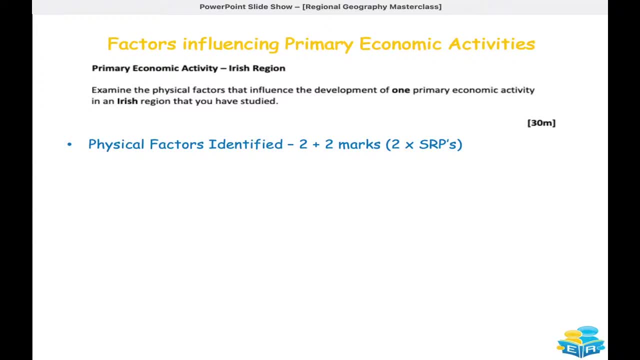 get. they're writing essays and they're getting maybe 20 out of 30 to get 10 SRPs. It just can't seem to get like. how do you get like your 24,, 26,, 28,, 38,, 30, how do you? 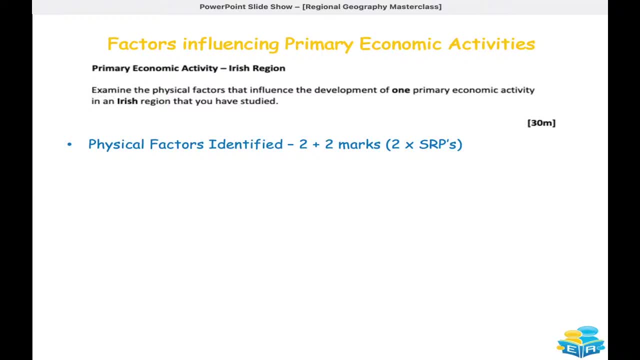 get the top marks And I'm just going to show you like, um, how lots of students like don't get pick up on easy marks And if you, if you leave out some of the easy marks, then it's more difficult to to get. 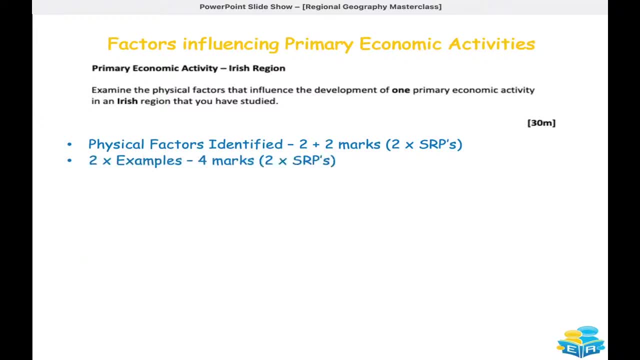 your, your 38,, 30 or 28, um and to to achieve then your H1,, H2,, uh, H3 in in like overall in the exam paper. Okay, So physical factors. So this question says um examine the physical factors that have influenced about one primary. 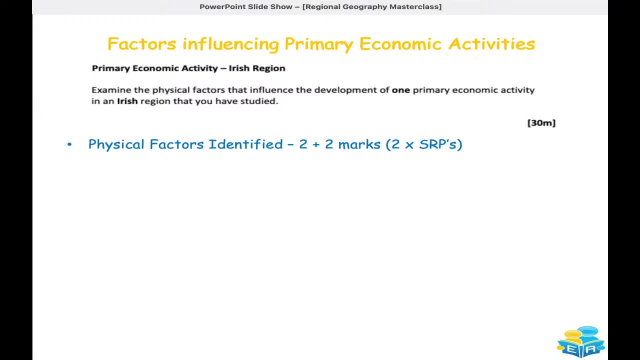 economic activity in Irish region that you've studied. Okay, So physical factors identified. So if you identify two physical factors, okay, you're getting two SRPs. So you're getting four marks for just identifying physical factors. Okay, If you then give two examples, okay, you're picking up another two SRPs, you're getting. 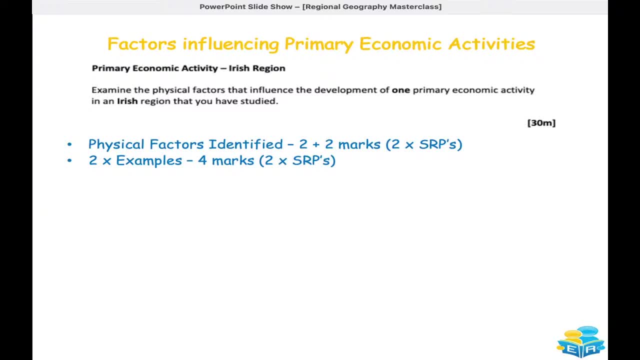 four marks, So for writing no more than four words. Okay, So no more than four words here for, like writing, uh, two physical factors and then writing two examples, you're getting four SRPs, eight marks. Okay, So really really easy marks to pick up and everyone should be, should be picking up these. 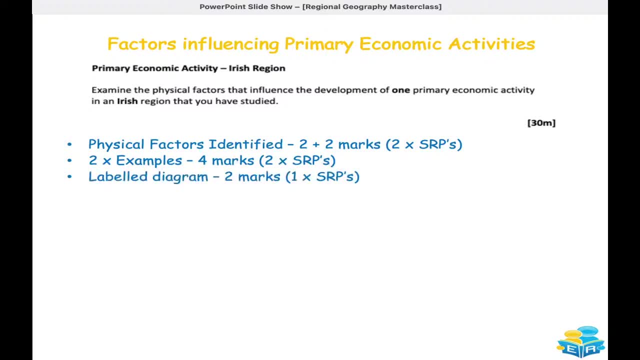 marks, Then if you draw a labeled or, even better, an annotated diagram, you're getting two marks, So you can get one third of the question. Okay, So one. you can get 10 marks out of 30.. One third of the question. 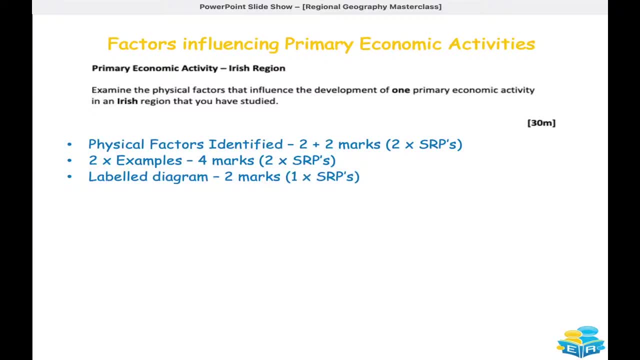 Okay, One third of the paper of this question, but just writing two physical factors, which is going to probably be two words. okay, maybe three or four words, but and then two examples. and there are two words and you draw a, you draw a diagram and you annotate it. you can. 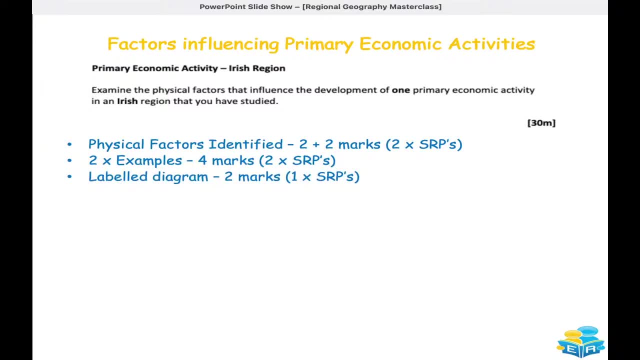 pick up you. you'll have already picked up 10 marks, Okay, And these are marks that students don't um, like, don't, like, don't get straight away. You need to be getting these right at the start of your essay. 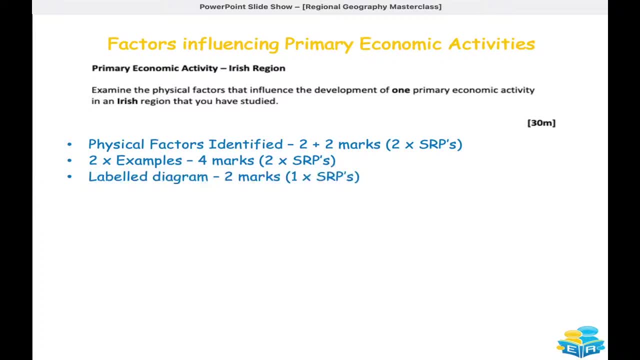 So, um, and that makes it much easier then to to get the remaining 20.. Okay, The the remaining 20 marks with just only 10 SRPs then. So it's much more manageable and achievable for students then to score the big marks then. 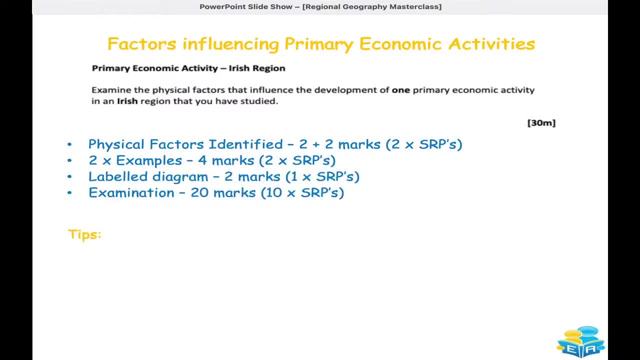 Okay, So examination then: 20 marks, 10 SRPs. Some tips for you? um, it would be to put examples at the start and at the end. As an examiner, you have to- uh, you have to- put yourself in the examiners like shoes. 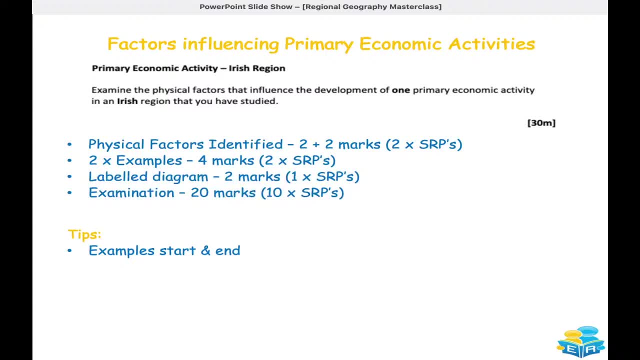 or correct in like June and July. Okay, Um, You've got X number of scripts that you're going through, Um, and it's it's very tedious and um, it's going to take like a it's, it's take it's. 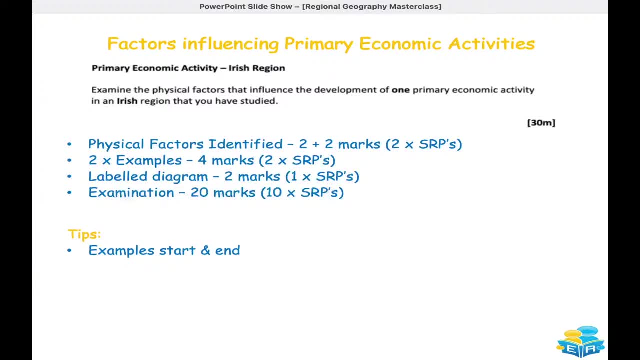 it's a huge amount of of work and time and what you're, as an examiner, you're in like in this zone where you're you're looking out for specific things. So like, for example, with this question, you're going to be looking out for physical 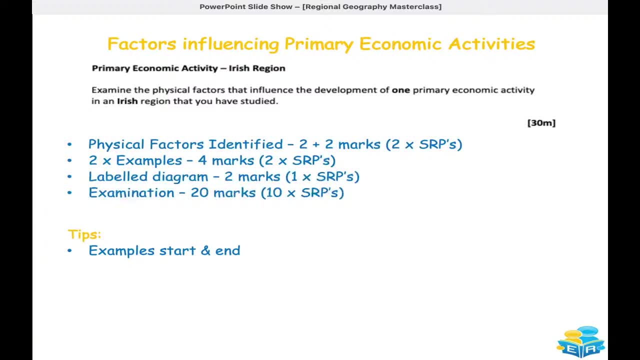 factors. When you put in the physical factors, you're going to tick, tick and SRP, SRP Examples- SRP, SRP. Okay, So a little tip is to put like the example to the start and at the end of the question. 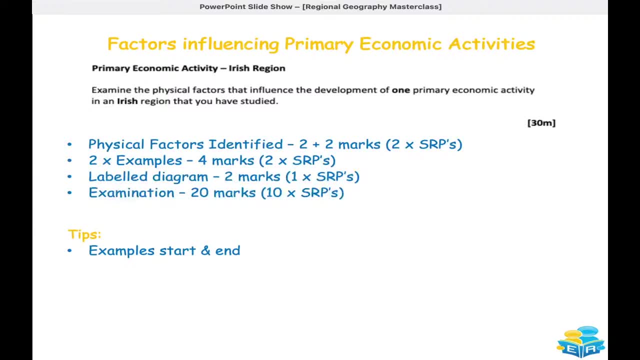 because maybe, just maybe, the examiner might give it an extra. you might put a two SRPs, uh, for example, to the start, and maybe you've put the examples at the end, And if you change up the examples you might just get an extra SRP. 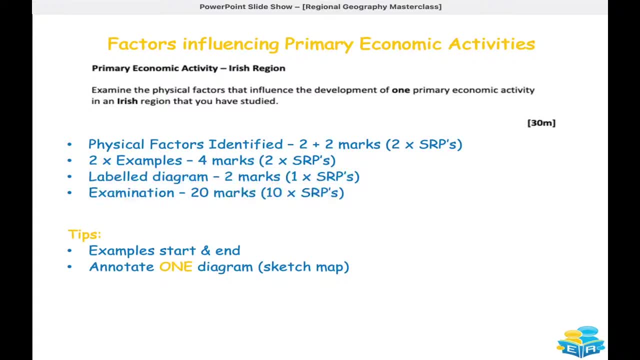 Okay. So that would be a little tip: annotate one diagram, Okay. So don't draw like lots of sketches and lots of diagrams, Just do one, but annotate, annotate that diagram and annotate it. well, Okay. And another thing is, like students say, what, what, what will I draw? 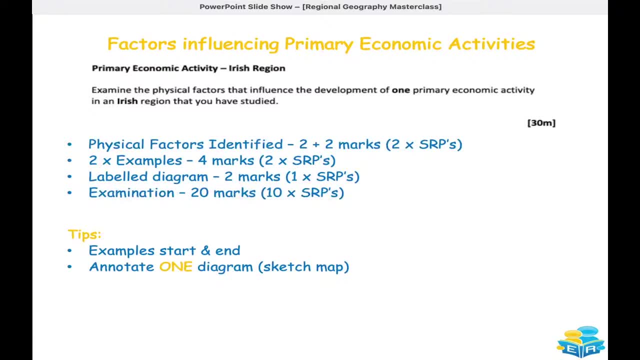 I'm not sure what, what, what I should draw. Well, if it's the Irish region- and you've practiced drawing the Irish region, you, you, you can draw it like that's your sketch, Okay, And then put in your primary economic activities link at the prime. 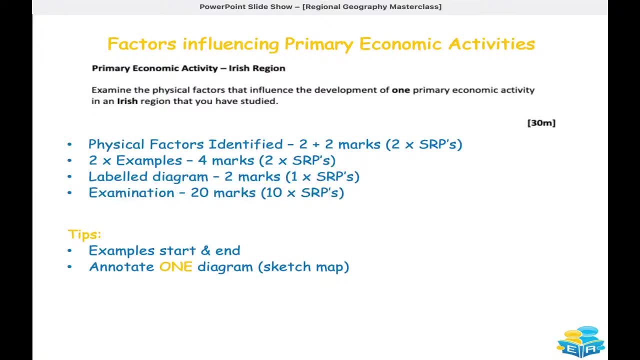 It has to be linked to, obviously, primary economic activities. but draw the Irish region, put in GDA and then put in some annotation about primary economic activities then and that, that, that, that you, that you've learned and that you know about, um, and that will. 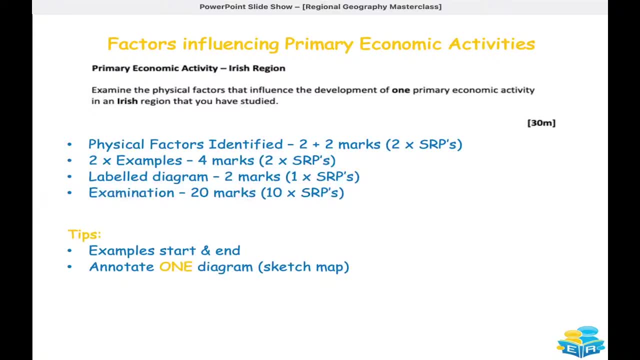 score you at least one SRP and potentially, depending on how well you annotate, Get you uh, two, three, four, uh SRPs. Okay, Uh, important that you focus on one primary economic activities, Okay. So the question says here in bold: and be careful. 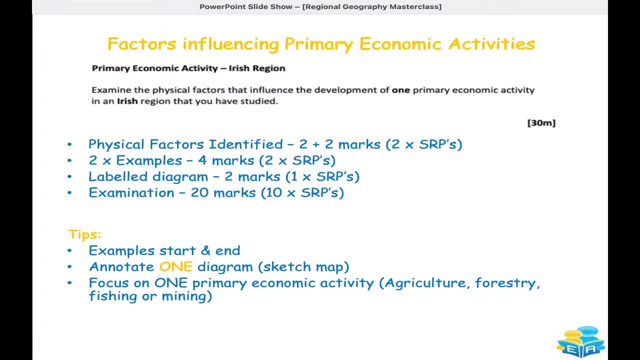 They're very. they don't try to trick you in the exam. Uh, the exam is always, like, very fair and it will always have everything that's really important, Like if it says and: or if it says or. they usually put it in bold. 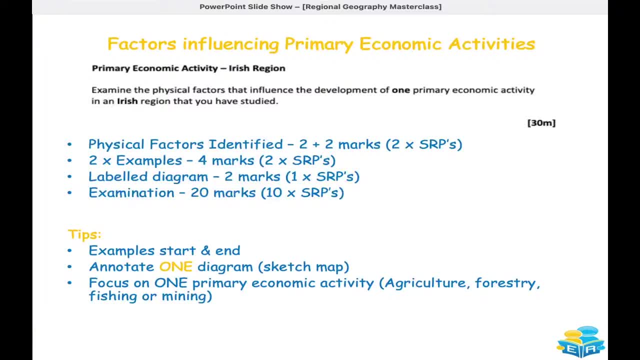 Okay, So this question says one primary economic activity, So you must just focus on one. So that's maybe agriculture. It might be forestry, might be fishing or might be mining, but you can't talk about culture- sorry agriculture- and then talk about forestry as well. 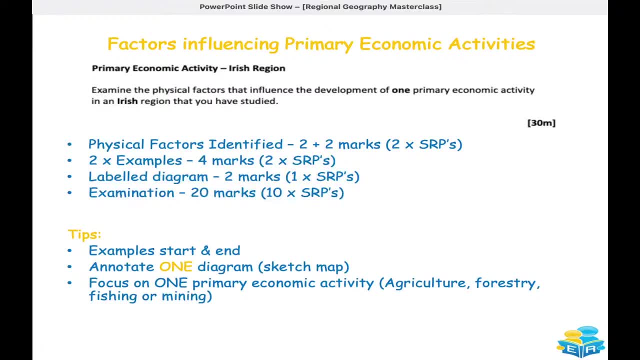 If you do that, what will happen? Okay, The examiner will mark it, but they will, And then there's. so they'll mark it based on all agriculture and then they'll mark it based on forestry and then take whichever one was. you scored highest in. 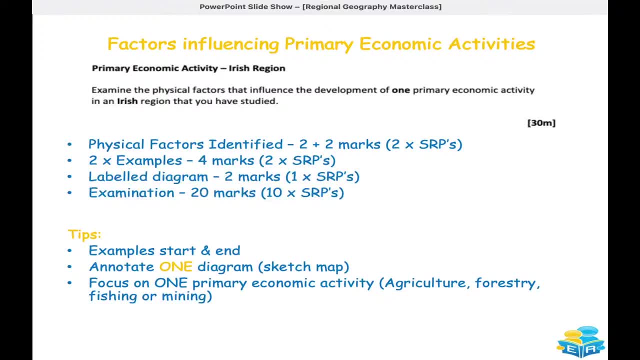 Okay, But they won't give you marks for both together because the question just says one: Okay. So again, be aware of the question. And that is so crucial, And where it can be a downfall for lots of students is that they don't read the question. 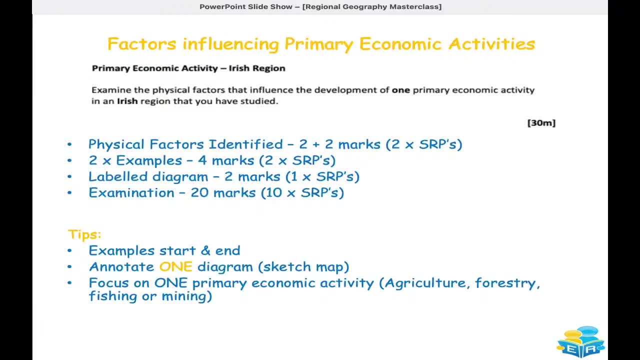 and then therefore, they don't answer the question. So I did say at the start to reword the question. reword the question a number of times, So the one primary activity that I focused on is agriculture. Say that maybe three, four times in your essay, just so you keep focused and you stay on agriculture. 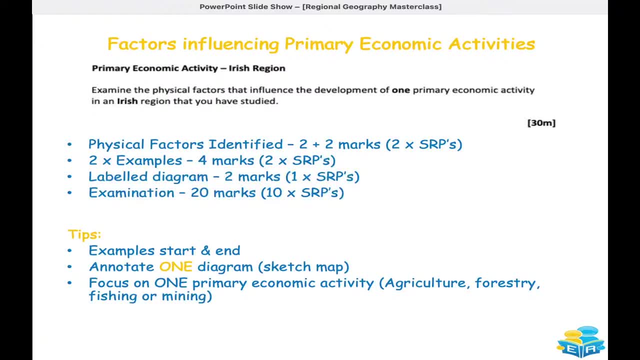 if that's the primary economic activity that you're focusing on, Always start on a new page, Okay, For each question. So so, so, so, so, Okay. So often you see, like when you're, when you're marking exams, um, that students like to do. 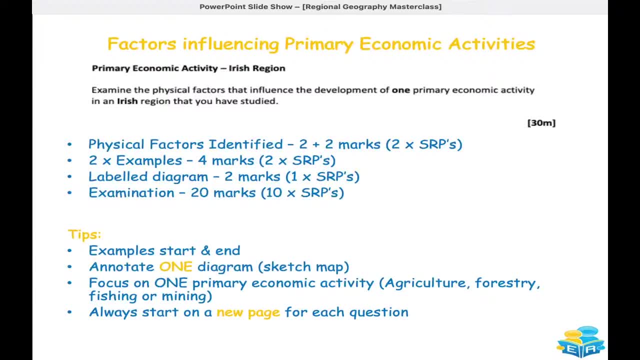 part A and they'll have part A in here, Okay, And then they might start part B, Okay, And they'll do part B all the way down And then like, if you imagine, like this space down here, just like the one line, okay. 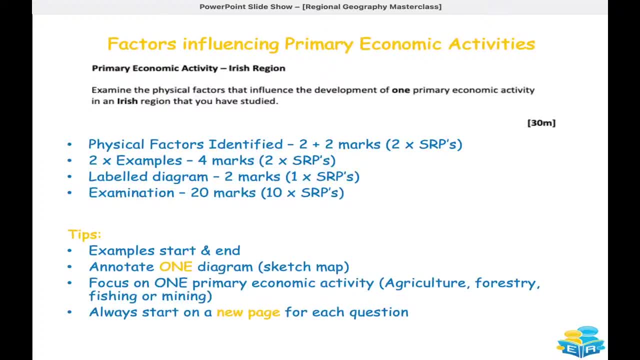 There's only one like line left before the end of the page And what happens is then student like finished and they've got, say, their part B finished And then later on they have to remember: oh I need, I didn't put a diagram in. 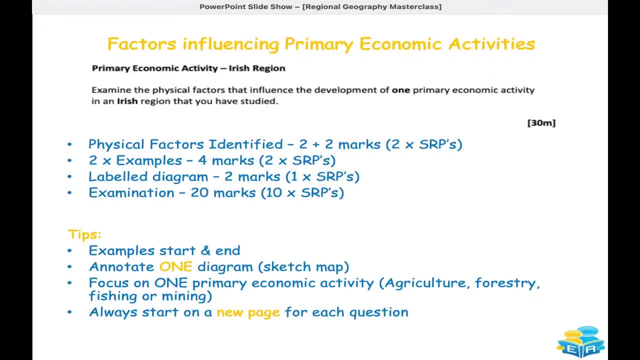 They draw the diagram really, really small down the one line because they can't go on the other page, Because they're not in a space or they might remember some fact or some another SRP, and they're writing like five lines in one space. 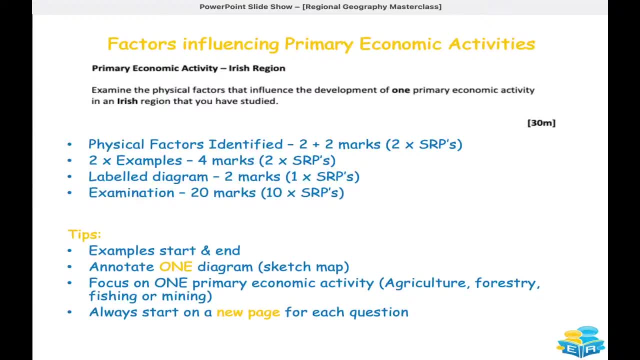 Okay, That's probably not going to score you, And if it is going to, if you are going to get marks for it, it might just be. it's probably going to be one, even though you could have potentially have three, four SRPs squished. 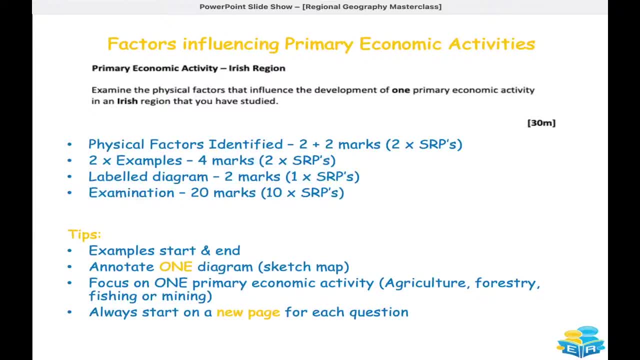 into the one sentence, Okay, So it's really, really important that you start on a new page for each question. So do part A, even if it only takes a few lines. go onto a brand new page, Because if you think of anything later on, you can go back and you can put it in. 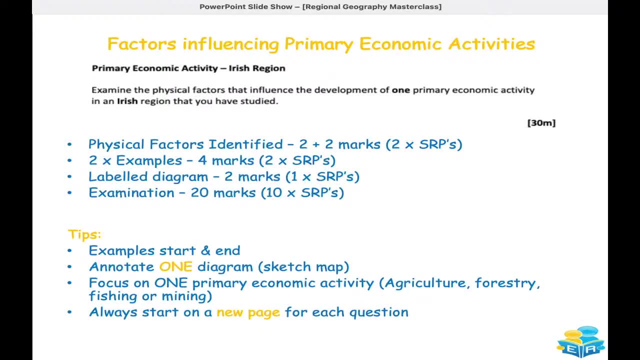 You've got space Also for the. for an examiner it's much easier to just to see the questions. It's laid out easier. It's much more examiner, like like user friendly. So don't pack everything in to into one page, like do part A and then, if it gets to half, 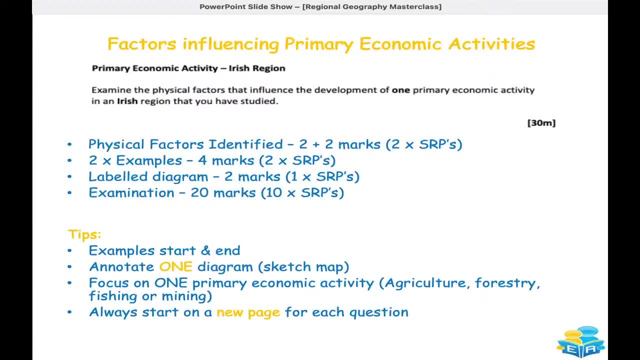 the page and you're finished, go onto a new page, do part B. If you do B and part B and it goes on for a page and you go onto the second page and you write two sentences. I wouldn't do C underneath it. 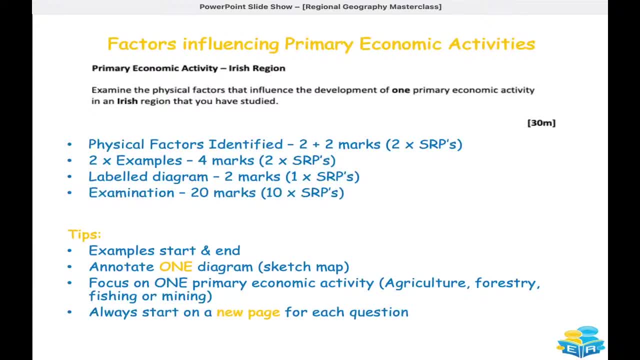 I'd go onto a brand new page and do questions, If I have any, if I ever, if I think of anything, if I, if I've got time, at the end I put a diagram I've got, I put some fact in there. 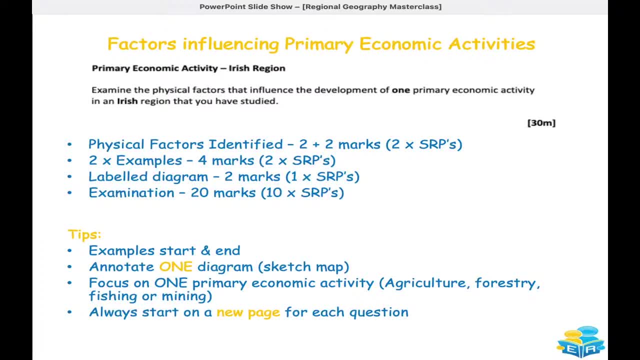 Remember maybe in the short questions, some information after getting that is relevant to my what I was talking about. I can then use that like so be, like be aware of, like exam examiner, like marking this and put them and laying it out like really user friendly for for the examiner. 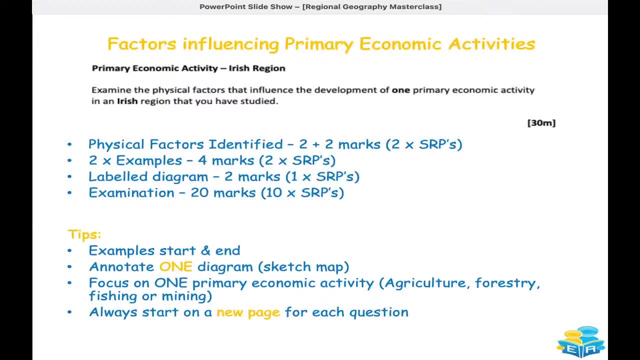 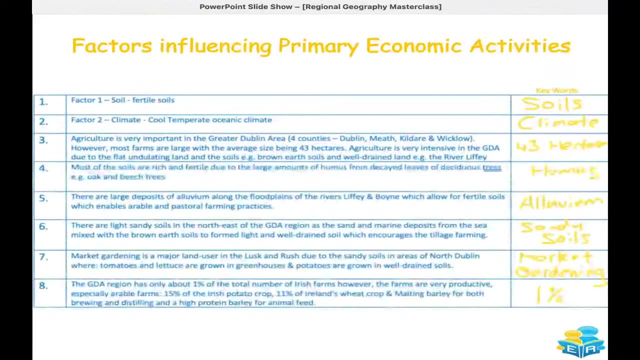 but also for you. So if you think of anything, you can put it back in. So that would be. another tip of mine would be to start every question on a new page. Okay, So this is like an example, then, of of this question. 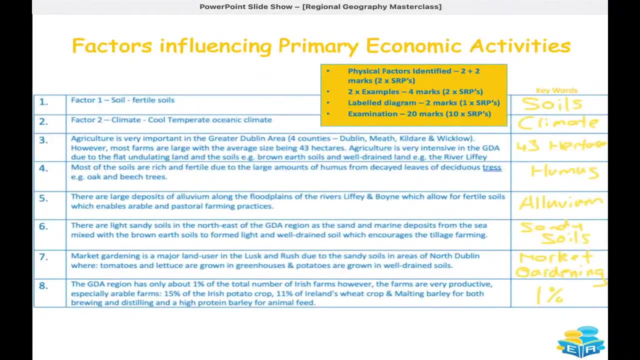 Okay, So I'm not going to go through. we've already spent, 35 minutes is taken, So I'm not going to go through. like, like the whole, like question that the questions is. here's the sample answer You can like. you can have this once you look, once you fill out the description, you'll 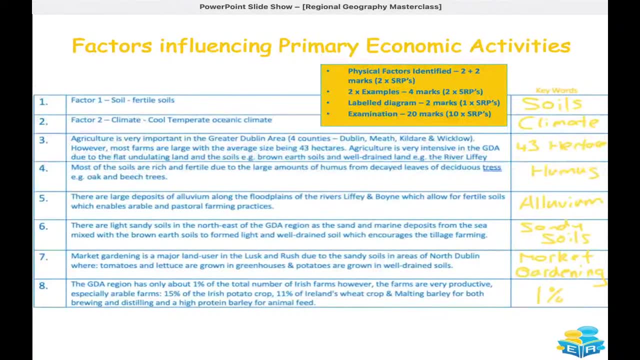 be sent out. all this, Okay So, but, for example, the physical factors case of straight away, you should identify them. So: fertile soils. Okay, That's my physical factor. And my second physical factor is climate: cool, temperate, oceanic climate. 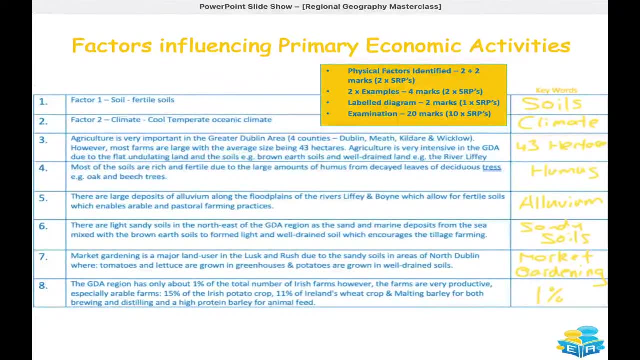 Okay, So I'm writing like a couple of words here: SRP, SRP. then you should give like, then your examples. two examples, two more SRPs, your diagram. Okay, So I've got the 15, when I would just say diagram. that's my sketch of Ireland. 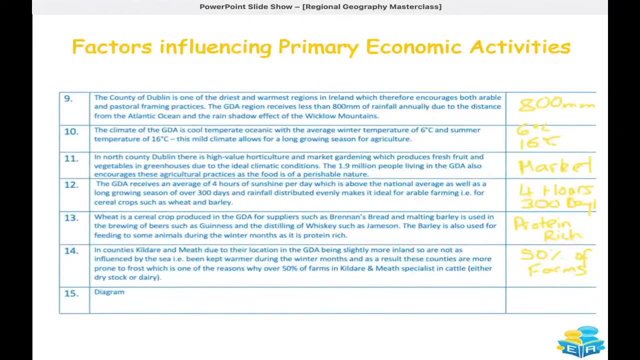 Okay. Okay. So I've got the 15,. I'm not going to do anything else because you're going to be using the same picture a couple of times, Okay. So just like just going to make sure I've got this all connected in place. 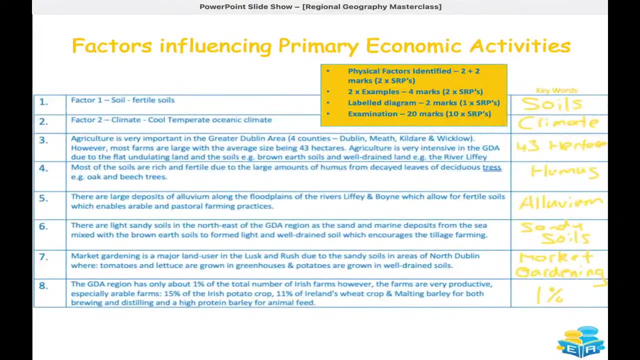 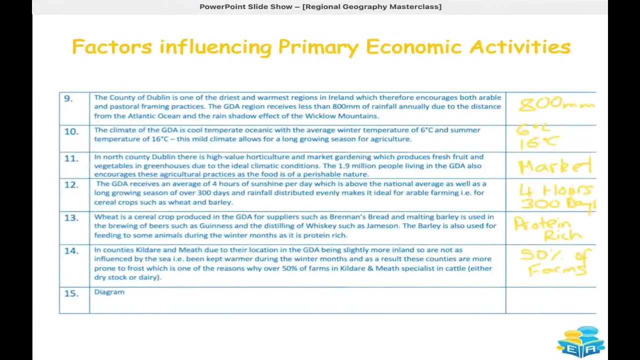 I've got the, the 50 that you can see here. with the 30s, you just go and you can see what the already have. Let's just make sure it is Yeah. So let's just make sure you can see what's in there. 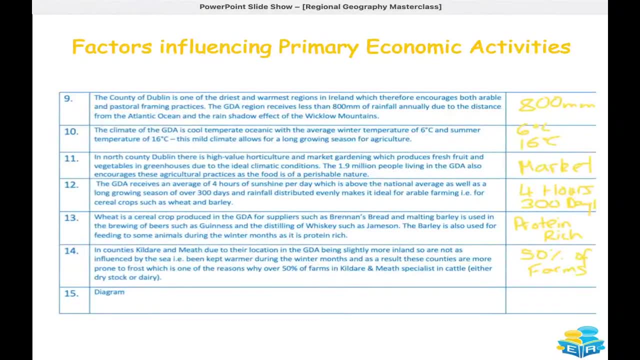 So let's make sure you you're going to see the 10s, Yeah, Yeah, 17 srps to get every examiner that marks it given a 30 out of 30, given a 15 out of 15, because there is- it is very subjective, like you know- one examiner could give something. 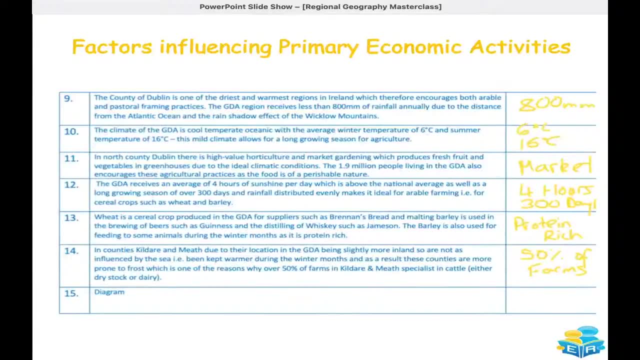 that could be 30 out of 30. another one could give it it could be 26 out of 30. so to to enable yourself to get 30 out of 30, you need to be aiming for about 70 srps. okay, and it's important. 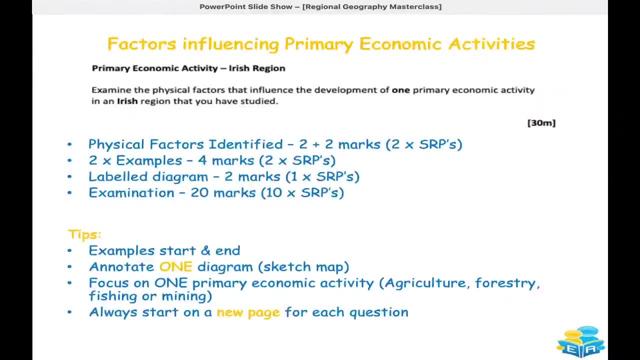 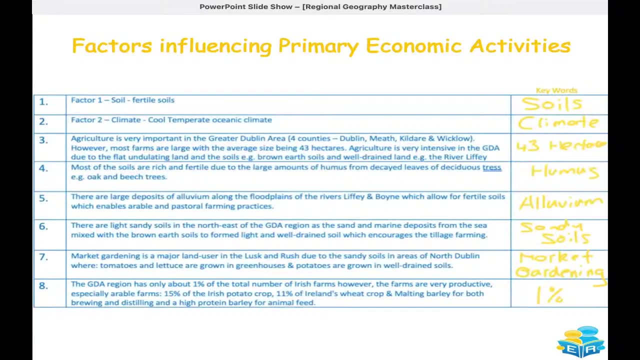 in our in our tip. i probably should have this in here. but another tip would be, about which your sentence is: make sure you, you, you don't, you put full stops in. okay, so put full stops in. and because if you don't put full stops in, if you just take it as like one big, uh, like one big. 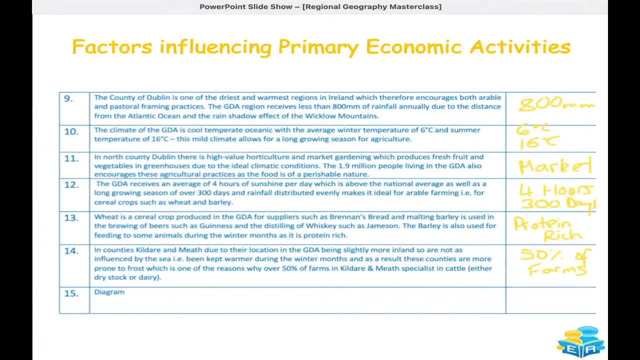 sentence it's only going to be one srp, where if you put full stops in and you've got like really concise, like points and you could have potentially have uh, one srp, that that, if you broke it up by putting full stops in, it then becomes two srps, okay. so that is something to be aware of as well. 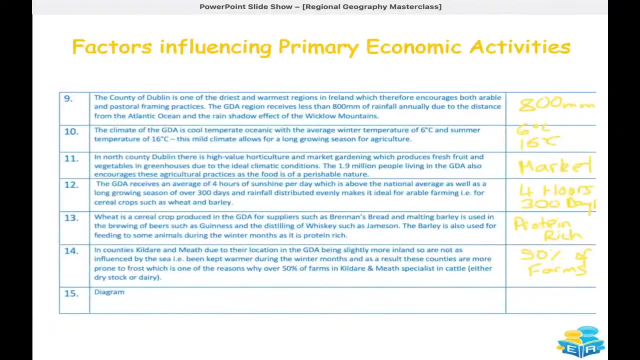 you need to be aware of that and make sure you put full stops in. okay, so that is something to write in short, concise. uh, relevant points. okay, so it's a significant relevant point, so it needs to be uh, short, concise and don't write like in so don't be like using connective words like that. 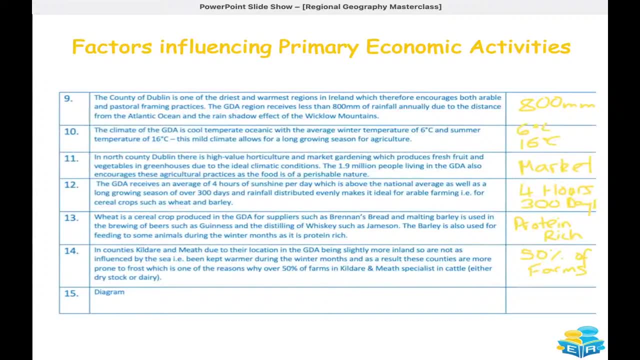 you might use in other subjects like, for example, like business. you know it's, it's all about developing your answers using connective words, but for geography it's it's really concise: um, like, like. well, it's not bullet points, though, but like, but it's, it's like a bullet point, okay, just. 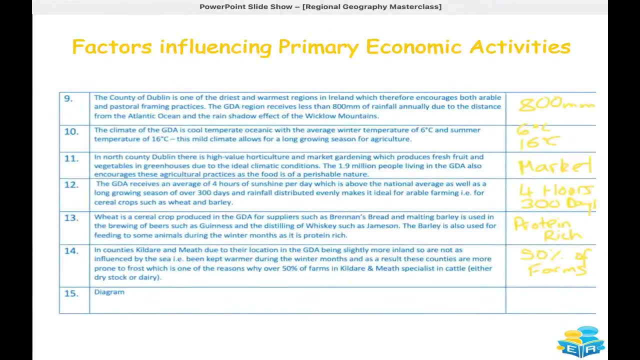 written in a sentence. okay, now you can. i know some students they use bullet points and it's you will. you will get away with it. but, uh, because there's the, the cohesion isn't isn't there for like the, for the 30 markers, but then it. you will be penalized then in the in, in your geology, in your. 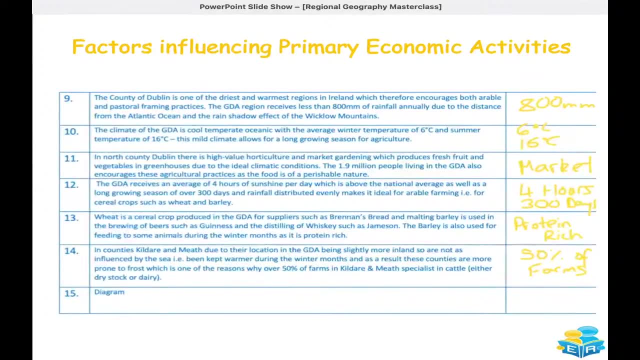 option later on. so so just write the sentence of short and concise, but put, but don't write them really long- and develop them into each other. just put a full stop and then you can develop on to that point then, because that could become. it could become then two s or a piece. 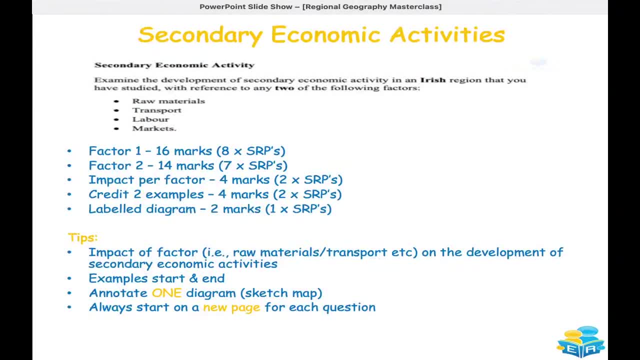 so the second one, for ireland, is looking at secondary economic economic activities. okay so, secondary economic activities, um. so this one here is looking at, um it says, examine the development of secondary economic activities, an irish region that you've studied with reference to two of the 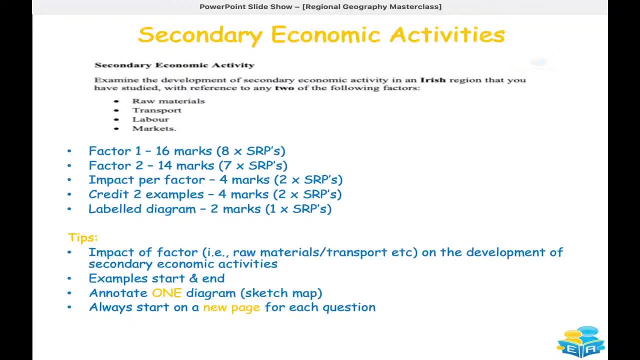 following factors: okay, raw materials, transport, labor markets. so it says two of the following and it says an irish region. so you're like: okay, right, i'm going to pick my irish region and then i must pick two factors. i can't do three, can't do one. it says two, okay, so you must do two. 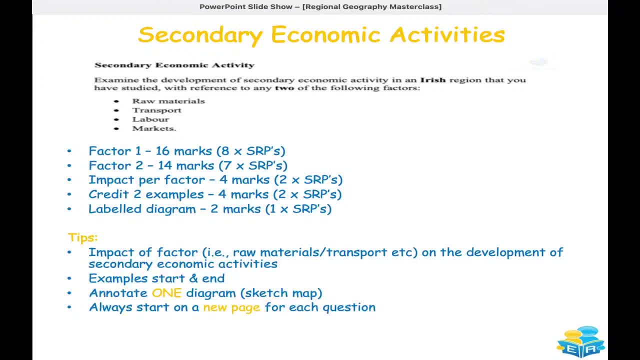 so, if you do, one factor is going to be worth um asrps and the second factor is going to be worth seven srps. okay, so you're looking at 16 and 14. it doesn't matter which way. that is okay. so factor one could be 14, in fact two, if you were at 16. so it's important to to show the impact of the factor. 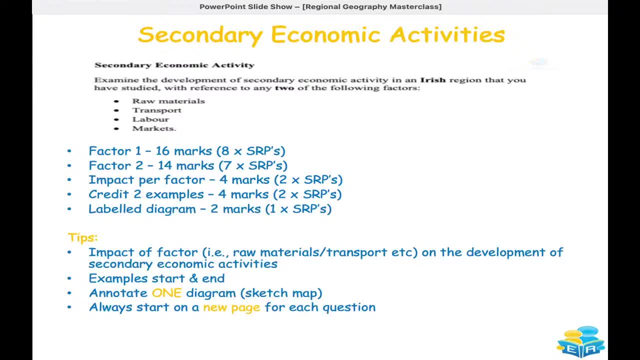 okay so the impact of uh, of this factor on the development of secondary economic activities, and there's a mark for each factor and there's a mark for each factor and there's a mark for each factor going here. okay so, if you can show um, how like, if one a factor of like uh, of transport, how that's. 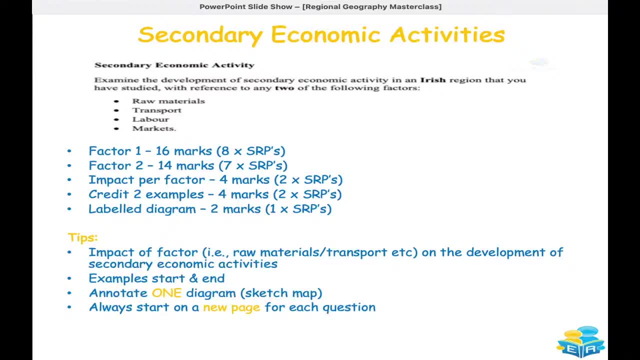 led to the development of secondary economic activities. you can get an srp and then do the same for its labor, raw materials or markets. you can get four marks, two srps, then credit two examples, okay. so if you can give two examples we're looking at, then another four marks, so two. 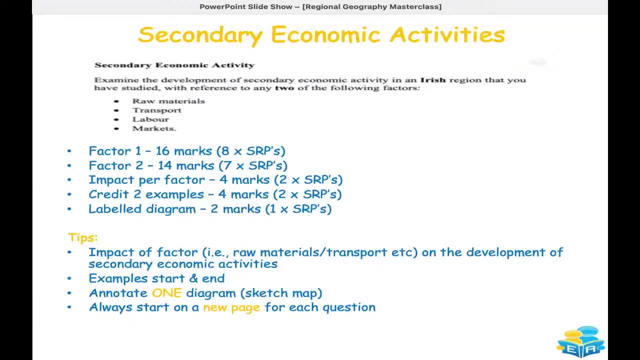 srps. again a label diagram. it's two marks, one srp. so here we go, we've got, we've got our 10 marks, we've got our five srps, and we haven't written that like very much in the paper, so it then it makes it much easier then for us to be able to get the rest of the marks then. okay, because 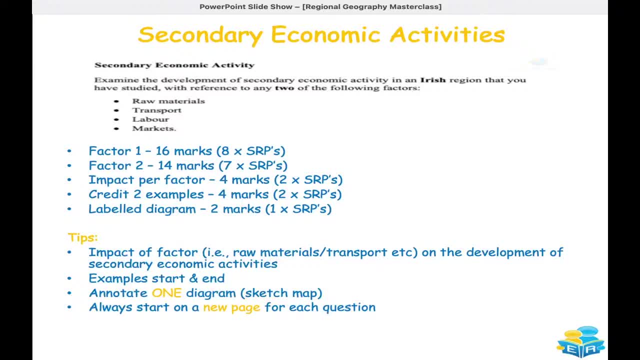 instead of this now becoming eight and seven. we've already brought this down to to maybe six and this down to, uh, to maybe four, depending on on what you've. if that, if you use the diagram for that, one, okay. so it's much easier then to to get the mark. so maybe it's five and five, okay. 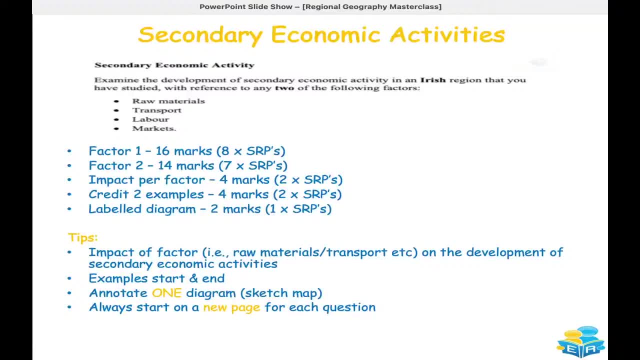 and they've. they've have to bring it down too. so when you're talking about the impact of the factors, so it might be like that, like that's like raw materials or transport- has to be about how, how this is like led to the development of secondary economic activities. so again, reword. 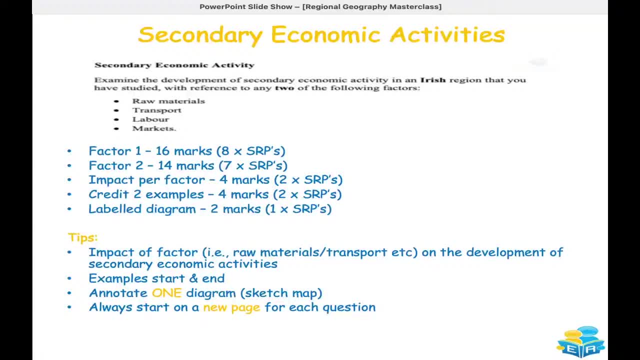 the question. make sure you reword the question because it keeps you focused, it keeps you then in line, it stops you going off on a tangent and be aware of the things that's in bold. okay, so it's an irish region. it's two factors, okay, um, examples again at the start and at the end. 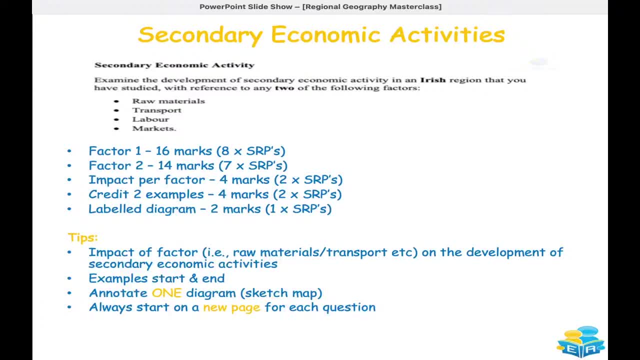 if you can come up with different examples, even better. okay, but examples at the start, examples at the end. annotate your diagram. okay, just do one diagram. don't do more than one. okay, but you can put as much detail as you want into into one diagram. you can pick up. 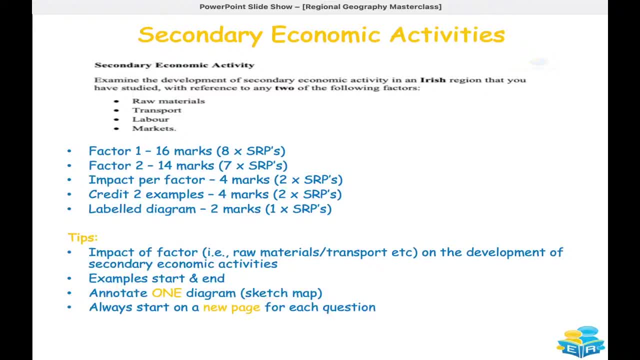 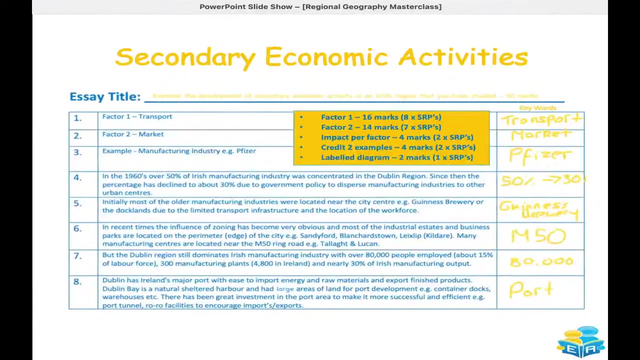 uh, you can pick up um, a number of srps, not just one, and you can pick up a number of them, depending on how well you you annotate, and always start a new page again. i'll have the sample answer here. okay, so factors here: transport, market, and then going into 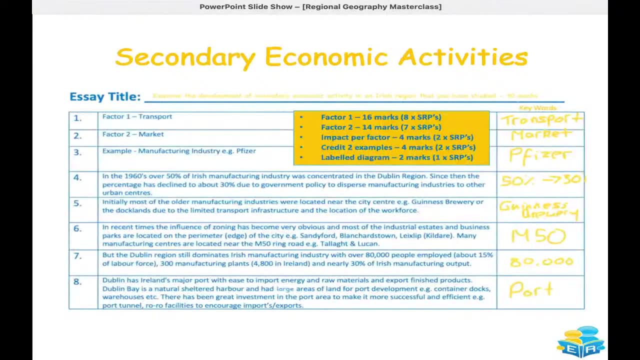 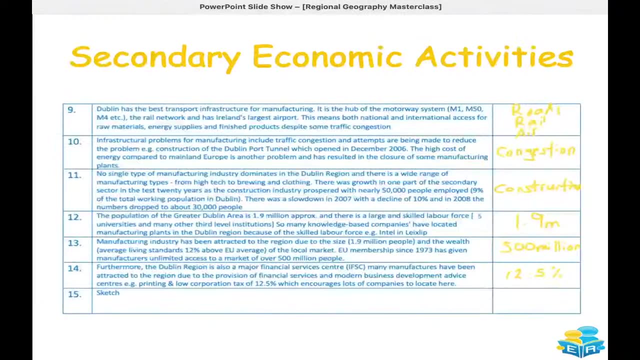 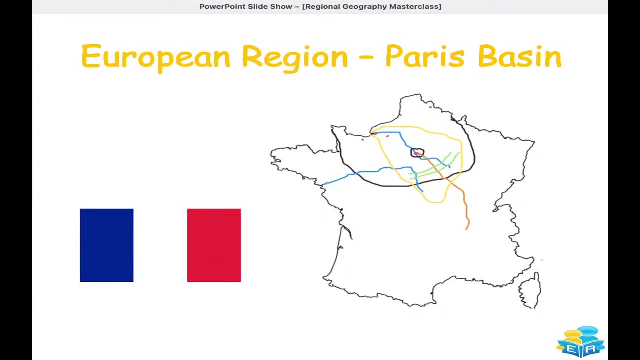 then the examples. we're going to have our diagram here, okay, our sketch, and then we're given like really good detail. then in for our srps, then for the sample answers, okay. the next one moving on to is, um, the european region. okay, so the european region, uh, that i tend to look at is, uh, paris. 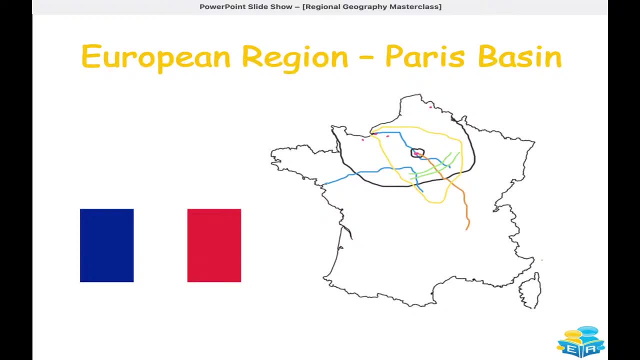 basin and the mesa journal, but particular focus. you should focus on the european. if, like you can, you can focus on one european region. i know the question come up where you're asked the trust. okay, and that come up in 2020, so might not come more than likely won't come up in 2021. 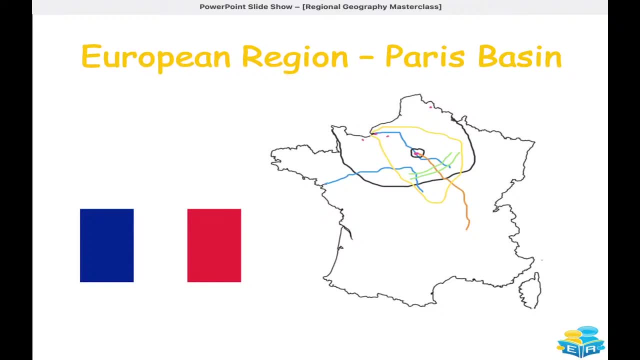 but you can, i would be focusing on one european region, okay, if i was a student. i've got a short amount of time, i've got a lot of need to study, a bit like right, and make sure i know my irish regions, make sure i know the paris basin, make sure i know my subcontinent, which for us would be. 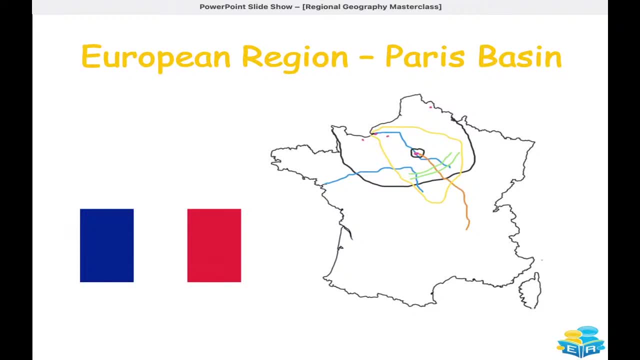 brazil. so and again i've went back for all. every time we're asked to draw like european region and and i've put everything for the last like 15 years into like one uh sketch here and that. so i know it can be a little bit messy, okay, but if you're asked to put in, say, um, oh sorry, it's gone. 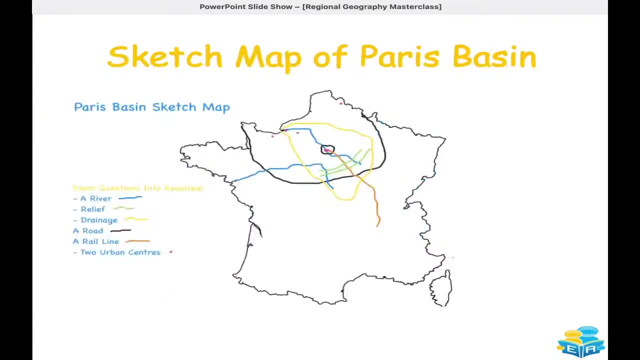 i've got it like here, okay. so if you're asked to put in, say, like a river, okay, so i'll put in like a number of rivers. so put in like the river san, put in like the river loire, okay. and we've got the boulevard. boulevard of perf- uh, perfique. sorry, i always pronounce that one there a little. 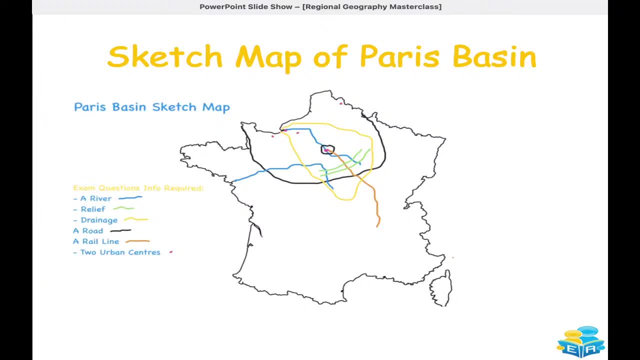 weird. um, we've got, uh, if you're asked to put in like the, the drainage, okay, so you've got like the, like the this area here, okay, which shows the drainage and it's the drainage of the river san. so here's the river sands which, just like this, is the area like going around, it's quite. 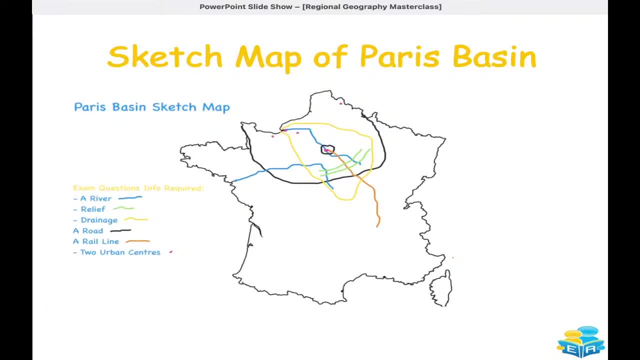 easy to remember. um, if you're looking at, um, the railway line, okay, so you've got the railway line uh running here. okay, the orange ones, it's going from paris all the way down to lyon and it's the tgv and which is operated by the se. 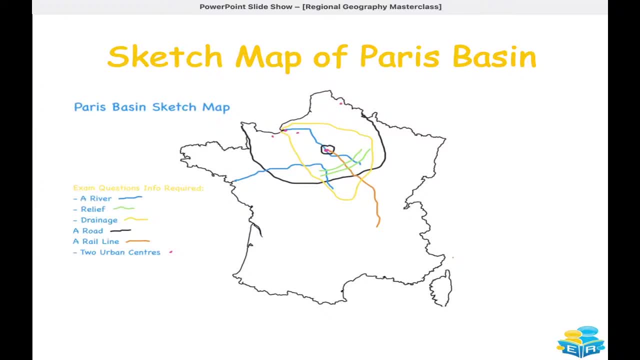 nf and if you're looking at you might be asked to put in like an area of like relief and lowland. most of the paris basin is lowlands but you have got some highland areas, the escarpments, which is like the green area here and where the dry champagne region, where they 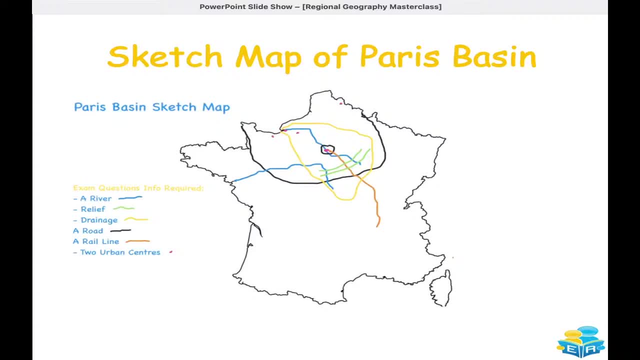 grow all the vines and you could be asked to put in urban centers okay. so usually you might ask like two urban centers, so you put in paris, you put in leo, you put in laharve or con um, so there's a number of different uh urban centers and you can put in like the tgv and the tgv and the tgv and 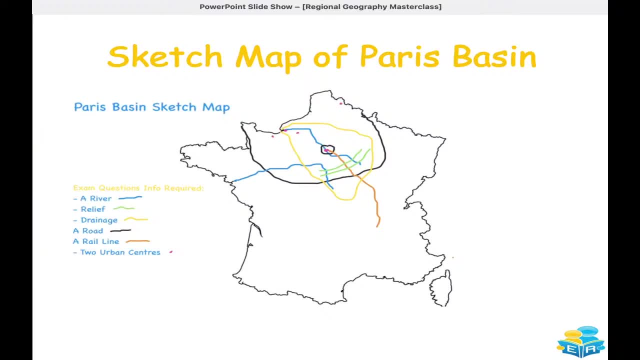 regions that we put in there. um, i haven't forgotten any, so, no, okay. so so these are again. you need to be able to to draw um your paris basin. okay, my, my advice would be to draw the whole of france and then put in paris basin. i just think it's find it easier that you'd be able to. 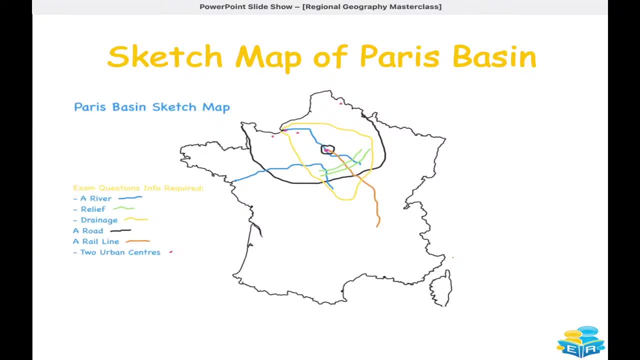 put it in um, particularly if you're putting in like, say, the tgv going into lyon you don't want to come in out of, like it does come out of the paris basin. so you, you want to. you want to display the whole thing, show off that you know how to draw. 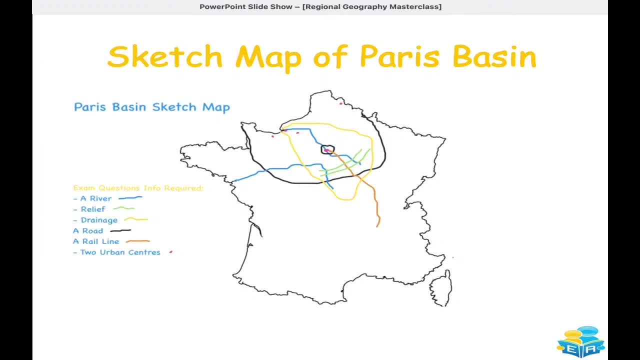 paris, oh sorry, you know, draw like france and then put in like the paris basin. okay, uh, top, and my really like top tip would be to practice. it's muscle memory. okay, so, this is muscle memory. so just practice, practice, practice. and if you practice drawing a few times, you'll. 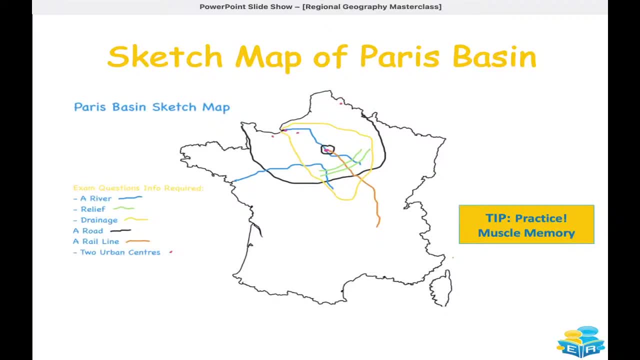 get good at it and you'll be able to- to always, uh, replicate it then, um, and you'll have no problem. then, whenever, if your question goes up it's a european question, then you're going to answer based on the paris basin. here's your sketch map, here's your diagram. okay, so the the next. 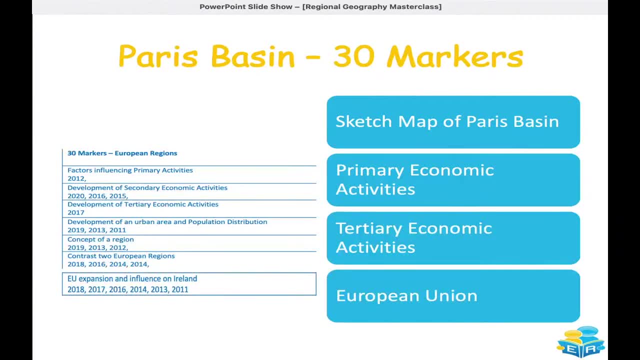 one is: i've again did the exact same thing: looking at all the different past papers and using exam revision to uh, to break it up by topic, and what i can see is: i can see the, i can see, like the all the different, like, like, uh, all the different questions that have come up. okay, 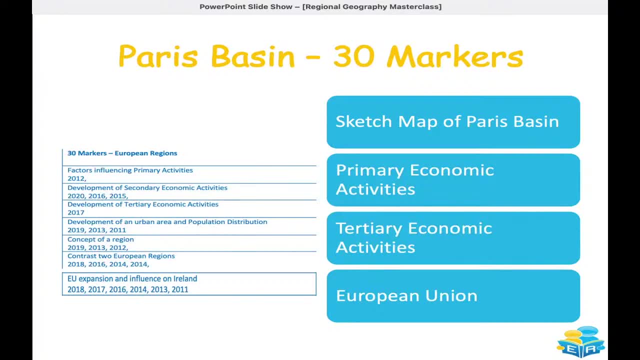 so factors influencing primary economic activities, development of secondary economic activities, development of tertiary economic activities, development of an urban area and population distribution. concept of region contrasting to european region. and then the next one is the european region's- uh, eu expansion and influence in ireland. okay, um, and based on this, the ones that 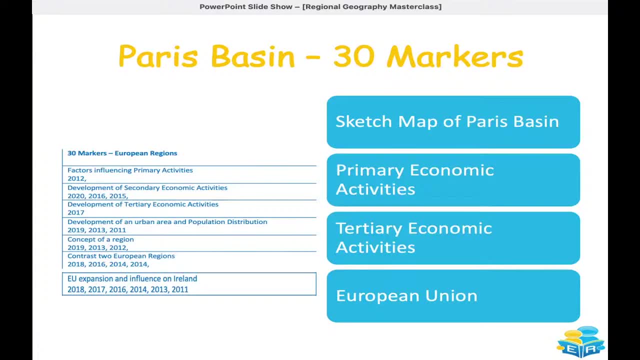 i would be focused on for this year. if i was a student sitting the paper in 2021, i'd definitely be able to do a sketch map of the paris basin. i'd be definitely know the primary economic activities. i would definitely know my tertiary economic activities and the european union. 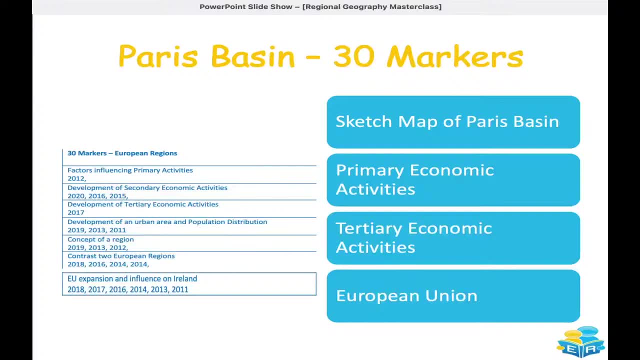 question, which is a very popular question. i just put it into, uh, i put it into the into the european region here, because it's it's. it's relevant that, because it's a it's the european union. so, um, if the question is something like account for development of 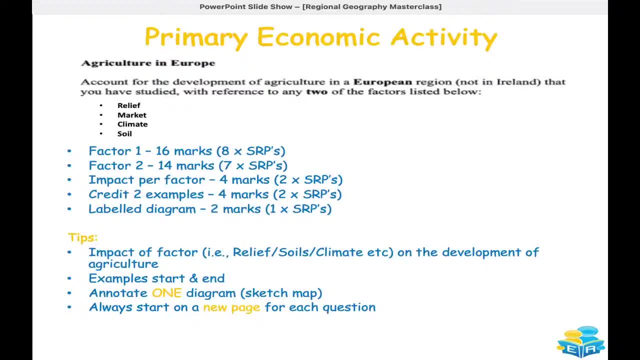 agriculture, um, in the european region, so not in ireland. okay, so don't make that mistake. where you talk about ireland, say it's very clear, not in ireland that you've studied, but reference to two of the of the factors in the below. okay, so you've got relief, market, climate, soil. how is it? 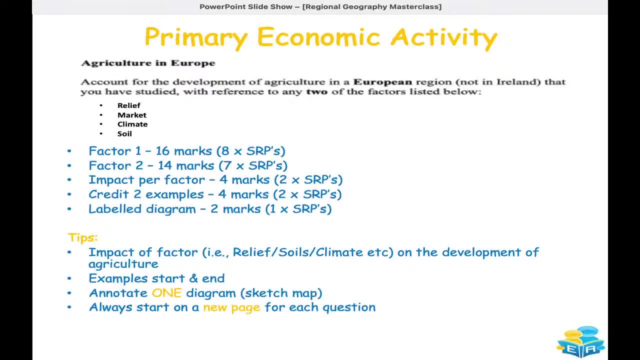 broken up. well, you need to pick two factors. so factor one: it's going to be worth eight srps. um, you need to give the impact of the factor okay and there's an srp going for for two impacts of each factor. there's two srps going for two examples. so four marks, and if you label the 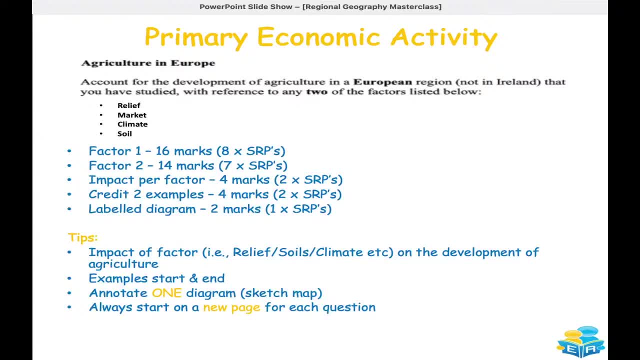 diagram. it's worth one srp or two marks. okay. so impact of factor: it's really important that if you're saying relief for soils or the climate, how does that impact on agriculture? okay, so how does relief impact on the development of agriculture? how does that impact on the development of agriculture? 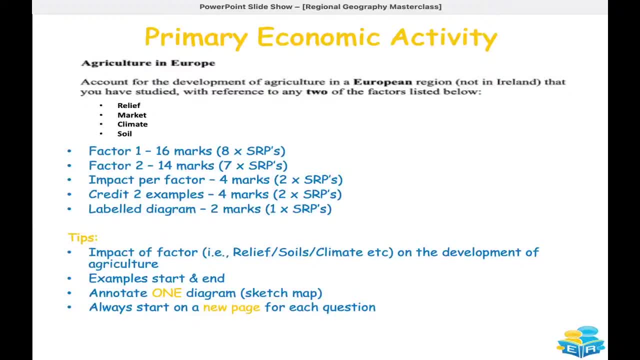 how does soils impact on development of agriculture? how does climate or market, whatever it might be- how does that impact on the development of agriculture in the paris basin or the european region that you're looking at? again, example to the start and end. annotate one diagram, okay one. 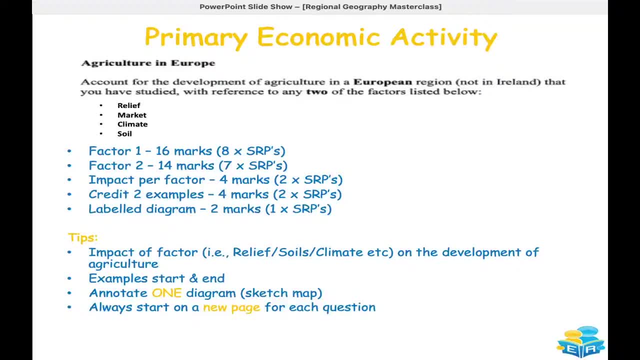 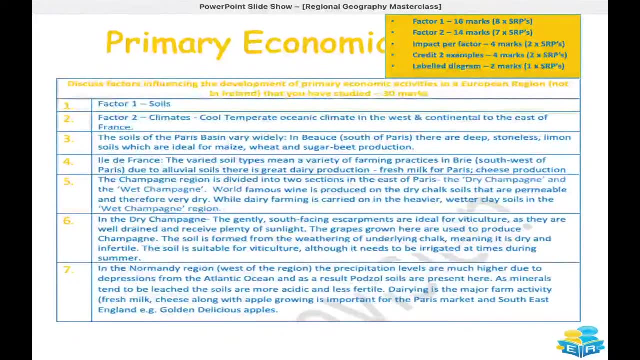 sketch and always start on your page, okay, so again, i've broken it up here. i've got sample answer where i talk you through it here. okay, so the two factors that i looked at was soils and climate. um, and then i'm gonna give like the impact of the factor on the development of agriculture. 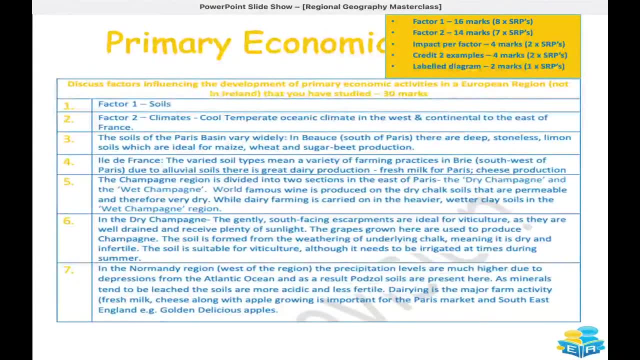 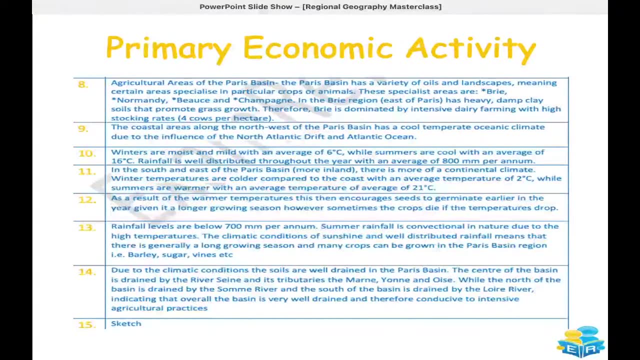 and i'm gonna give like two examples, i'm gonna have a sketch, okay, and we've got then our answers. you'll see again that they're very, very detailed, okay. so, and i've got my full stops. in short, concise, uh points um given like really detailed, okay. so, for example, here rainfall levels are below. 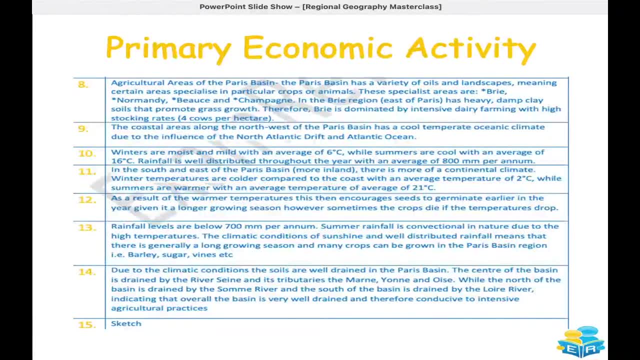 700 millimeters per annum, full stop. okay, because i might that might get an srp and it might not, but it might get it when i have the next one. okay, but if you just run it into it, it will definitely only be one srp then okay. so i'm going to give like two examples. and i'm going to give like two examples. 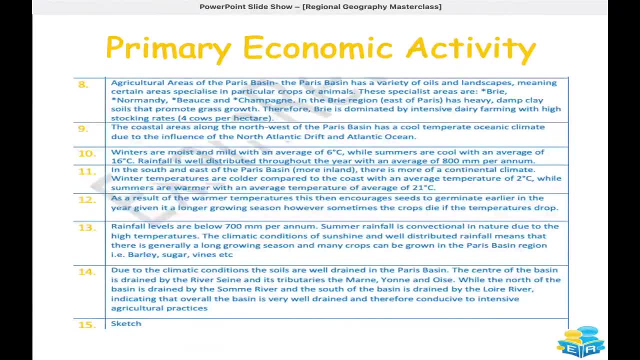 okay, so important. really concise, short sentences, uh, with lots of full stops, is really um, it's really important, okay. so, for example, like with this one here, winters are moist and mild- the average of six degrees celsius- while summers are cool with the average temperature of 16 degrees celsius. full. 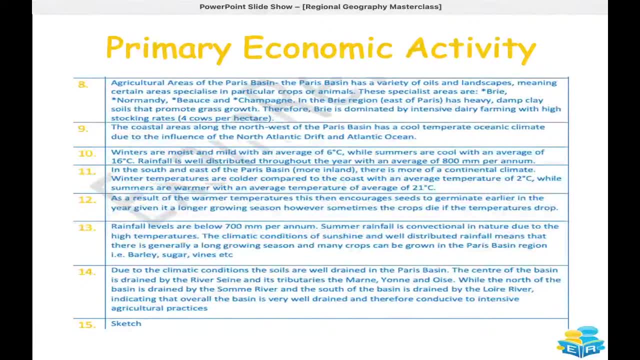 stop. okay, don't have to run this in because might get an srp for that. depending on um the examiner, and rainfall is well distributed throughout the year, with the average um of 800 millimeters per annum. okay, but if i ran that just into it, if i didn't have full stop and i just made 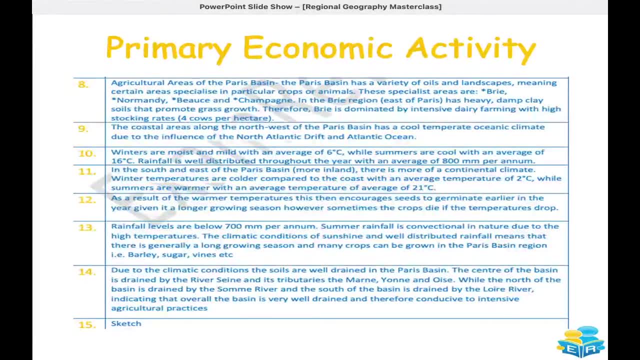 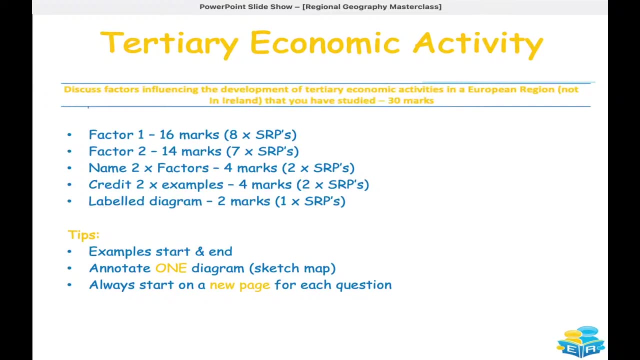 that all that would be one srp, but now i can potentially get two srps even with just that, because it's short, concise, really detailed, like really detail, tell me, and exactly what i need to know. okay, the next one for paris- uh, paris basin i'll be looking at- is tertiary. 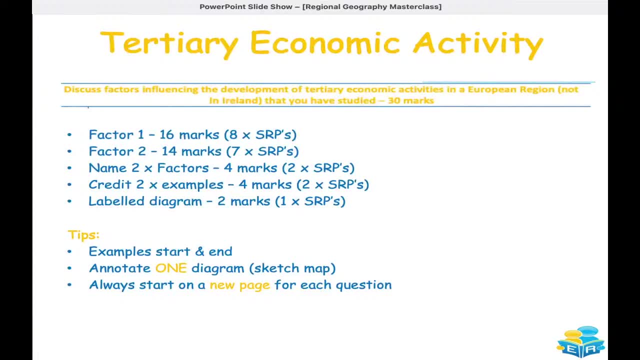 economic activities. okay, so example of a question: discuss factors influencing the development of tertiary economic activities in the european region, not in ireland. that you've studied. okay, again, factors one is going to be asps. factor two, seven: name the two factors. you're getting one srp for each one, so it's four marks. give me two examples. uh, you're getting two srps, four marks. 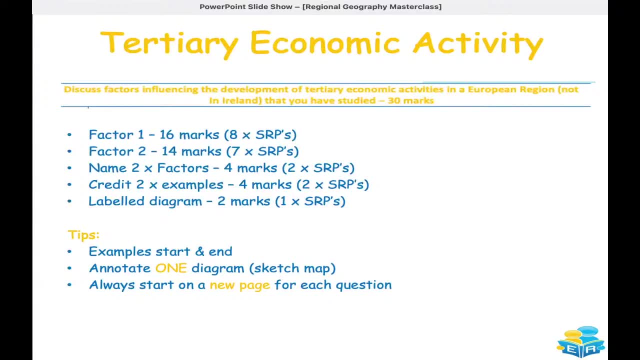 and you're getting again a diagram you draw. you draw a france and drop it into paris basin and put in tertiary economic activities. if it's um tourism, if it's road and rail, um it might be like transport facilities or tertiary economic theories, depending on what you, you've decided to. 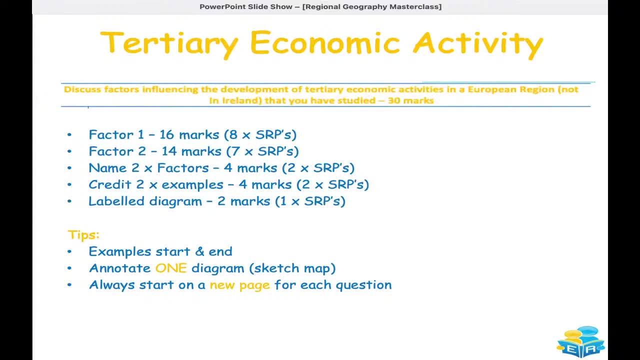 discuss. it's easy to put it in. you know all the information. you've practiced drawing out france and you've got all the different um things that you've been asked for the last 13 years with the diagram that i had to start, so it's very, very easy for you to score um, an easy um, at least one srp for. 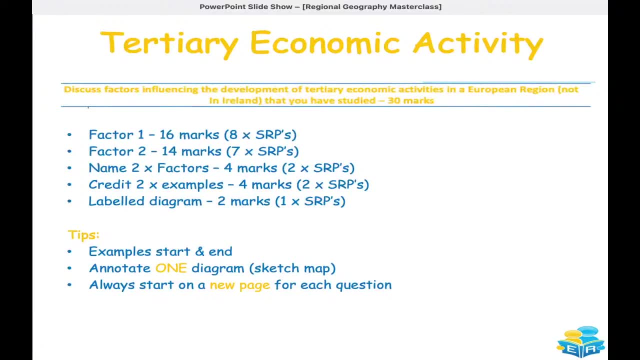 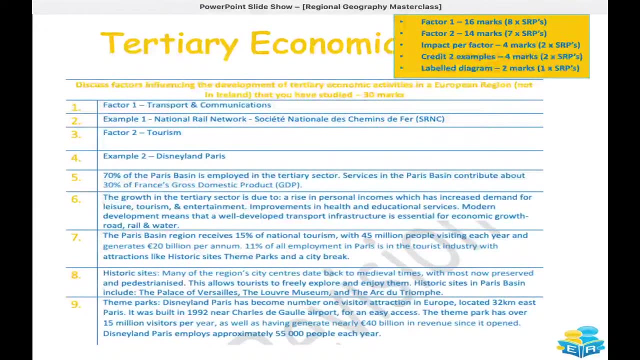 your label diagram example to the starting end. annotate one diagram using the sketch map and always start on a new page. okay, again, we've got the sample answer here. this is going to be and i can give to you. this will be given to you as long as you fill out the. 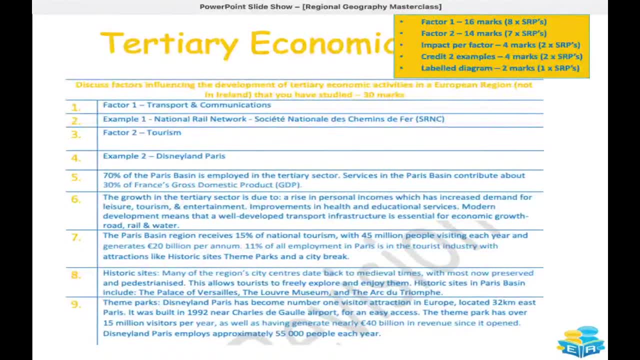 google form. okay, um, you'll be given. um, you'll be able to, you'll be given, like all these slides, okay, so you've got factor one example, factor two: example: i've written, i've wrote like very few words there and i'm getting that's four srps and then with my next page i've got my sketch. 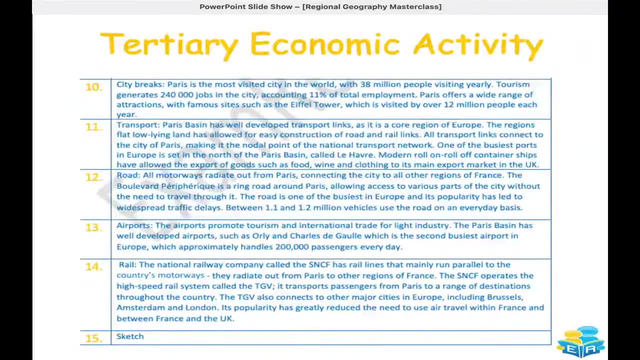 i've got. that's five srps, really easy, and then you can see that i've got lots and lots of detail for the, for my, each of my srps. they're really concise, give me really good like information that are really specific to the area that i'm looking at and to the topic that i've been. 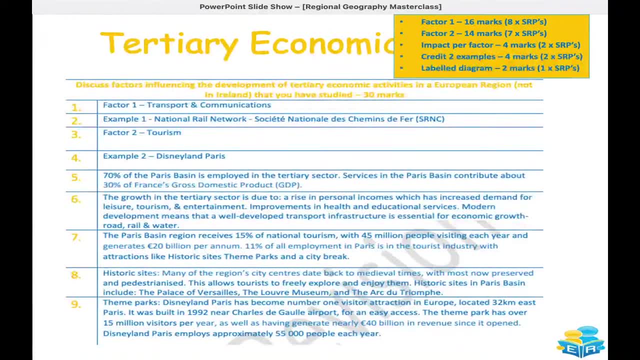 asked, which is tertiary economic activities, and it's going to, i'm going to score 30 out of 30. okay, and with these, with these like um sample answers they are, could they would they have 17, 18, 19 srps in them? just to make sure that you, you're a student, you want to maximize your, your marks. 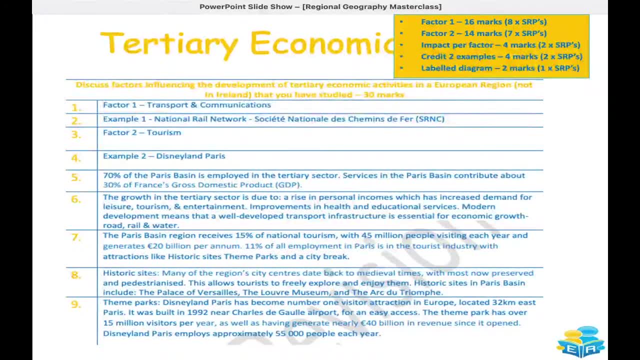 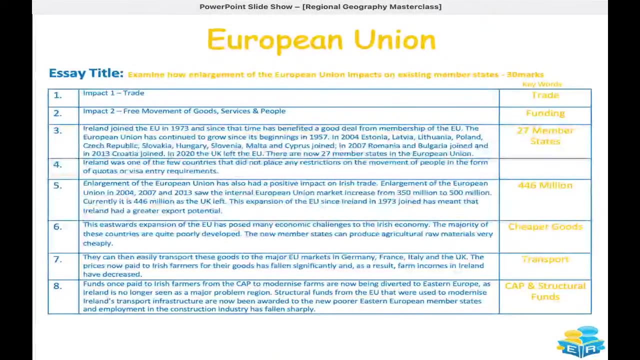 you want to get a h1, you're going to need to have. you should be aiming for about 17 srps to make that. like all, no matter what examiner uh reads, um your script, they're going to give you 30 out of 30, okay. the last one then is the european union. okay, so very, very topical with brexit, um, and. 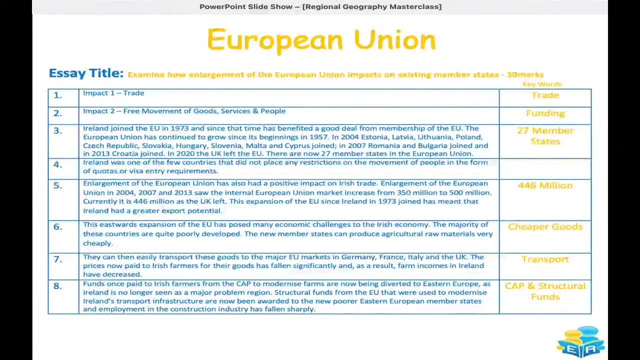 with the uk leaving the eu, um, like this year. so it's going to be something that is is potentially it comes up very frequently in the exam anyway, this european, the european union question, but it's going to be something on on the, i would imagine. uh, so be prepared for this. um, so, with this question, says how enlargement of the 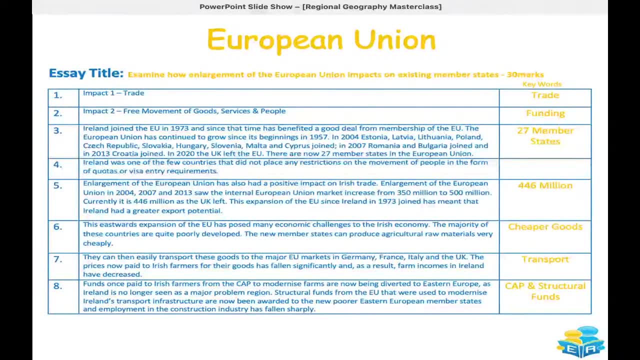 european union impacts on existing members. okay, could be, maybe, how brexit has now impacting on the european uh union. okay, how, how is or how is brexit impacting on, uh, the existing members within the european union? um, so, so be prepared for a question like this, okay, and even with the with 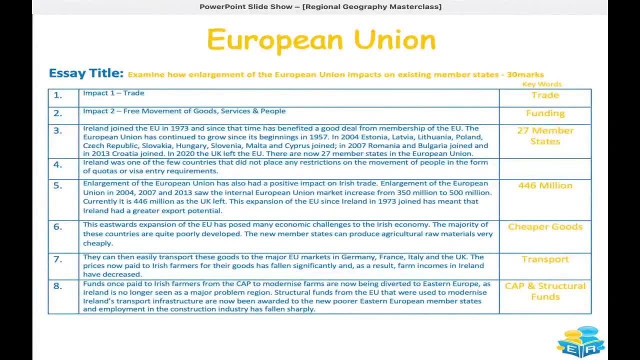 if it, if it changes and it's got like um, that the question is on brexit, like in this question, is similar to like enlargement. this is all still going to work. okay, all like lots of these, like these points and are going to work for that. um, actually, i didn't say try to the this class. 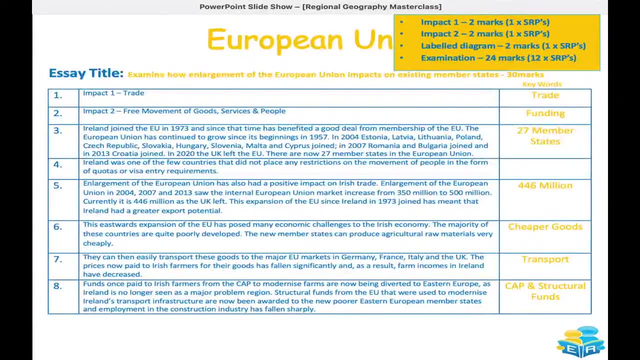 apologies. if you have any questions, please do ask. um, please do ask the questions on ilm, i'll answer them. i'm just going to quickly go in and see, okay, so i'm just saying: if there's any questions here, so please do. if there's any questions, just ask. 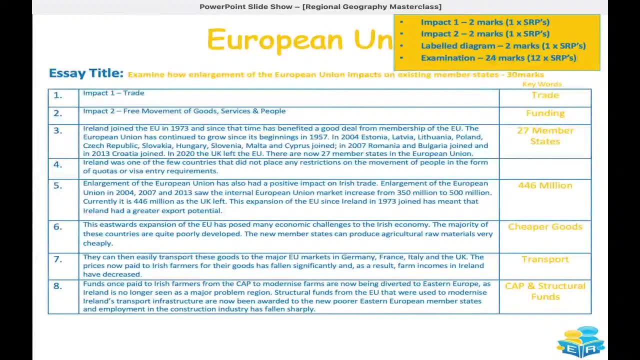 again, it doesn't have to be about regional geography. um, actually did. i'm sorry. i'm just going to the the chat here just to make sure there's no questions. i haven't that you've asked and i didn't see okay. so no, i think we're okay. okay, but if there's any questions about any part, 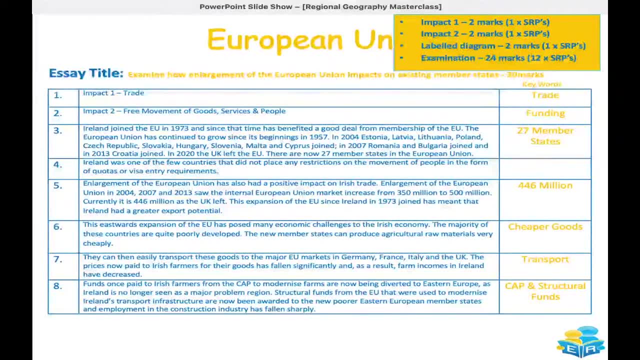 of like geography. please do ask them in the comments section and i'll answer them in the Q&A box and i'll happy to answer and i know you can imagine, uh, this year you'll have a lot of questions because there's lots of changes, lots, and that's why i hope to start with the adjustments. 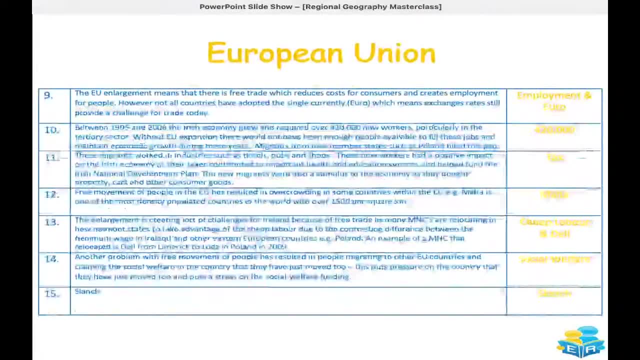 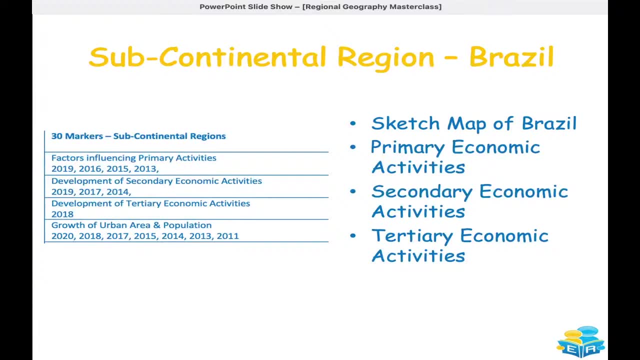 that. that made it really clear to you. and then we're going on to like the subcontinent region. okay, um, so obviously i'm not, i'm just going to whistle. uh, stop to like through this really, really quick. um, and with the the subcontinent region, brazil, make sure you can, you can draw your. 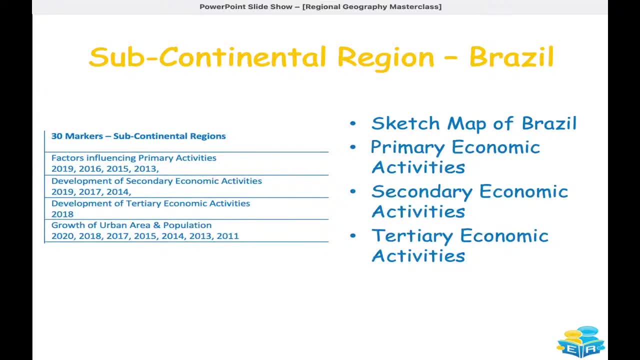 subcontinent region. okay, so draw it like this and then i'm going to go ahead and i'm going to be able to draw the sketch map for for this year, i'll be focusing on primary economic activities, secondary economic activities and tertiary economic activities for the brazil region. okay, 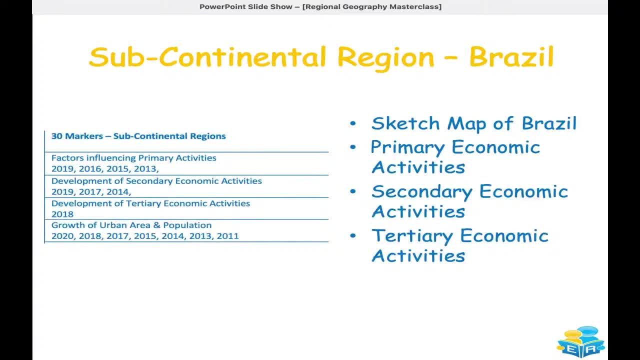 i think they're going to be very, very important. um, based on how what's what's come up in previous years and the growth of the urban area and population distribution come up in 2020, so now it is a really popular question. so it could potentially, but i think it's going to be- 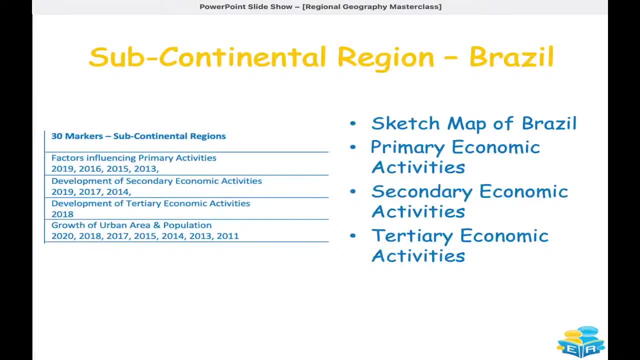 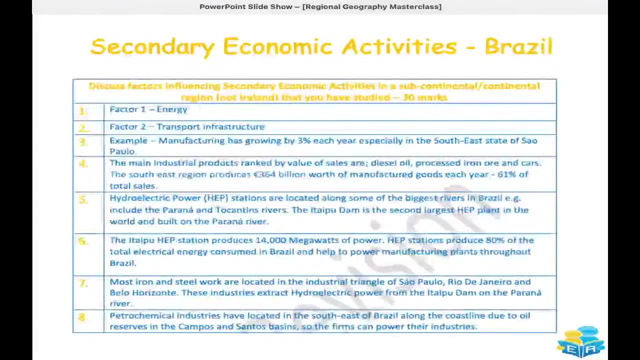 uh, like these questions- the primary, second, tertiary- that will appear on the 2021 paper. okay, again, we've got all the got all the sample answers in here. okay, i'm just gonna whiz through this because i know i'm kind of running out of time. 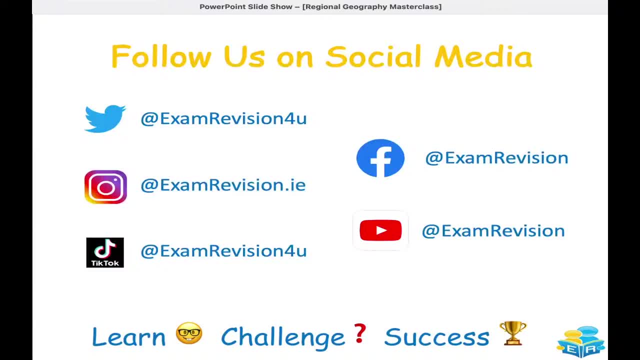 okay, um, if anyone has, uh, isn't following us on social media, please, um, can i ask that you follow us on social media? so we've got um twitter and so if you're a teacher or if you're a student, that has twitter, and if you're a student, teacher's instagram or tiktok. we just set up tiktok recently. 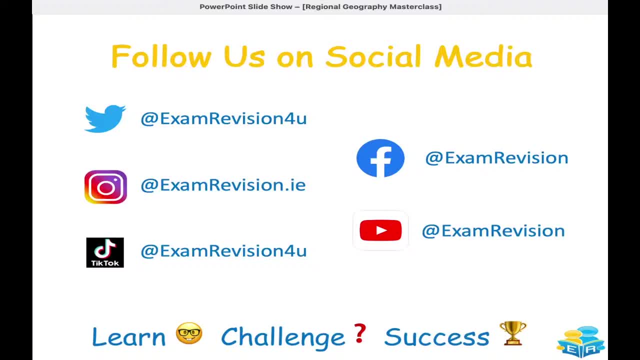 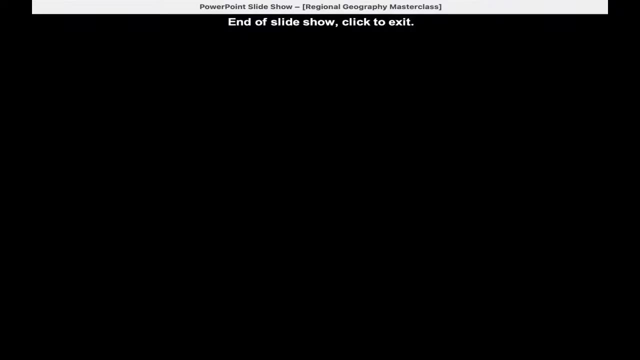 okay. so we're trying to build their following on that and if you haven't subscribed to our youtube channel, i think we're very close to 12 000 subscribers. that'd be brilliant to get to that milestone and be really grateful, and we're just trying to help as many people as possible and with like um, with the like, with um, with with. 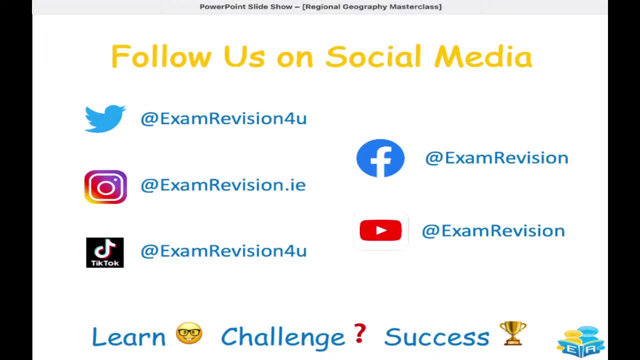 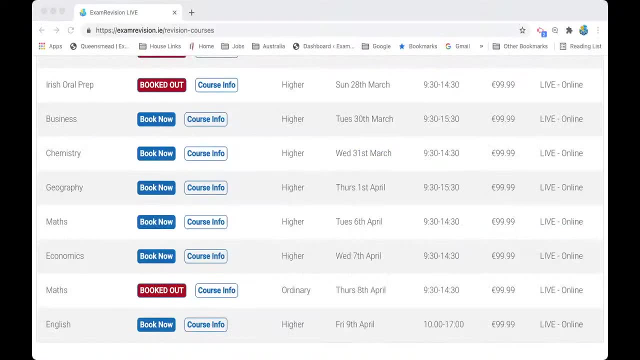 their study. uh, we're trying to make like learning like much easier and cater for all different types of learners, because we notice it's, it's, it's. it's quite difficult to to um, like, like, like, to be able to learn like like we're not. we don't all learn the same way from like from from a book and it's. 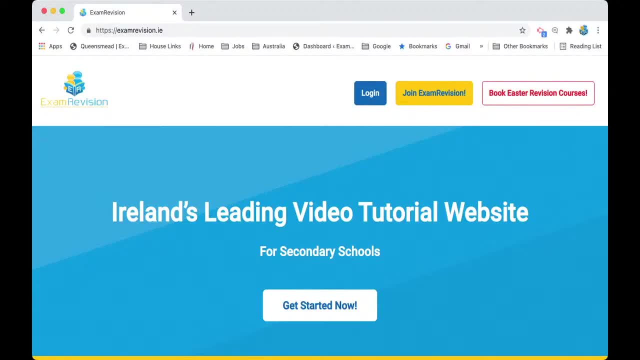 great to be, uh, if you're a visual learner or if you're an audio tutorial learner, that you've got the the tools and you've got to watch videos and use notes and like that's what we try to provide here at exam vision. uh, just before i finish up, then again, just if you want to attend, uh, our easter. 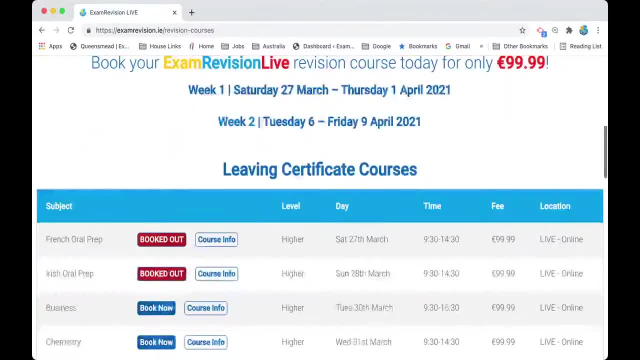 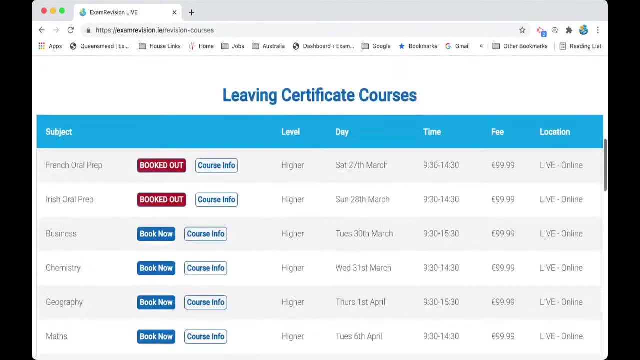 vision courses. they are there's. there's like still some available okay, uh. so business, chemistry, geography, maths, economics and higher level english, uh are still available and but they do book out and because we have them capped and once we have them capped we're going to be able to do a few. 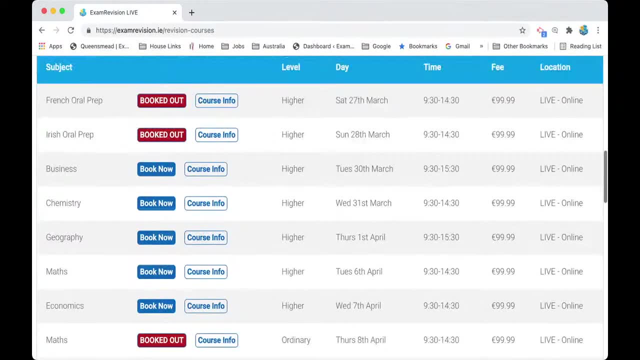 other courses as well. so if you're interested in that, you can just check out the exams. we've got a link in the description below and um, we'll get to that link in the description of the video and we'll see you guys kept because we wanted to be really personalized and tailored to to um the students that attend. 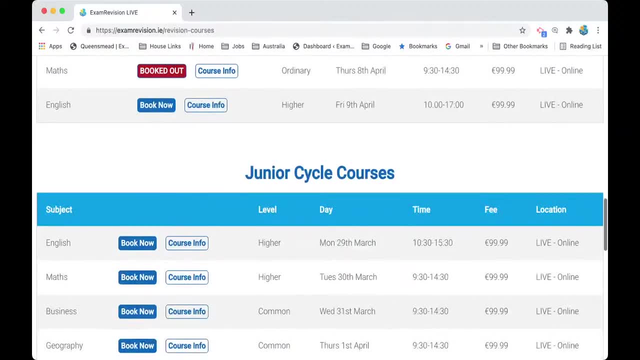 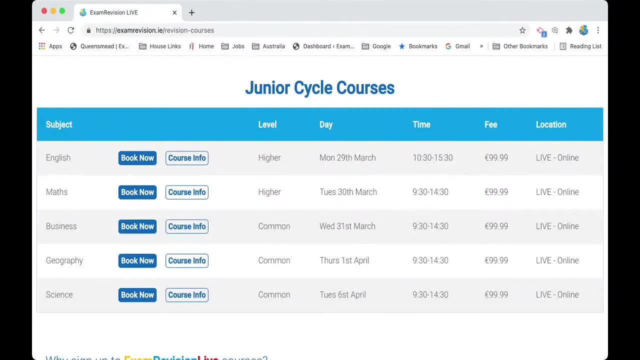 the courses and we also have junior cycle as well. so if you have younger siblings that are interested and they're really much, very much like booster classes and filling it like gaps in knowledge that maybe students might might have, might have because of the school closures, um, and that's what.